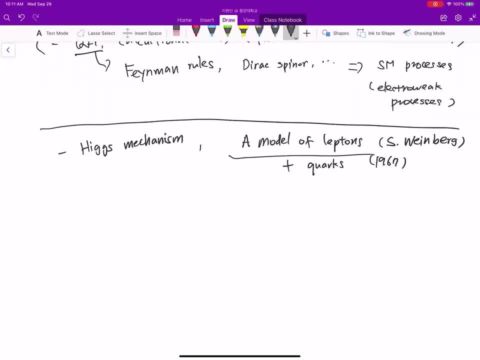 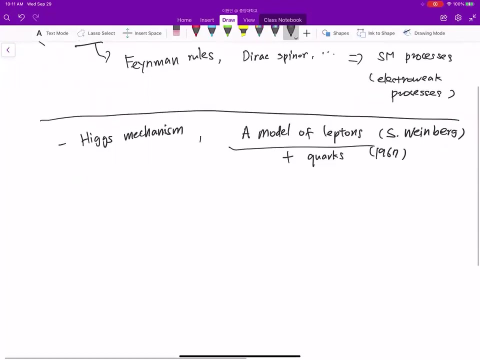 for which the Steven Weinberg awarded Nobel Prize, I mean include, together with the Glashow Weinberg and Salam At that time. there are several candidates for the standard model, But experimentally the Glashow-Weinberg-Salam model has been proven. 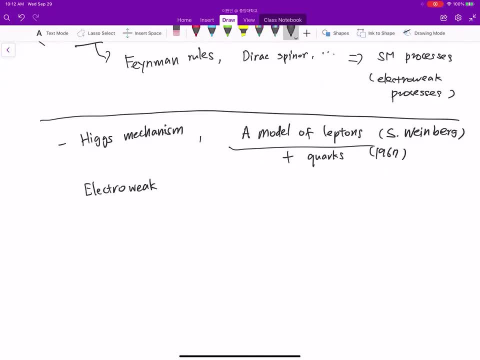 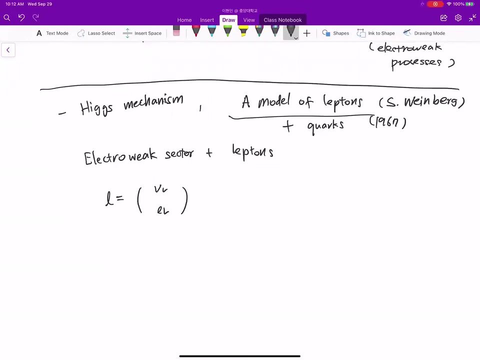 was proven to be true. So electroweak sector plus leptons. So leptons we are, but there are three generations of leptons. But the family, the flavor structure will be discussed later. Just to, I think. 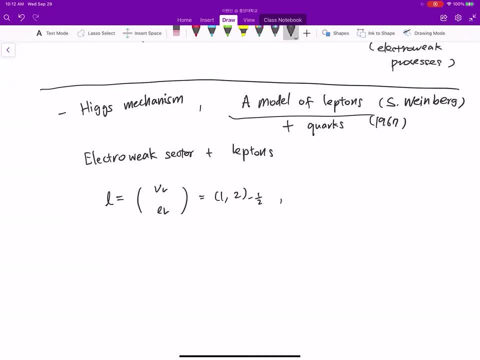 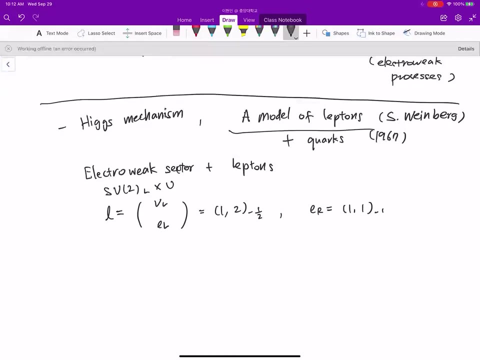 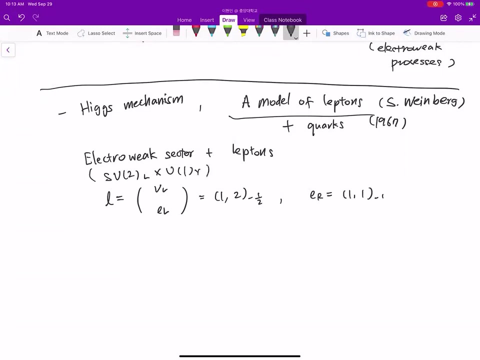 let's take one, only one generation. So this quantum numbers under the gauge symmetry. So electroweak sector gauge symmetry is the is the structure. So, as you know, the one is the SUS3 color. color 2 stands for SU2,. 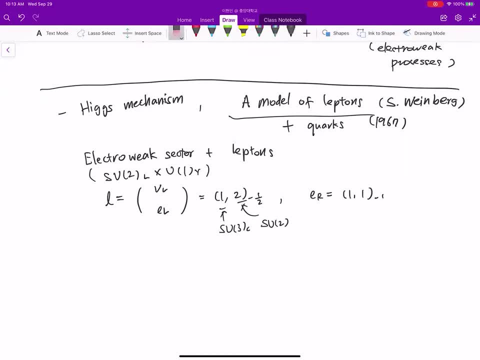 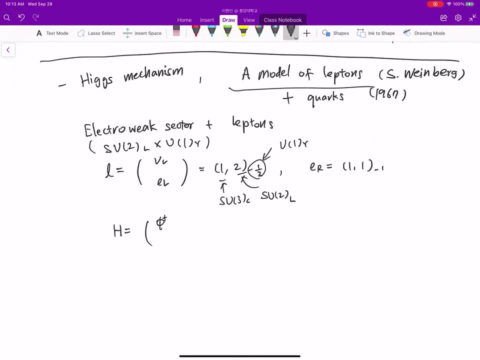 left-handed And this subscript is stands for hypercharge, And we have Higgs-W- Higgs also in the written in. this is the replaced solution, And so this is. I've been doing circles: crisscross matrix type. 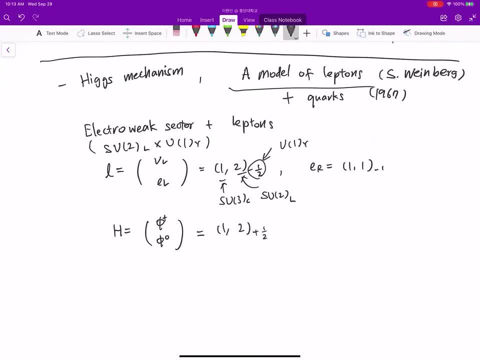 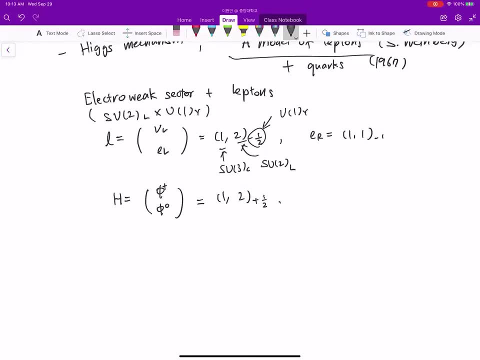 because this is, but the. that's what we called by, by the Higgs-W, Because Higgs-W is an object, with this counter, like right under your point circle of this clear And two complex scholars with the gauge. 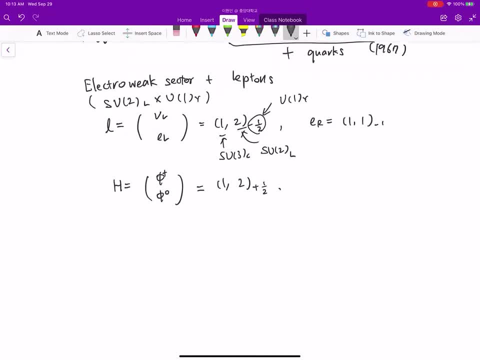 the quantum numbers, like this one, And for for for leptons, there is no need for conjugate of complex, conjugate of the complex Higgs doublet in this form. but then this, it's not introducing additional scalar, but the same Higgs doublet. you can take the. 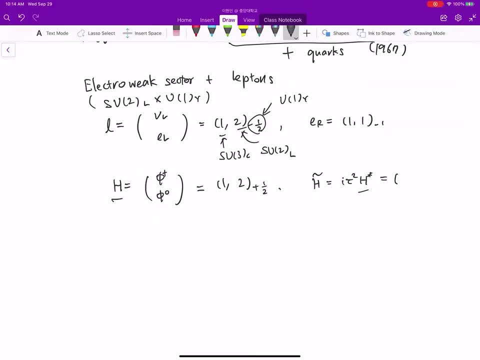 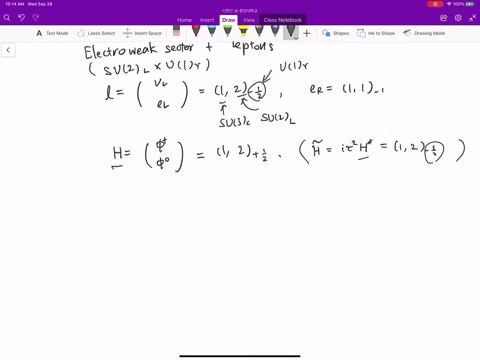 complex conjugate and the tau two is the Pauli matrix. so in this case the quantum number gauge, quantum number. so SU is the still doublet, but the hypercharge is the minus one half instead of plus one half. so this is important for masses, for for quarks. 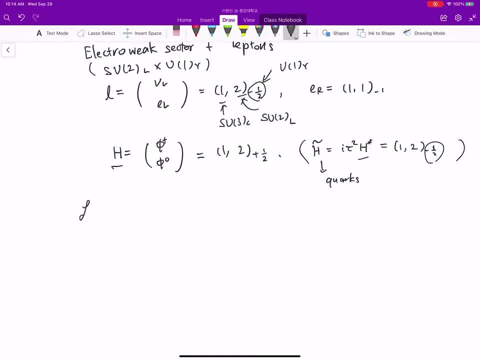 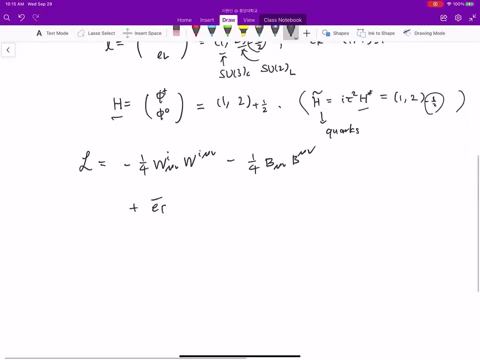 for leptons you don't need, so then the Lagrangian you can write down. so SU to gauge sector, first the field strength tensor and the kinetic term. the kinetic term for fermions, in this case we are using the four component location, which is 38 degrees for 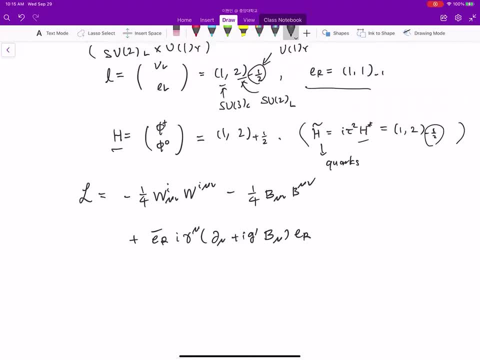 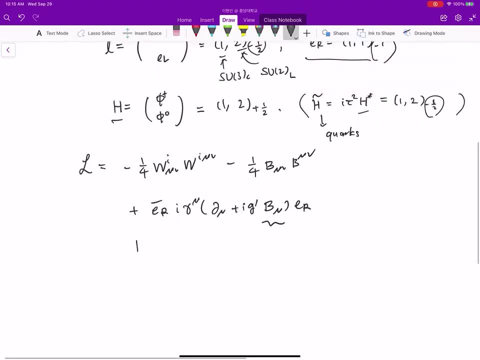 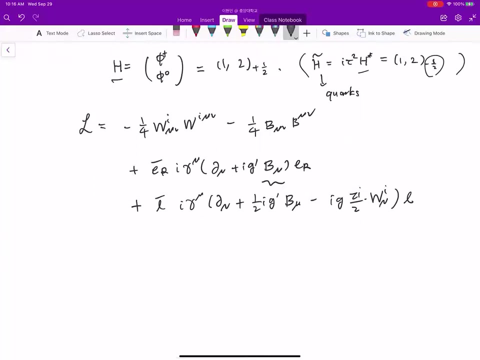 plus the, so the remaining surface zones to hypercharge and also couples to uh elect, uh electroweak gauge burdens response. so, uh, here we omitted identity two by two identity matrix here hypercharge and also gradient, the derivative. so there's the one two by two matrix. it is omitted implicitly there. 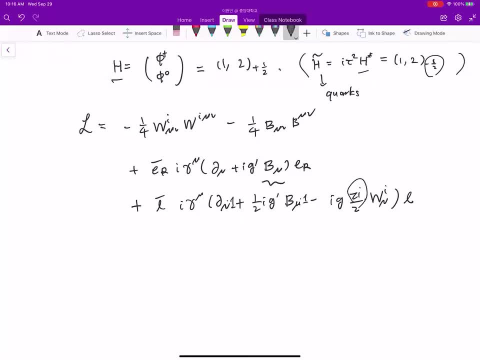 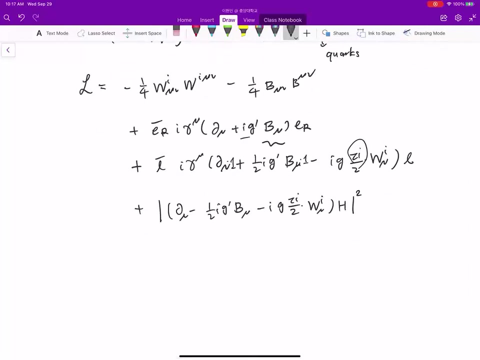 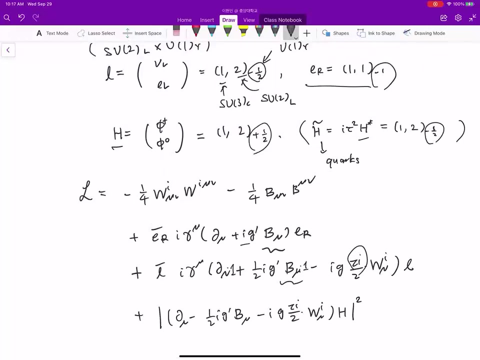 and there's also. we have a power matrix right and the higgs kinetic term also there's one. so higgs kinetic term, then you have. you see the, the convention for the uh hypercharge, uh coupling. you see the uh it's upper design for fixed opening one half. because of that you have this one for su2. they. 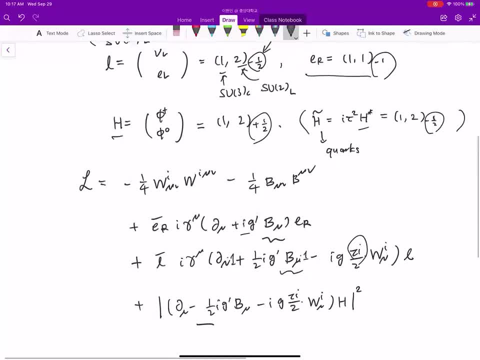 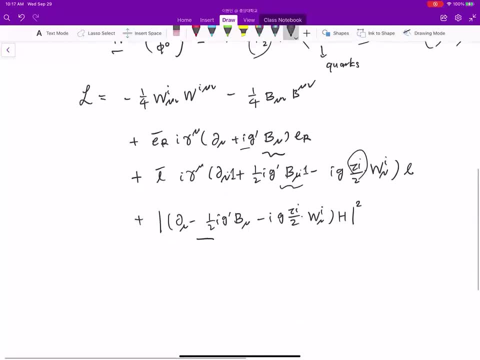 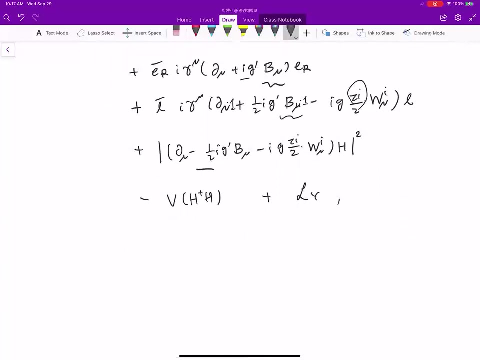 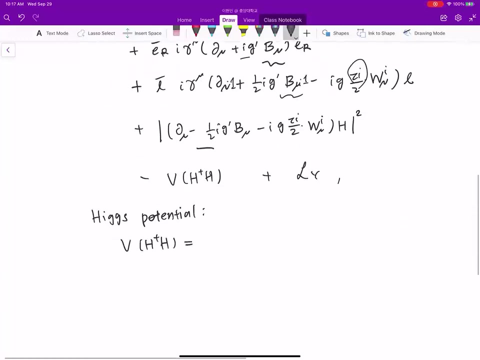 are all non-hickory, the same representation. i mean the lepton doublet and xw. and then we also need to add the higgs potential and the yugawa interaction for lepton. so his potential. so we h, it's h, h. so this, the potential, x potential, is function of h, h. 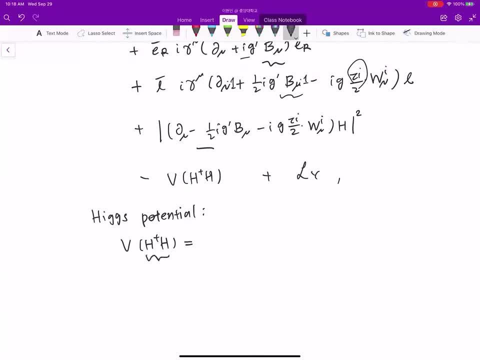 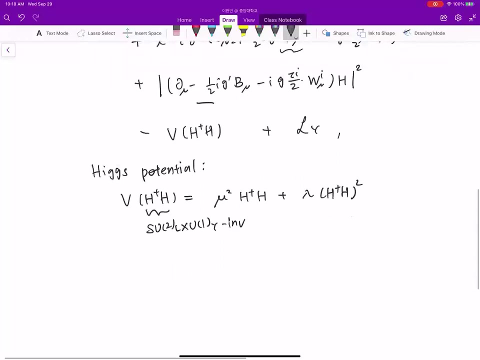 because h- h is the invariant su2, because su2 cross u1- invariant combination. so the lowest order in this combination will be the lowest two will be the core, h, h and then h- h square. so the mu square is mass parameter: x mass. it's not very different from physical x mass, but this is the mass parameter and this is quartic. 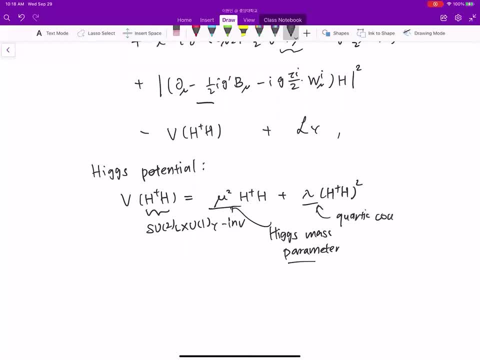 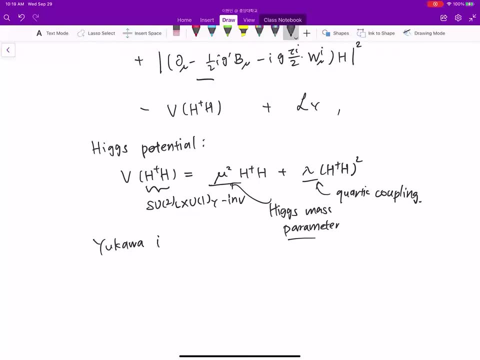 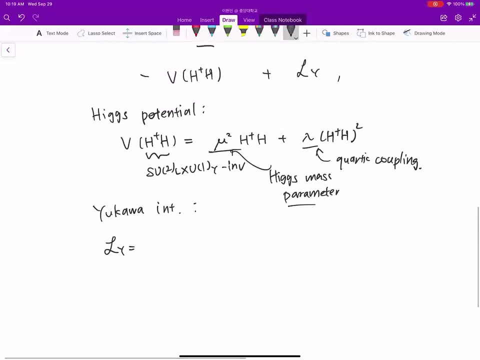 coupling, you know, so then you'll have that. that's very specific, alright, so this is, you know, all four shape, then these two yourself. so one of them is in common, the one, small one, is a bigger part, the other one is in hyperpoint. so this is your expression of the two. 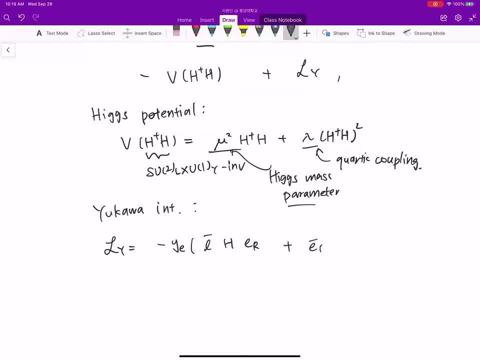 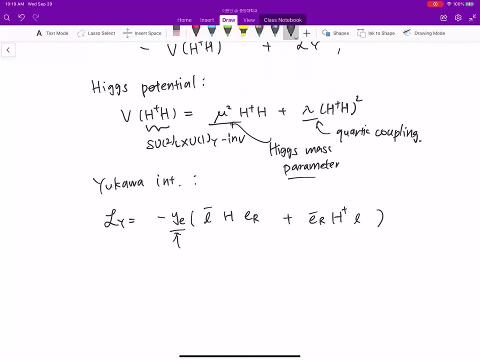 because of that iced shape. go to the equation and use the situation, do a h h round. So this is the only choice you can take. Of course, in general, this Y is the Yugawa coupling. This could have complex phase, but it is known that you need at least three generations to 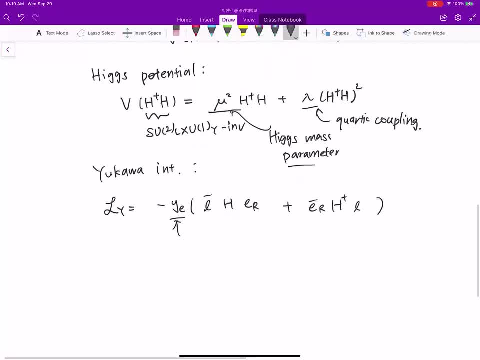 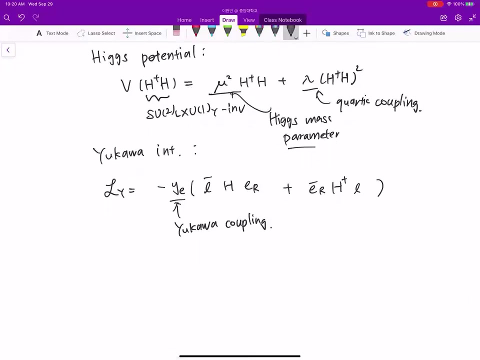 get non-zero CP phase So you can ignore potential complex phase. So this is Yugawa coupling. So there is a general discussion on the independent, on the physical CP phases, CP violation basis. So in the case of quarks also there are some non-zero CP phase in the leptin sector. 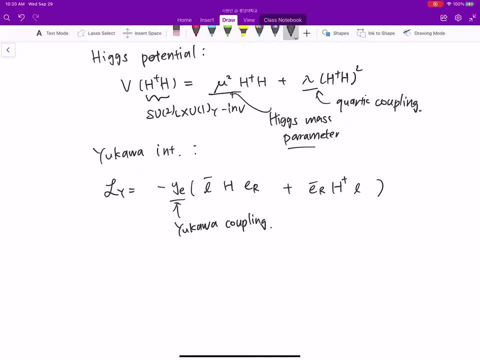 But this lecture we are going to discuss mostly on the quark sector for CP violation basis. So here then you can identify the first. you can check the hypercharge right: hypercharge, This ER is. the hypercharge is the same as electromagnetic charge, so minus one, which. 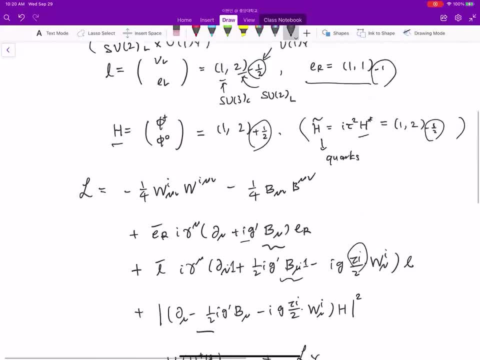 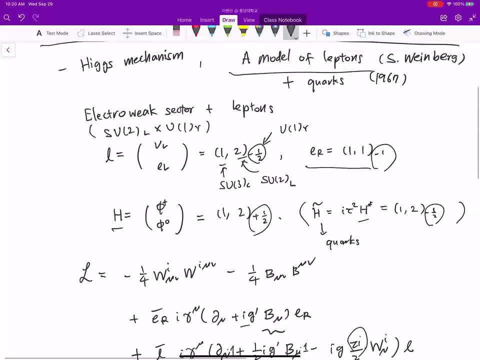 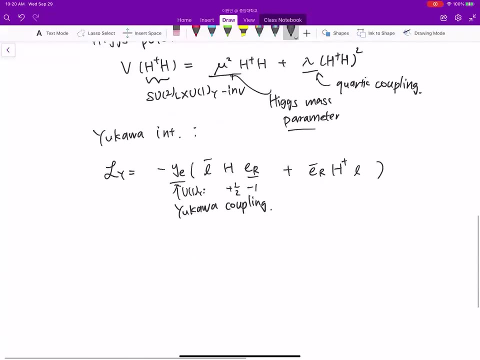 is minus one, So H. you can go back plus one half, right. so plus one half. And then leptin doublet, minus one half, So the conjugate. so then plus this bar, let's say plus one half. 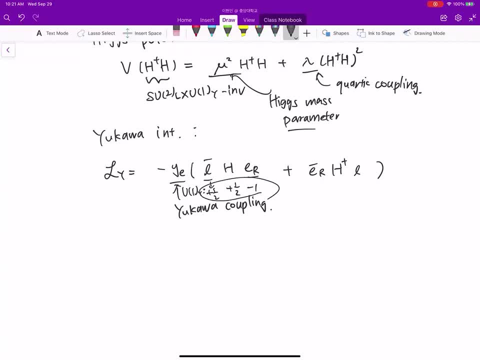 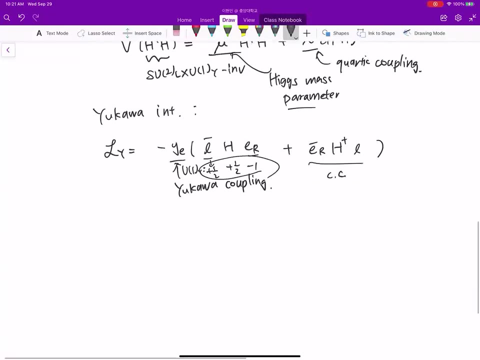 So if you sum them up you get zero. So hypercharge, invariant, and just the second term is the conjugate, So complex conjugate, this one is conjugate And for this SU hypercharge, you can check And SU. 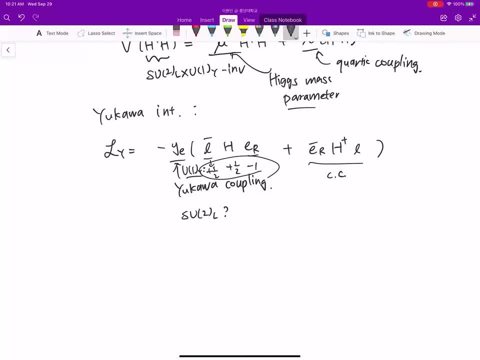 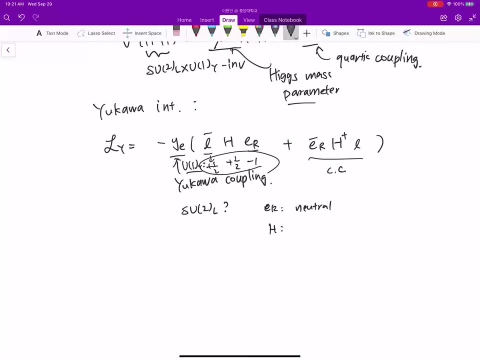 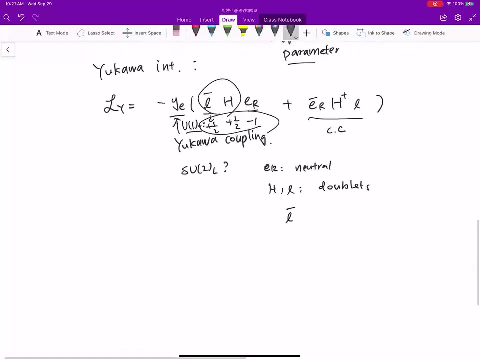 INDEX variance you can also check. And so ER is neutral. Your lepton singlet does not change under the SU. So but you know, the H, H and L, they are leptons, they are doublet. So since we take the conjugate here, so let L H. 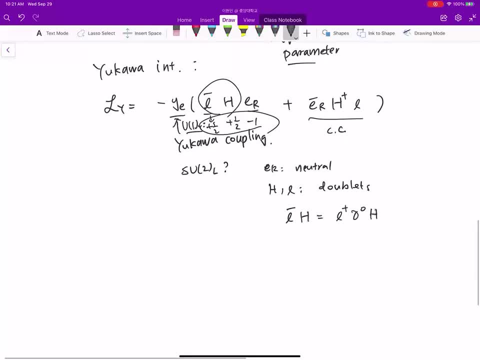 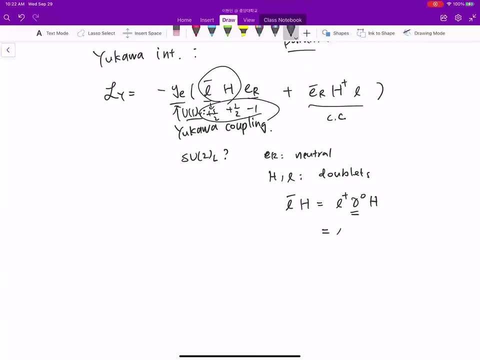 means L theta, gamma zero, H, but this gamma zero acts on the Dirac spinor indexes And then this does color right. So just you can interchange. So this can be a combination: L theta, L SU, L invariant, So L theta, so 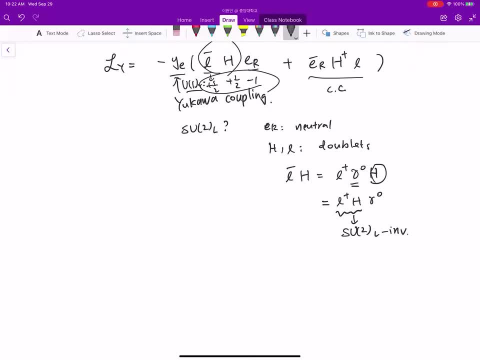 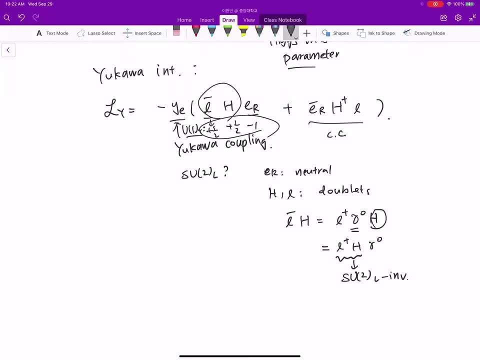 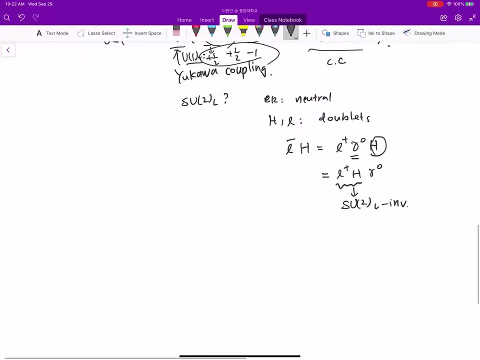 just from the transformation property. So we are going to discuss more on the gauge transformations, But you can convince yourself that this is the SU invariant interaction Between Higgs and leptons. This is very simple. So, and then the full gauge transformation is also. let me write down here more. 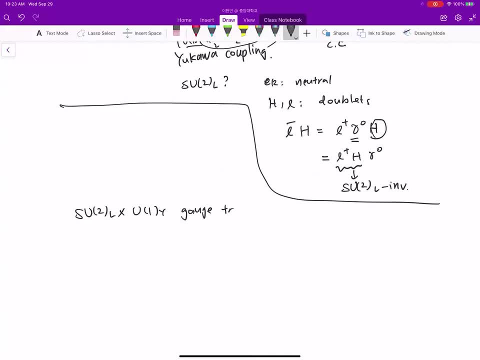 explicitly, Because we are going to choose certain gauge condition for the later discussion. So we are, so singlet is due to singlet, but the ER transforms under the hypercharge. So set Y is a gauge. transformation parameter depends on spacetime, So which is local. 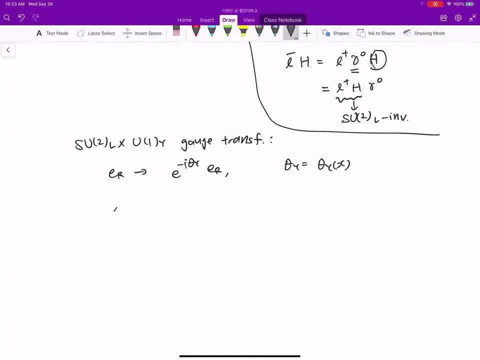 transformation and, in the case of lepton, doublet with the same gauge transformation parameter. but we need to divide by two because the transform transformation depends on charge assignment, so and the su2, su2 transformation, uh require introducing additional transformation parameter. so here there are three transformation parameter. 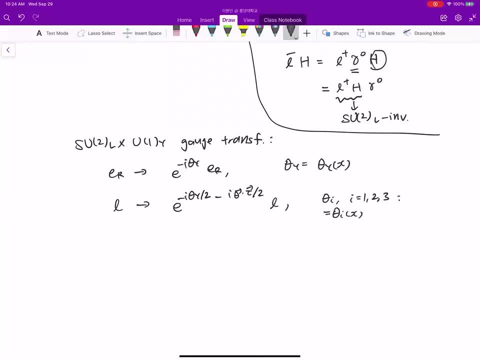 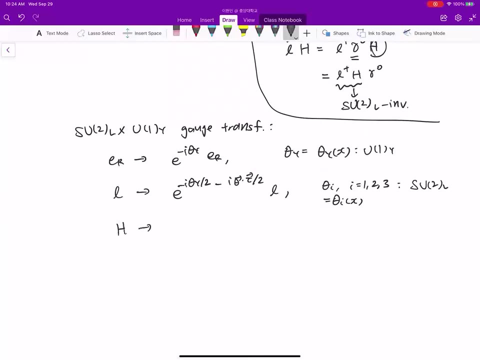 so also this transformation parameter is a function of spacetime. so this is su2 transformation. this is hypercharged and higgs also transform, but the charge is opposite to the one for lepton doublet and su2 transform. it transformed in the same way under the su2 as for the lepton doublet. 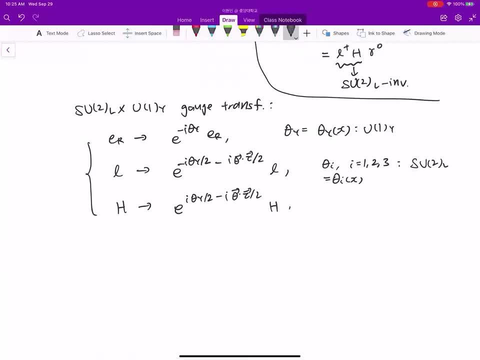 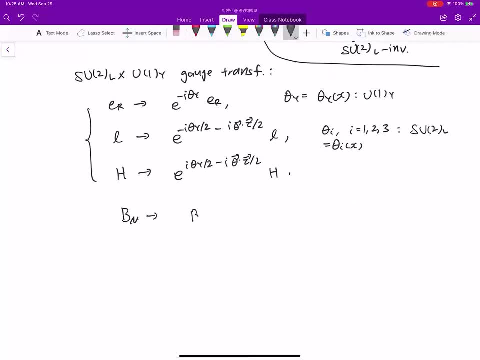 and this is the kind of a metal metal section and the gauge field must transform at the same time by the gradient of the transformation parameter and here, so as compared to the u1 electromagnetism qed, so g prime supposed to be e in the case of qed, but we have a gauge coupling associated with 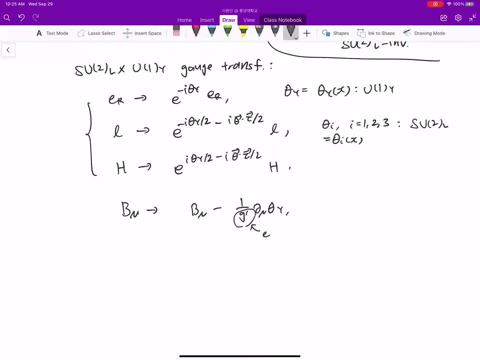 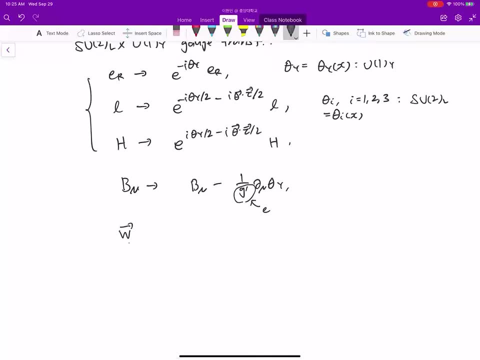 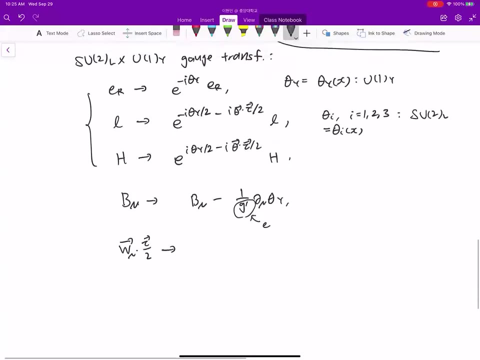 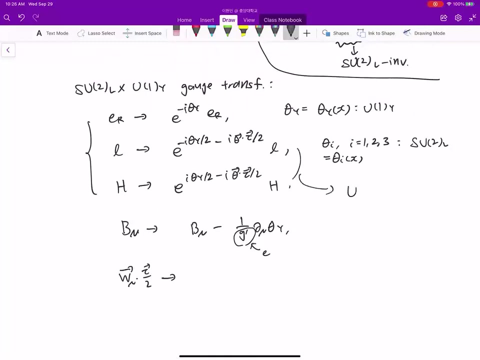 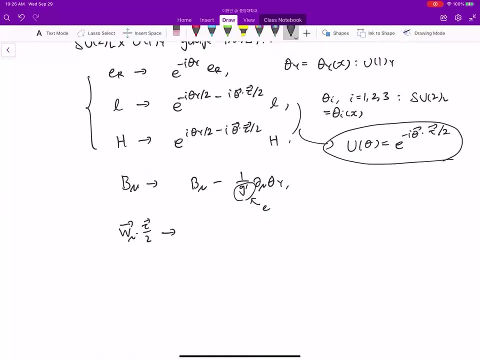 hypercharge, so g prime instead of electromagnetic charge, and also su2 transformation. so here just let me call from this su2 transformation, let me call u of zeta, i mean the exponential su2 part, let me call the su part, u of zeta. then, in terms of u of zeta, transformation of the su2 gauge field, written in this way: 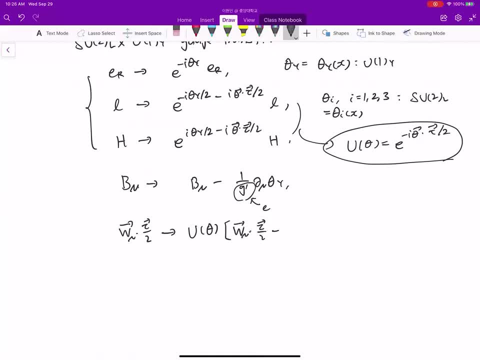 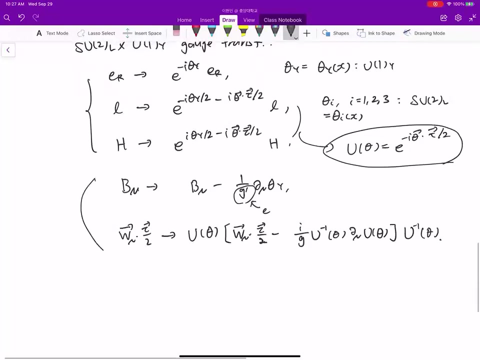 so We have discussed for general non-Arvillian gauge symmetry, but here we specify the non-Arvillian gauge symmetry to SO. So it's just a simple application, right? So this gauge field, then you can show that the previously written Lagrangian is the gauge. 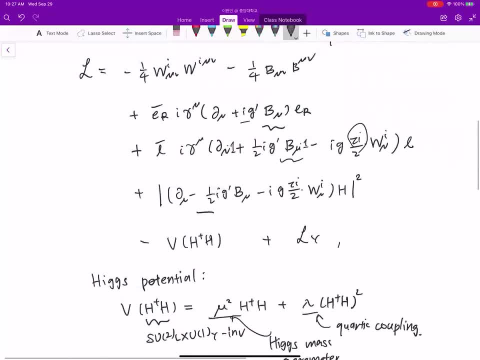 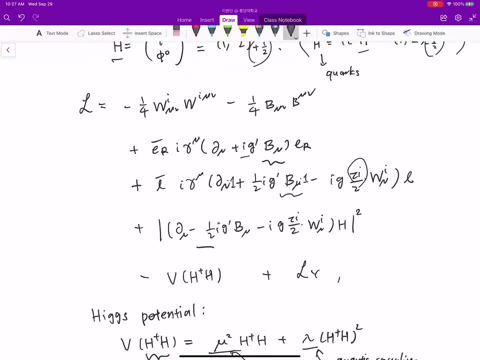 invariant. This Lagrangian is the gauge invariant, as you can see. I don't know if you know, maybe, Arvillian, This is the edge field. So this is the edge field. So this is the edge field. This is the curve for the standard model Lagrangian, as you know, right. 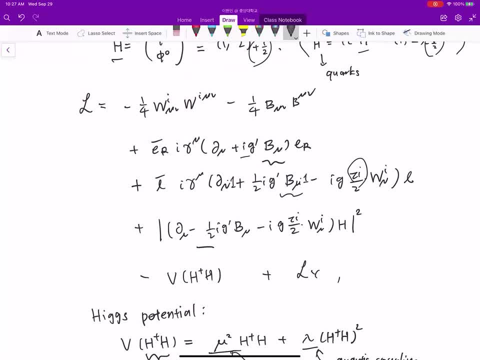 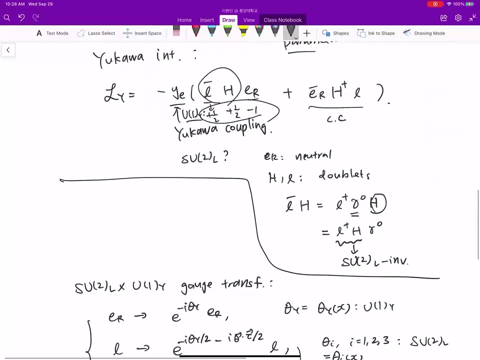 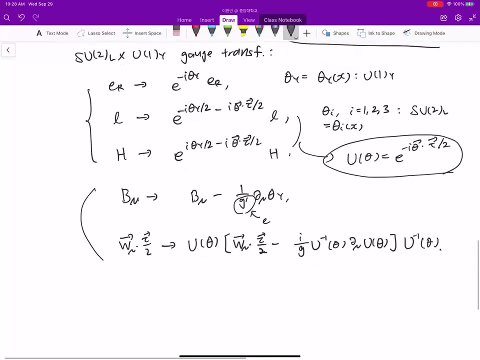 This is the simplification, and I don't know what is missing, but just the collectively written for all fermions except for the same Lagrangian. Of course this one is not complete because there is no gauge-fixing Lagrangian, So we need to introduce gauge-fixing parameter. then the Lagrangian is longer. 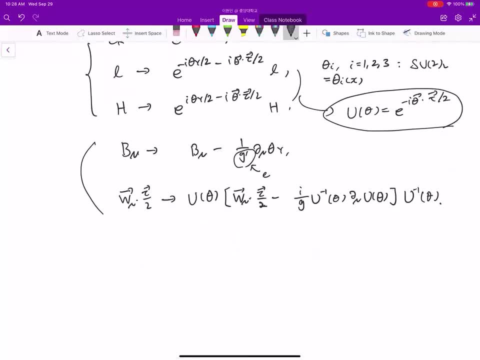 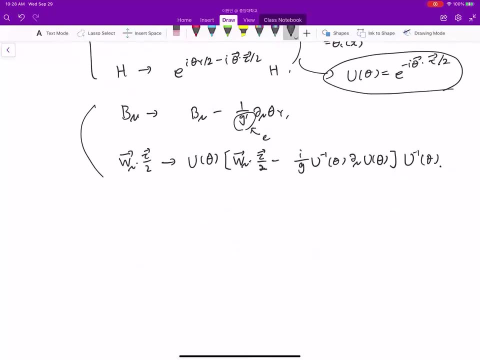 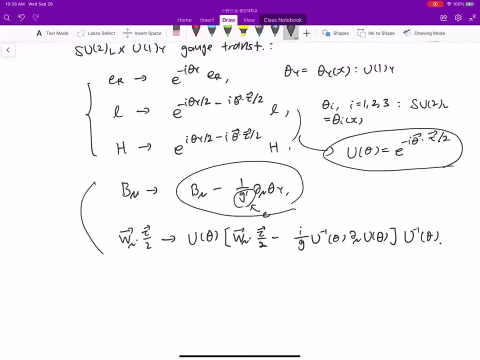 So now we are going to discuss electroweak symmetry breaking and the unitary gauge. Unitary gauge is in. unitary gauge. you can choose any gauge because you have a degree of freedom to transform, So so-called Higgs mechanism. 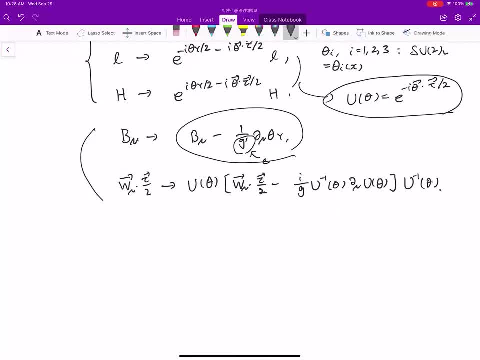 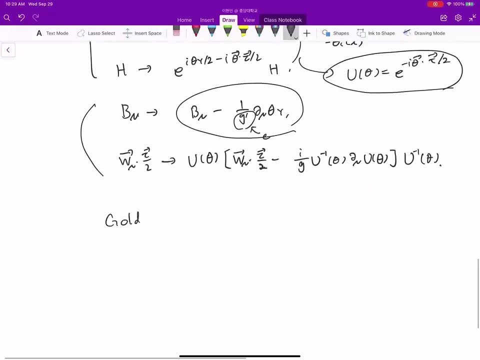 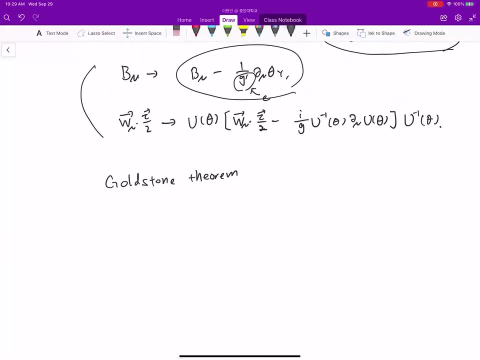 So I didn't- actually I didn't have time to discuss Goldstone theorem. So in the case of, I mean when for the global symmetry, the Goldstone theorem tells you that there are a number of massless global symmetry, when global symmetry in the case, 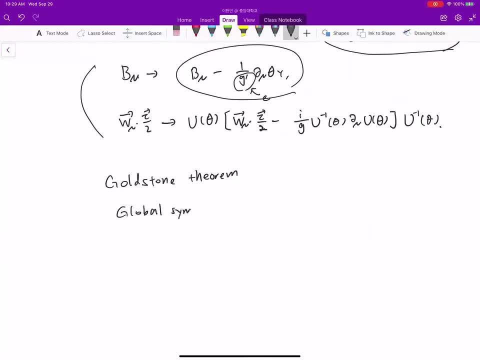 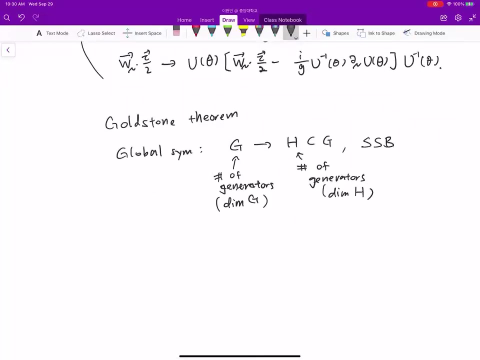 of global symmetry. Big symmetry is broken down to a small group and the small group belongs to a bigger group, And then you can count the number of generators in each group, Generators Or dimensions of G, Dimension of H. Then you can break this by spontaneous symmetry breaking. 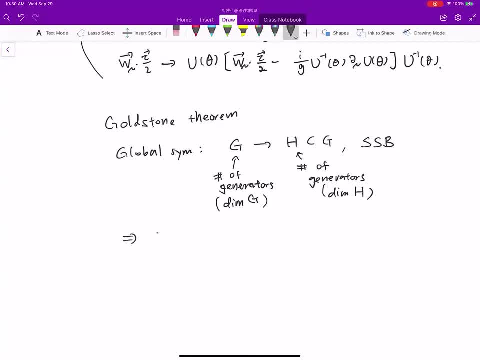 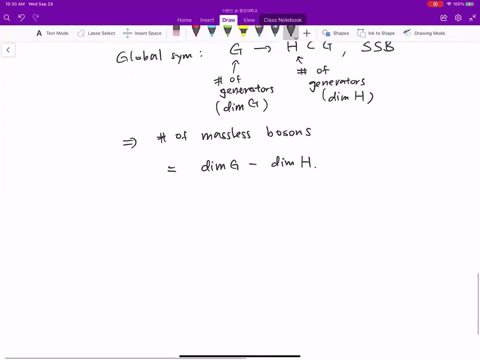 Then the number of massless, same as difference between the number of generators and this we call uh, we uh this or broken generators we call broken generators. so this is the number of this is the number of broken generators. the broken, uh. because we are breaking a big group to small group and some of the generators 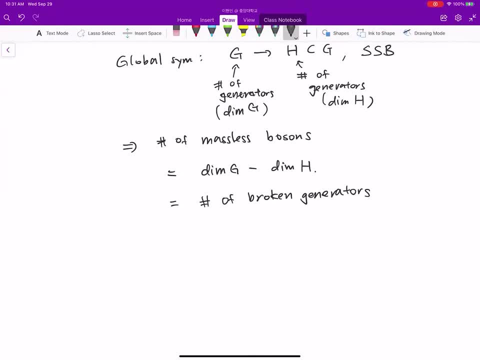 in a bigger group do not belong to each. so some of the, some of them don't belong to each. those are broken, the broken generators, and and we call uh this mess list. uh, world's border is the sorry mess list. borders are called the stone version number. gold stone versions. 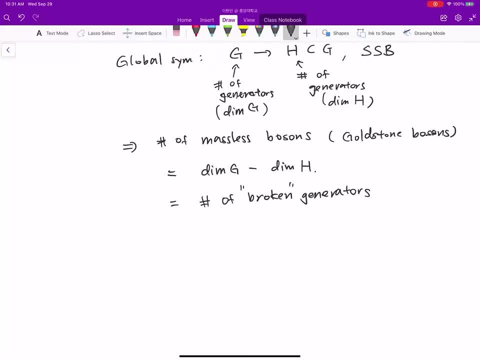 and uh, this number, gold, gold, stone versions are kind of transformation parameterizing. uh, the vacuum manifold, as you know, as you remember the mexican head potential, the vacuum has a degeneracy, you can transform along the valley without caused the energy. so there is the vacuum manifold and the shape of the vacuum manifold, called course, space. 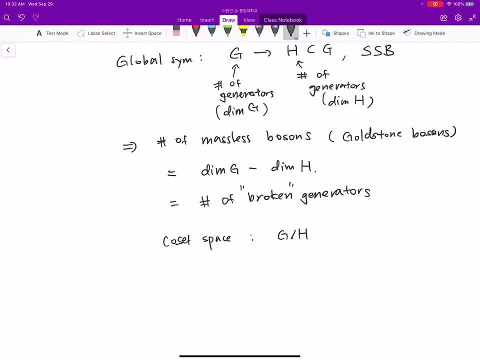 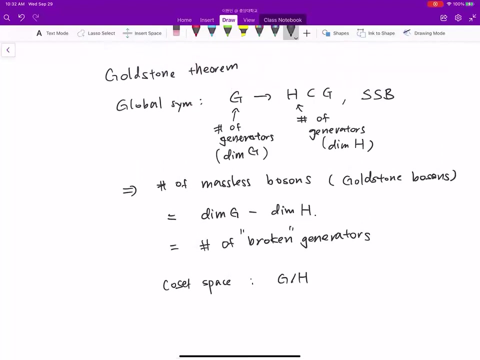 so course of space is uh over h, and the number of parameters to describe this kind of internal space is number of broken generators, so number of mesh exposures. so so this is necessary, of course, this, this goldstone theorem is the, the the vacuum must be wrench invariant. 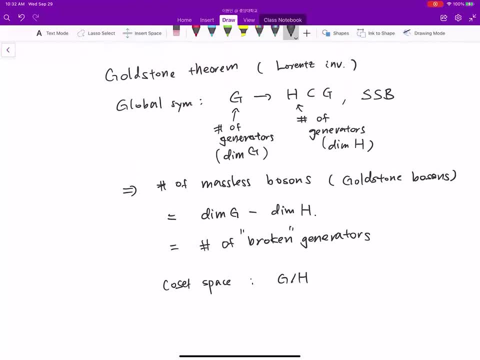 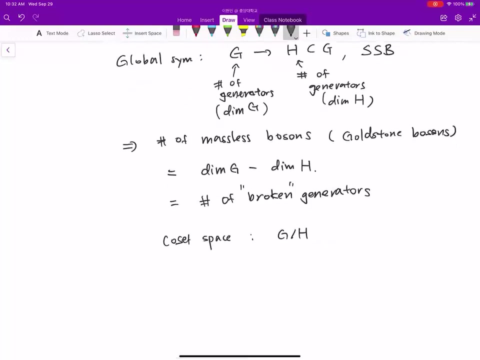 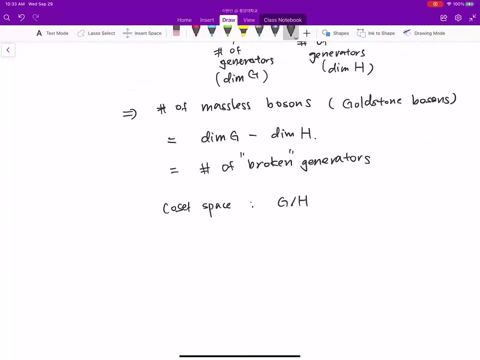 so wrenching variance is required, otherwise this goldstone theorem does not apply. so in some, in some cases, in condensed matter system, uh, the goldstone theorem does not apply. so discounting the number of mesh exposures is not. it's not the same. so so because of the massless versions, those are typically problematic for phenology. 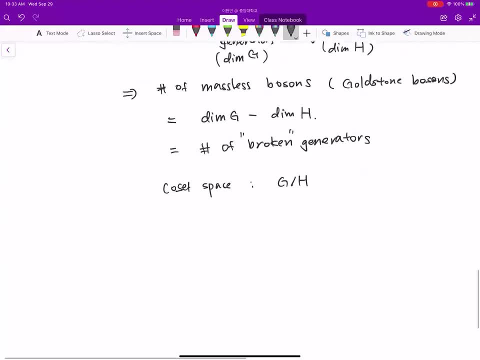 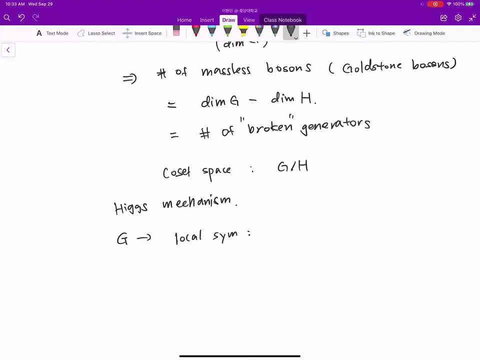 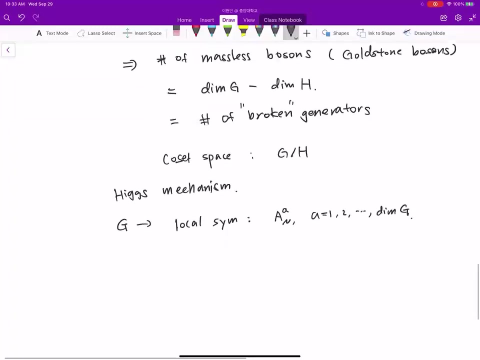 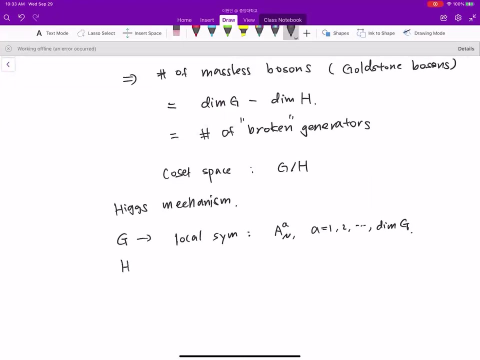 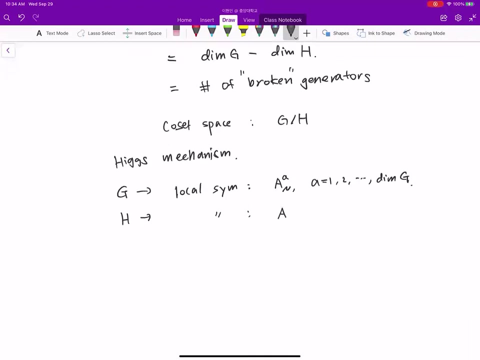 so we need to eliminate them. so his mechanism tells you. so this method is number. so if you promote g to local symmetry, then you need to introduce the gauge field, because the h also promoted to global local symmetry and maybe so i'm labeled the indices for the gauge field differently. 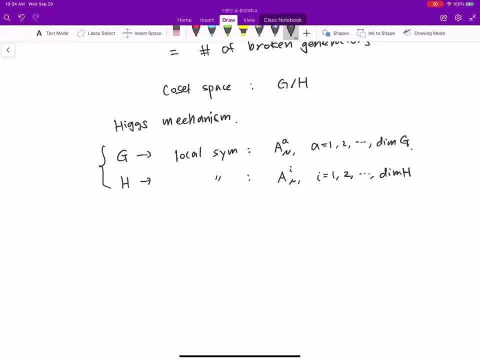 then, in this case, some of the- actually this a, uh, i mean this a- are the same a, but you are missing something. so these are massless. we are counting. this is massless gauge versions only, but there are massive gauge versions which do not belong to the massless gauge versions for h. so so there are massive gauge orders. 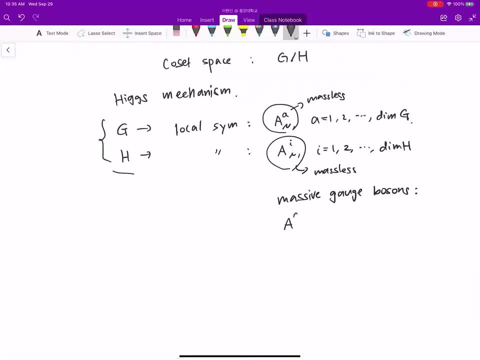 so those are, let me call a u and this uh uh, i don't know how to call this, just to let me ordering in this way: so this engine h plus one. let me order the gauge index in this way, so massless gauge versions are listed in this way on up to dimension h and the other. 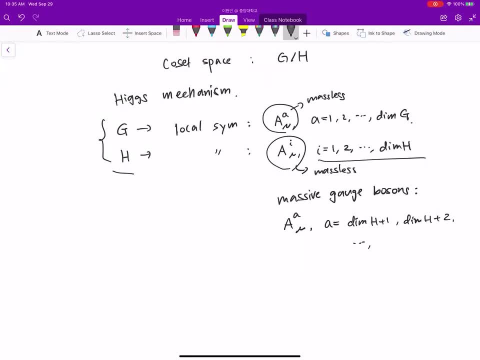 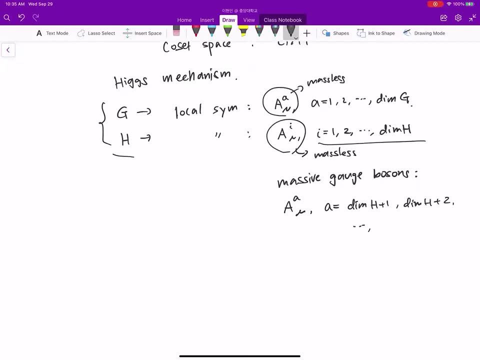 supposed to be massively small gauge versions before symmetry breaking, labeled in this way: from dimension h plus one, dimension h plus two, etc. until dimension g. uh, so if massive gauge version appears after symmetry breaking of g, if the symmetry is broken already to from from g to h. 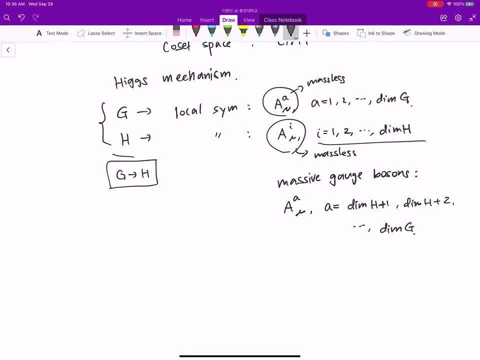 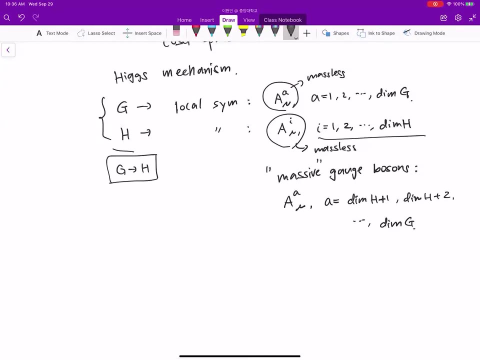 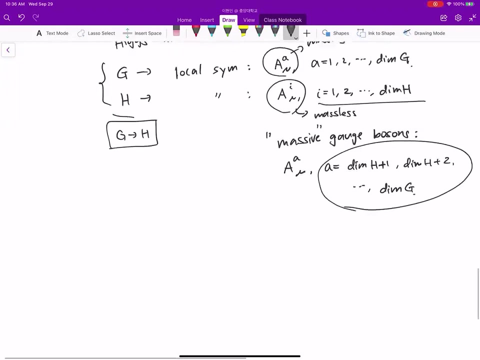 so because h is smaller than a g, you must have broken symmetry. the sum of the massless gauge versions get massive, and here the broken massive gauge version is the number of massive gauge versions. you see how many of them, so just you can count the indices. so then the dimension: number of massive gauge versions. this one, right. 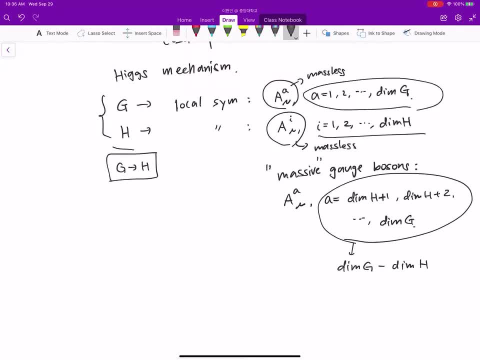 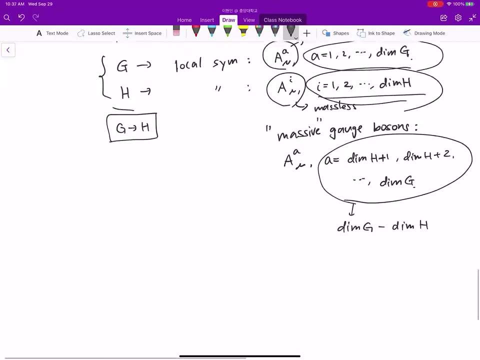 just to. this is the full gauge versions, and you have a dimension, and this is the remaining massive gauge versions. the difference will be the massive gauge versions. So you then you have actually the broken generators. number of broken generators: I think the number of broken generators are the same as in the global symmetry. the difference is that we 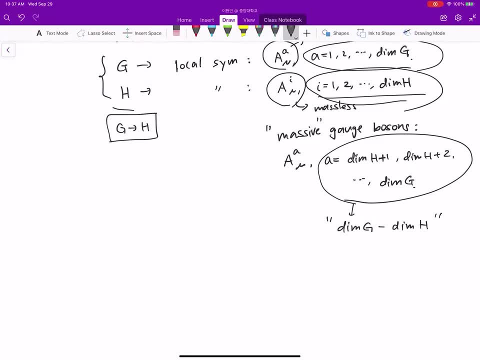 have gauged versions. In the case of global symmetry, there is no gauge version, The massive gauged versions. we know that there is longitudinal polarization, So there are three: two transverse plus longitudinal. So there are three right, two transverse plus longitudinal. So these are the three devices. 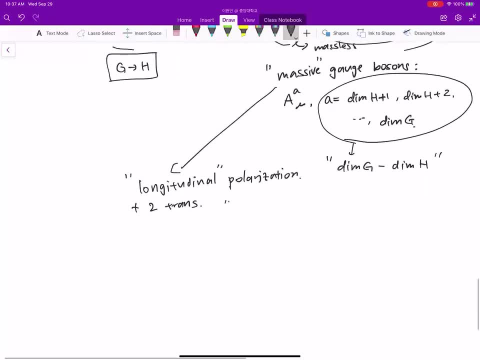 So there are three devices: two transverse plus longitudinal polarization, and then So this longitudinal component- actually we call it Higgs mechanism because the would-be Goldston version- So we have, we have this amount right in global symmetry. 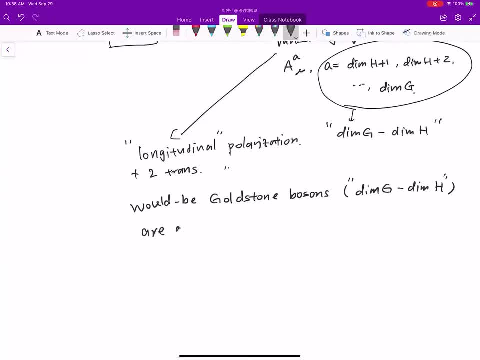 but this would-be Goldston versions are eaten by this massive gauge versions. So there are number of massive gauge versions is the same as number of the would-be Goldston versions. These are not Goldston versions. So when you think about Goldston versions, 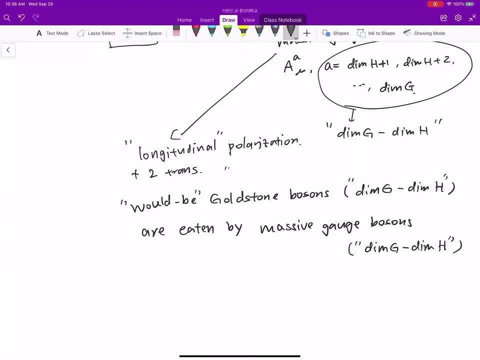 in global symmetry. they are physical degree of freedom, but these are otherwise kind of, otherwise concept. So this symmetry is not local symmetry. This degree of freedom will be physical. Goldston versions. So these are eaten by massive gauge versions. So, counting, you have a. 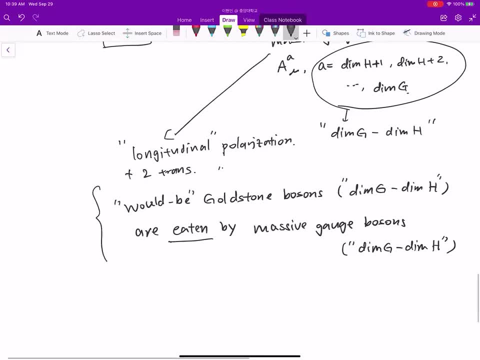 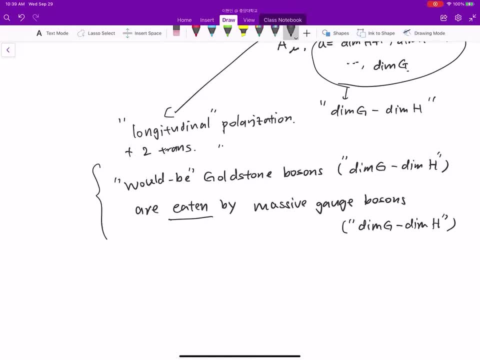 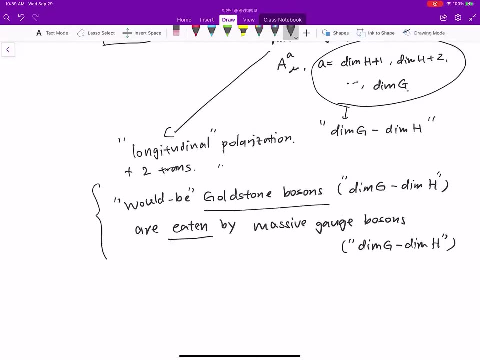 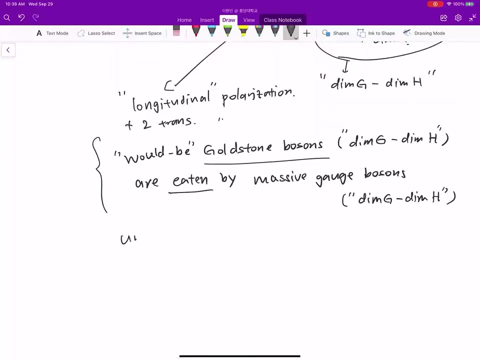 I mean the correct counting of the number of degree of freedom. So then you don't have. you don't have to discuss the Goldston versions anymore, just that they are eaten And the unitary gauge will be in unitary gauge. 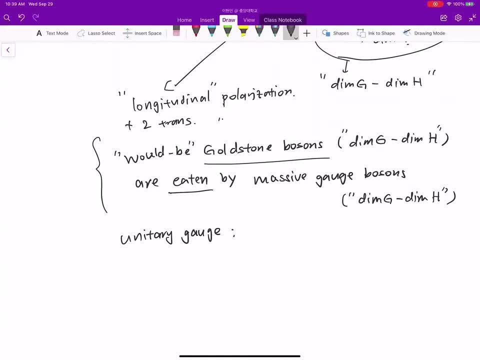 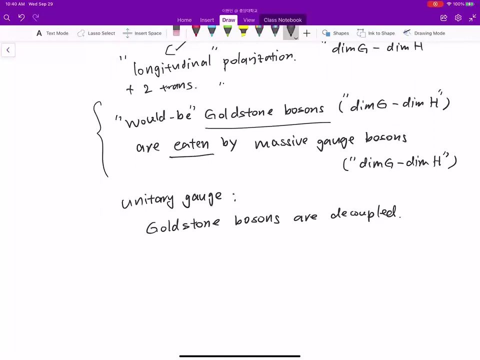 Goldston versions do not appear. We call Goldston versions the decoupled, so do not appear The decoupled. I mean the Goldston versions also carry some masses, depending on the gauge condition, So sometimes they are massless. 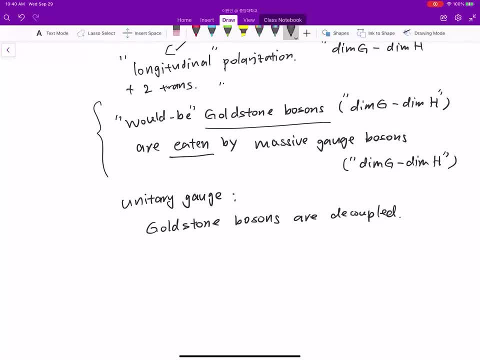 They appear in the Lagrangian. Sometimes they are, you know, massless. Sometimes they don't appear because their masses are very large and infinite. Essentially their mass is infinite. So they don't appear in the Lagrangian. So this is the 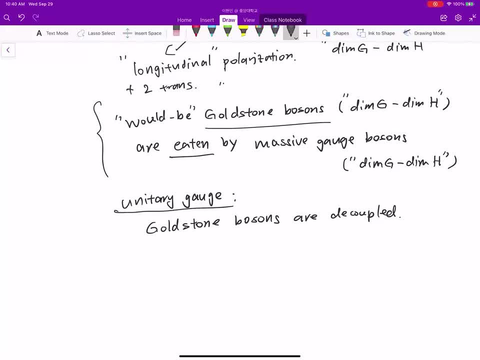 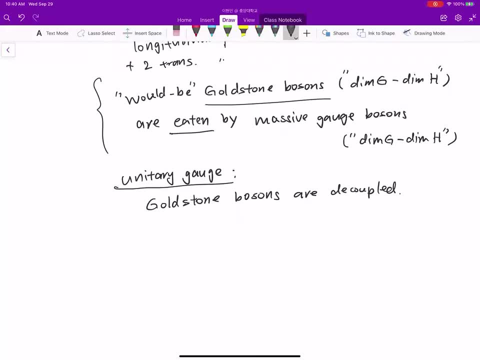 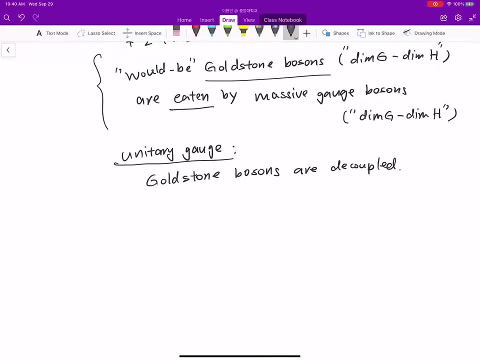 we call unitary gauge. You don't see Goldston versions in the Lagrangian anymore, You only see massive gauge versions. So I think that this is the general statement. If you think of breaking of small group, larger group to small group, 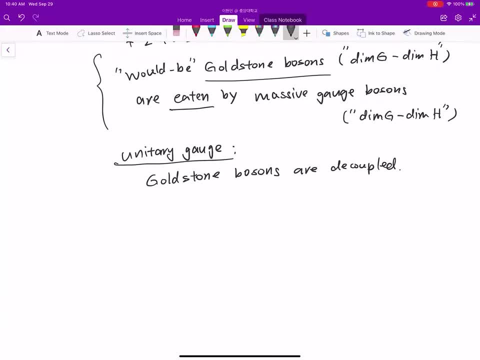 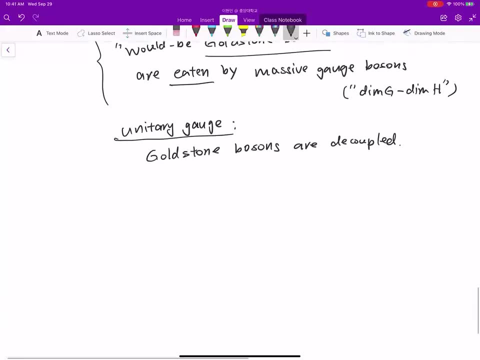 this discussion would apply. So there is no problem because of this, massless Goldston versions anymore. So now this: we discussed electroweak symmetry breaking. So electroweak symmetry breaking depends on the potential right Higgs potential. 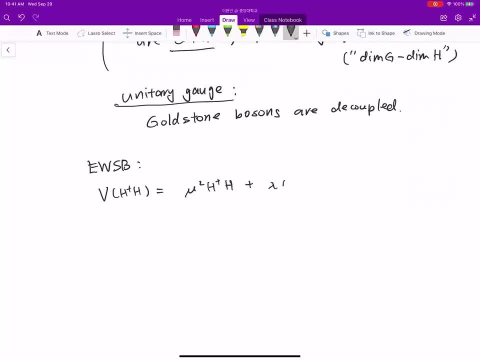 It's a simple form. And the mass parameter? we take the mass parameter mu square to negative. So we look for non-zero vacuum expectation value. So it's a minimum of the potential. So minimum of potential. simply, we look for constant value of Higgs. 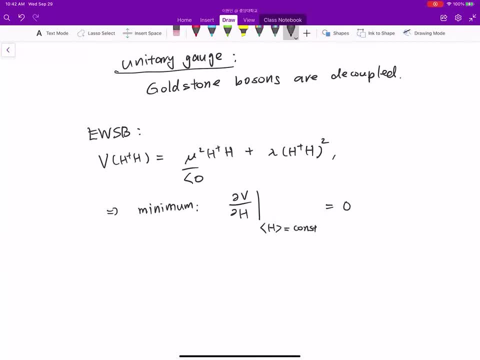 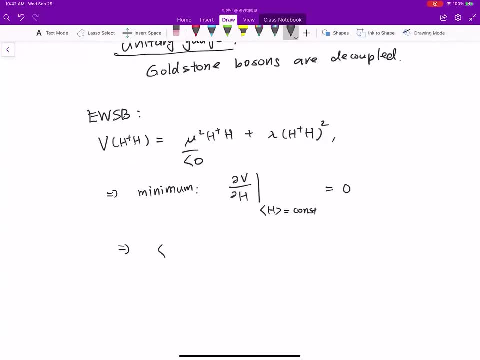 which minimize the potential Higgs potential. And then, as in the simple, I mean the U1 symmetry. you can find that I mean here we need to be careful about assigning the vacuum expectation value because of this, because instead of one complex 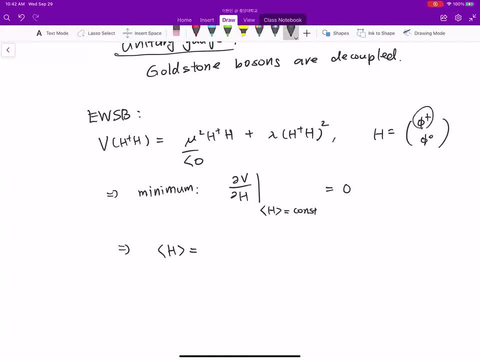 there are two complex fields, And the upper entry we have a plus charged, plus charged scalar field. The downstairs we have a neutral, So that this plus charged scalar will be eaten by the W version, the charged electroweak gauge version. 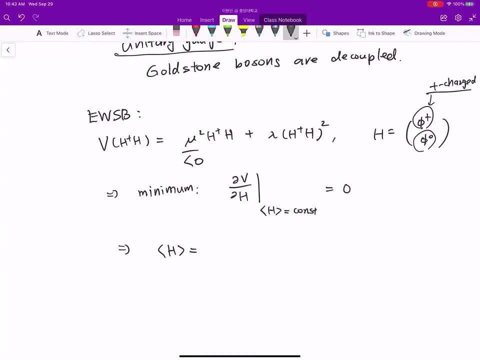 So I mean, in any case, this complex scalar could not get a vacuum expectation value. So you are breaking the charge, So you shouldn't break electroweak, you want electromagnetism. So then in the background it's your vacuum expectation value. 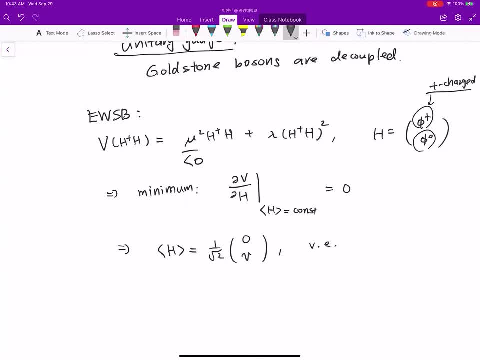 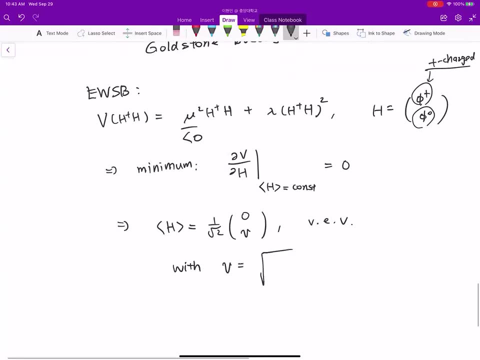 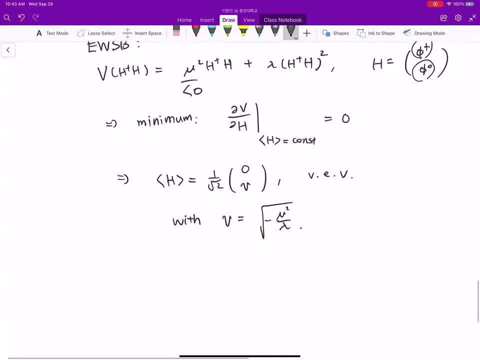 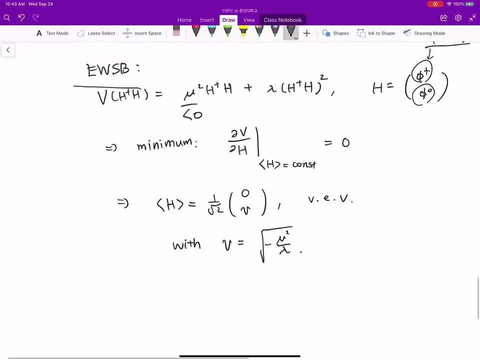 So this is the vacuum expectation value. So this V is given by, in terms of mass parameter and Higgs quality coupling, As you remember. it's simple, right, So? but this is the vacuum, But in order to describe the physical spectrum. 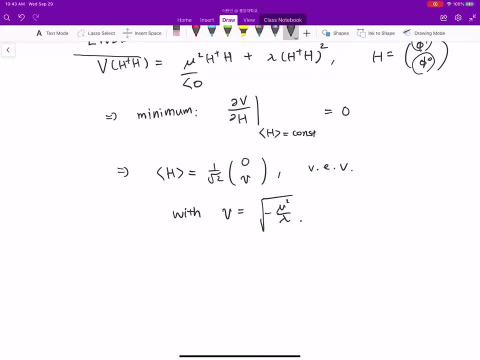 the vacuum. the identification of the vacuum is not you know, so you need to do the perturbation, So its potential. you see we have this shape If you take the section. so this the real part of pi zero. 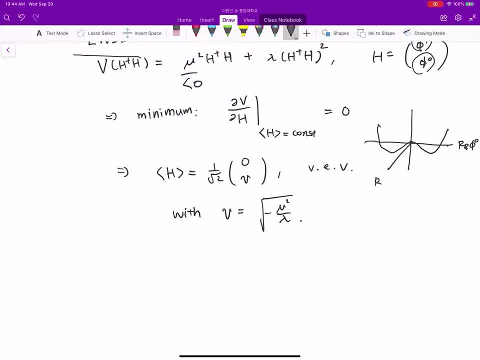 and this octagonal direction and the imaginary part, for instance. So here we have this V, This is its potential. So we are not interested in this more complicated potential. But the non-zero vacuum expectation value is taken only along the neutral component. 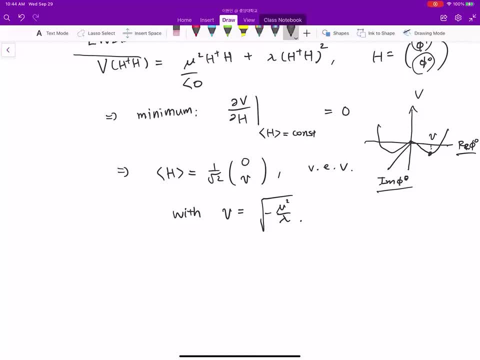 So, and then we have, we have two directions to go. I mean this, this way So, this way So, and also we have. I mean you can do a perturbation, So perturbation around the vacuum. 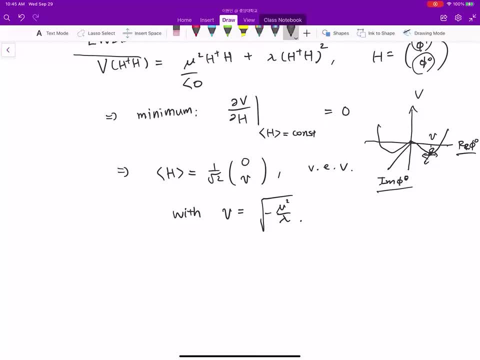 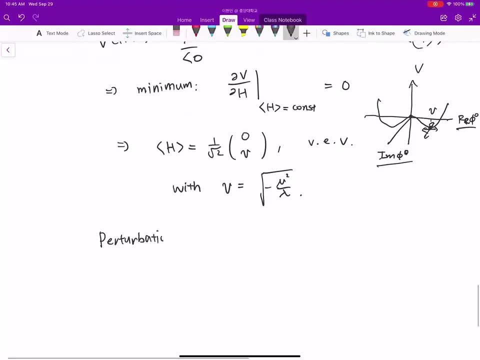 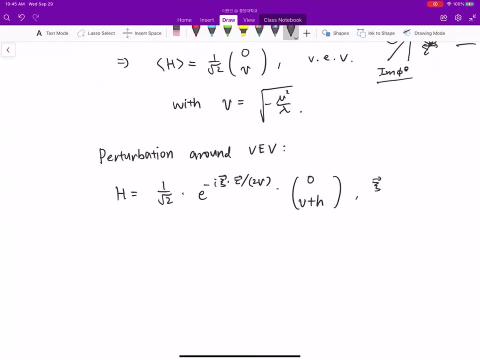 in this neutral component, also charged component. So then the complex scalar, So perturbation, you can parameterize in this form. So in this form: here xi and h are four real scalar, So this is not the unique choice. 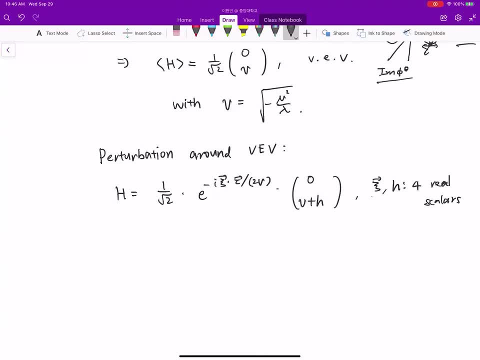 This is one of the choices for perturbations. So this xi and h, those are filled with the function of space-time. So these are four real scalars. There are four real scalar perturbations, as you remember, neutral and charged component. 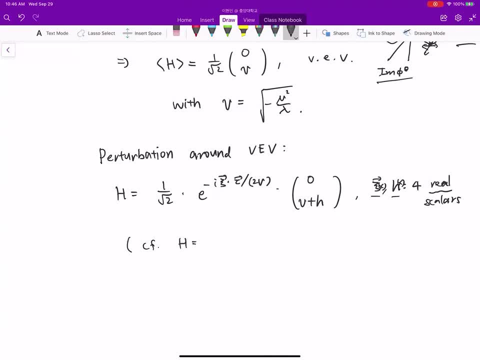 But in principle you can choose different parameterization. This is a kind of polar coordinate representation And you can take like a different parameterization principle, But in this parameterization you keep the same number of degrees of freedom. Sorry, this is. 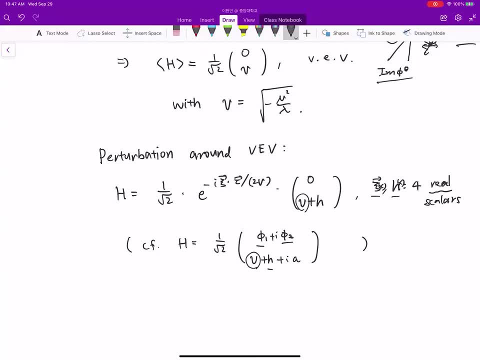 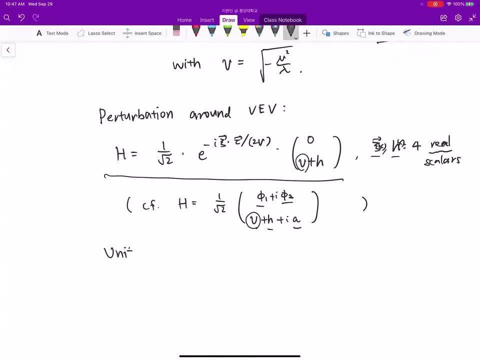 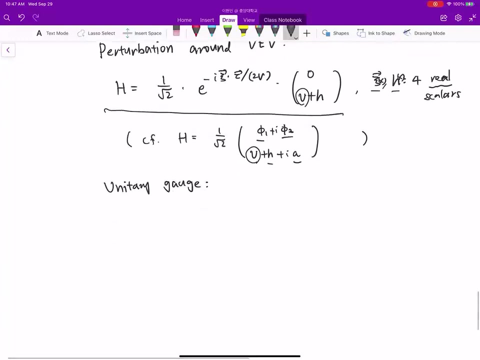 around the vacuum. expectation value: small, I mean constant. the background: you have perturbation. The degree of freedoms: number of degrees of freedom is the same in both cases, But we choose this one And the unitary gauge, So we can. 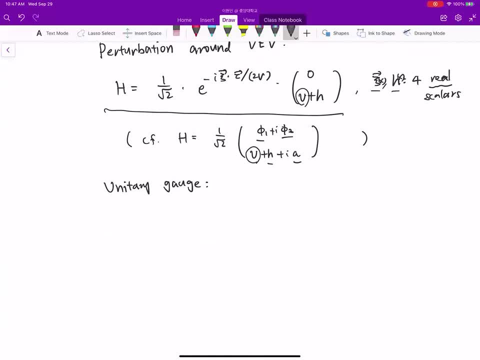 transform the gauge transformation, So Higgs transform. By the way, this factor, the free factor, let me call this U inverse xi And U of xi. we are making SU transformation for Higgs. Then we have a U inverse in front of it. 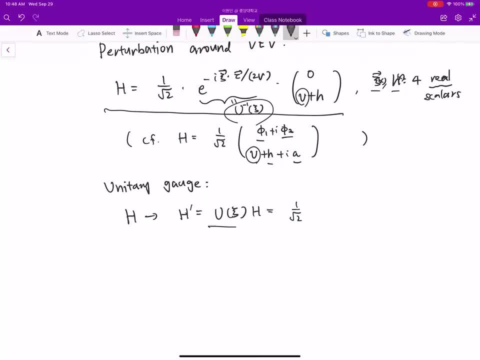 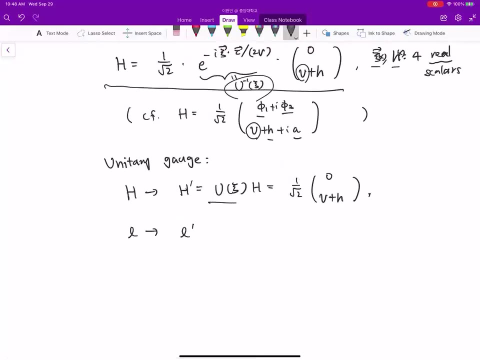 And that U inverse is canceled by this U, You are left with simple form for the Higgs doublet. And also, when you transform Higgs you have to transform the other field too, And also you have to transform the gauge field. 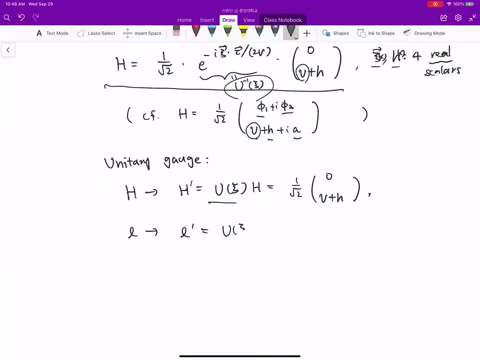 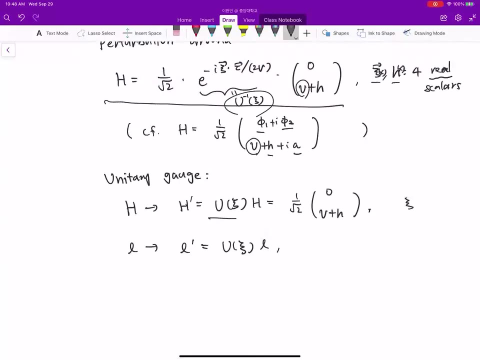 So so lepton, doublet, also transformed by the same transformation parameter, So you can think of this- is to, let's say, xi parameter. I mean it is equivalent to choosing the transformation parameter to xi over 2V. So this is the SU transformation. 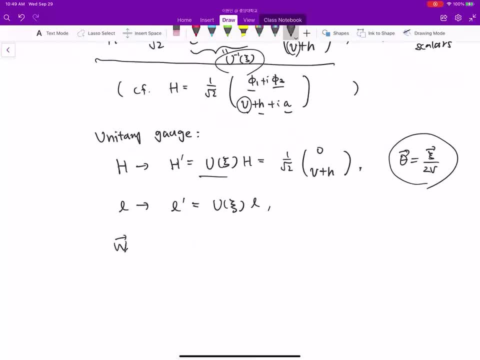 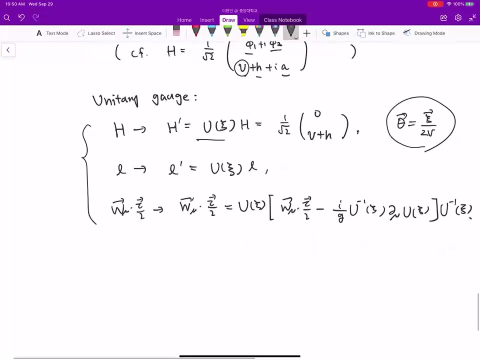 And the SU gauge field transform. I don't know. Let's do this Just a specific kind of specific transformation for the SU. This one I don't know. So you can see the shape of the ball. The shape is not the same. 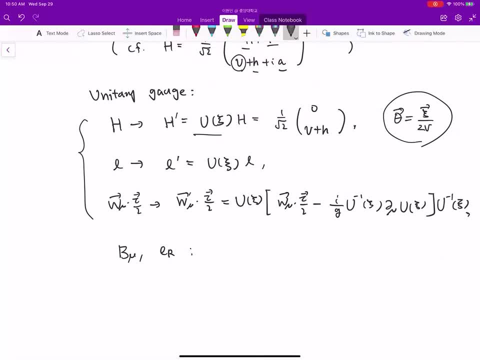 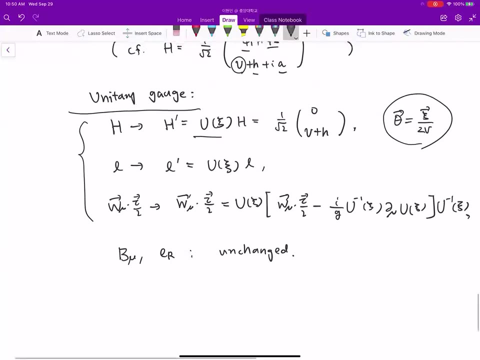 as the previously, Let's see the shape, So it's all the same. And then you can see the shape of the ball in this simple form, and the goldstone versions would be goldstone versions. so of course, here the H is a Higgs. 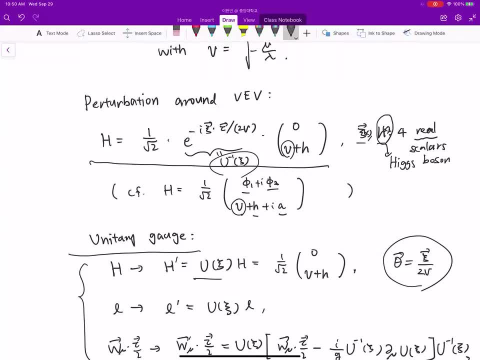 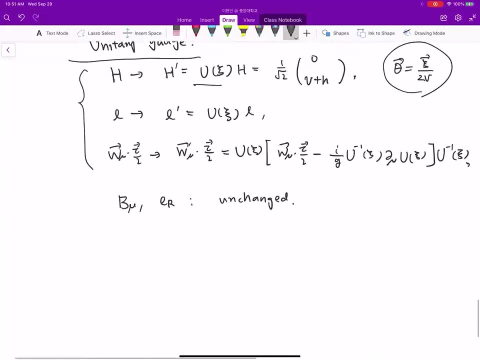 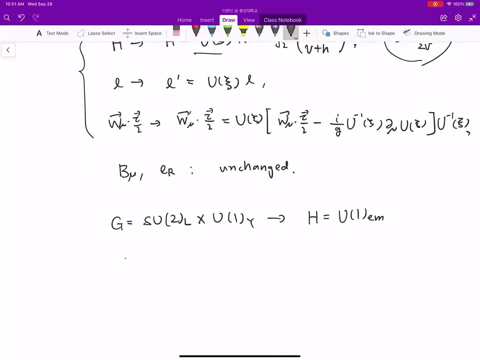 Higgs version and this psi would be, would be goldstone. so in the standard model we know that the local symmetry, so g, equal to SU, SU, cross U hypercharge, broken down to small group, which is one electromonetism. So the dimension of group is: we have three from SU, one from hypercharge. 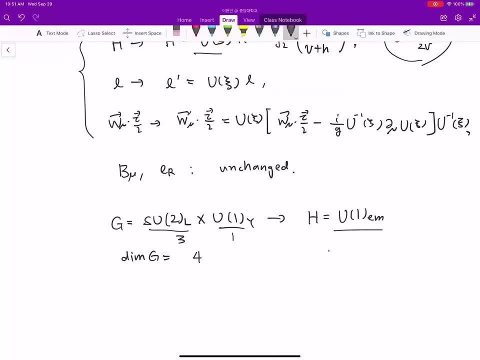 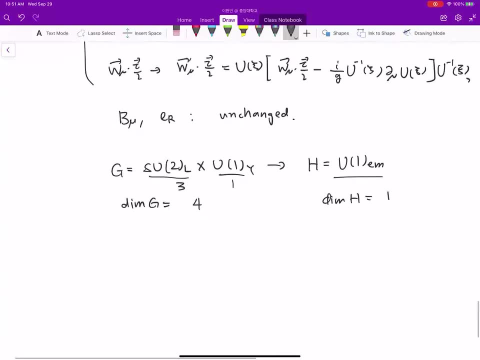 there are four, The U. we have dimension of H equal to one. There is only one generator Because of that, as you can see, the would-be Golduston versions. so, number of would-be Golduston versions equal to dimension G minus dimension H, which is three. 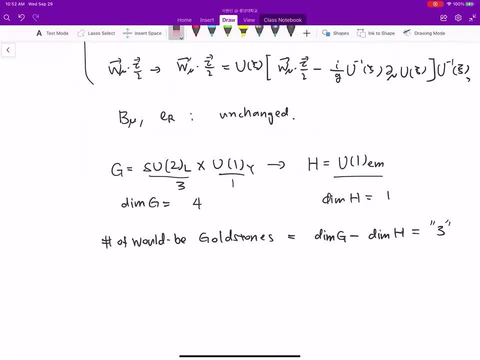 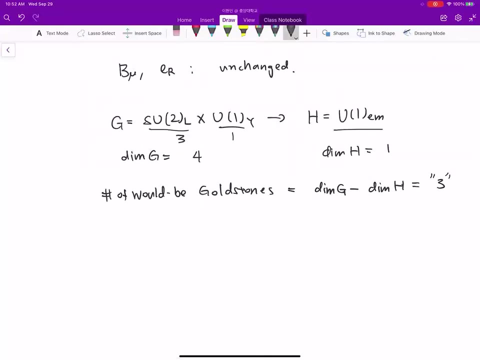 So if this SU is global symmetry, you have three Golduston versions, But we have a gauge field, So because of that we have a mass list. We started from W. Now we have a log gauge symmetry. this is the gauge symmetry, So we have three of them. 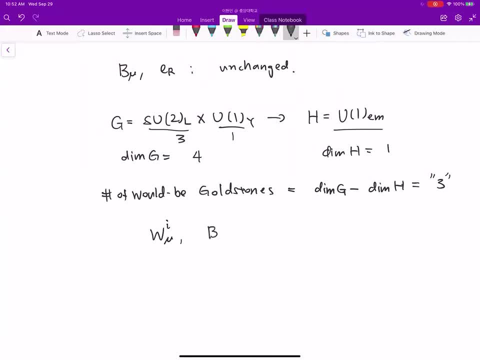 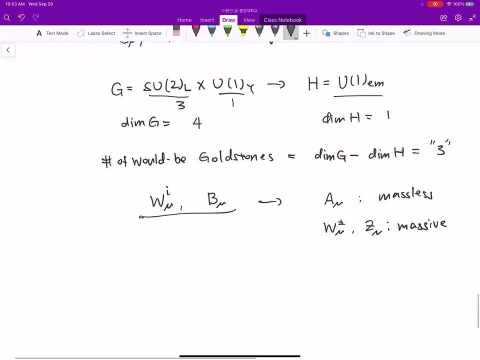 three gauge fields for SU and hypercharge, And those become photons. So one mass list and three massive gauge versions. Three is the plus minus charge, W version and G version. So this is mass list And this is mass list. So these are mass lists. If for electroweak symmetry, so electroweak symmetry. 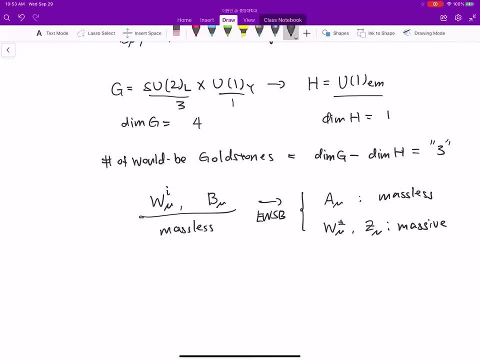 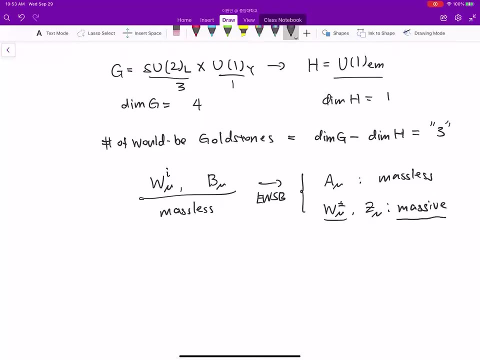 We have. just the number of degrees of freedom is the same before and after. So then you can see that the massive there are three. So these are complex. So in the real degree of freedom there are, there is two real degree of freedom. 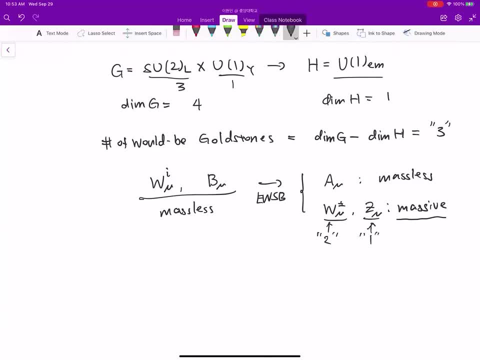 So one because of the three, three gauge models. So it counts. I mean, the number of degrees of freedom is the same. The number of massive gauge versions is the same as the number of would-be goldenstone models, just broken generators. 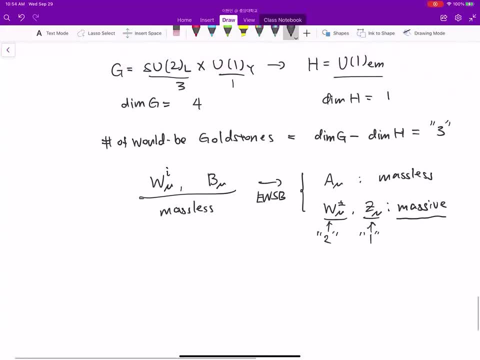 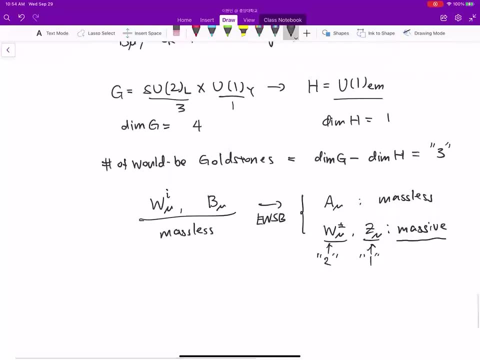 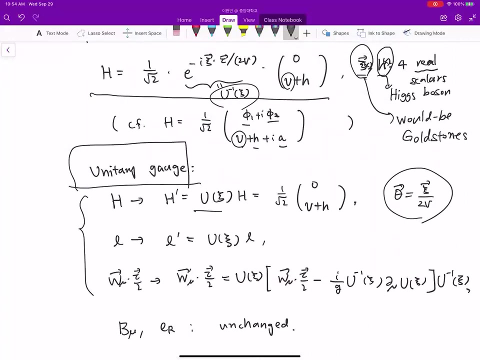 So his mechanism is working for the standard model in this sense. So because of that we eliminate it. We choose the gauge conditions such that this unphysical degree of freedom do not appear. So that's the unitary gauge. So if you want to keep this would-be goldenstone version in the Lagrangian, 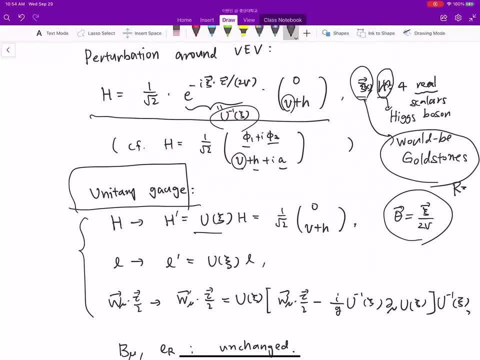 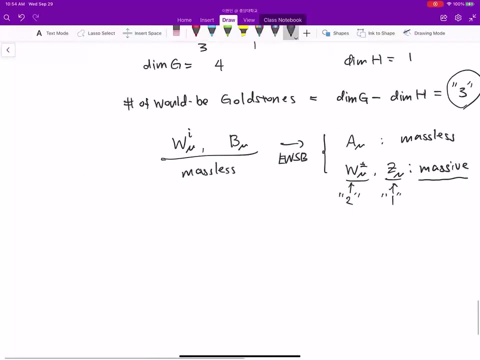 then we call this arc psi gauge, general arc psi gauge, Because psi, I don't know this psi. there's also gauge-based vaccine parameter. We call it psi or this psi. also It stands for the goldenstone versions, So arc psi gauge. 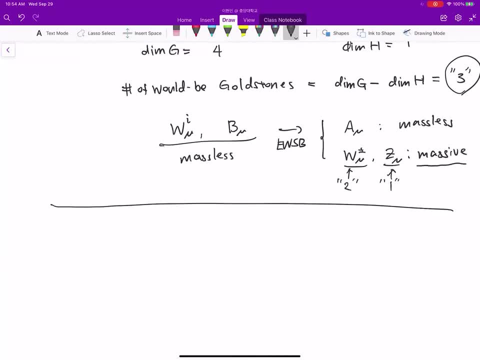 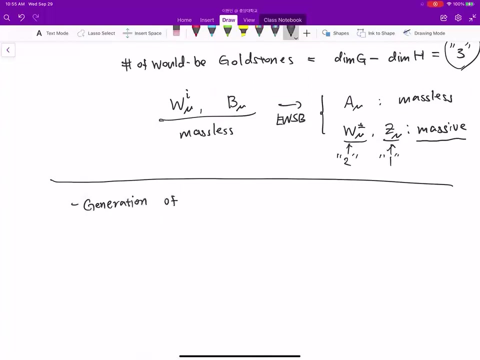 So let me go to now physics, The details of the generation of masses and the Weinberg angle. So the current. from now on I'm going to discuss generation We'll be using, And then Interaction terms, Of course, in that interaction terms, And also neutral current and charge current interaction. 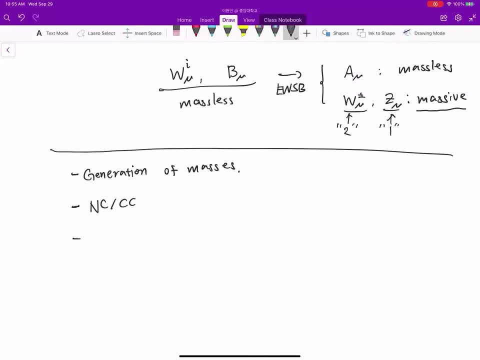 And the next goal is to discuss GIM mechanism and CP violation. So we call this a flavor and the flavors include the generation of masses, also the structure mixings and CP violations etc. So GIM mechanism- using I mean the flavor mixing- is crucial for GIM mechanism to work. 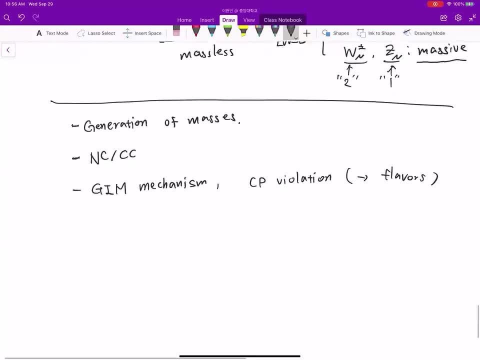 So we are going to discuss this one. a neutral current and charged current are mostly. we are going to discuss neutrino scattering process and beta decay and muon decays. So first let me discuss generation of masses. do you have any question? I forgot. 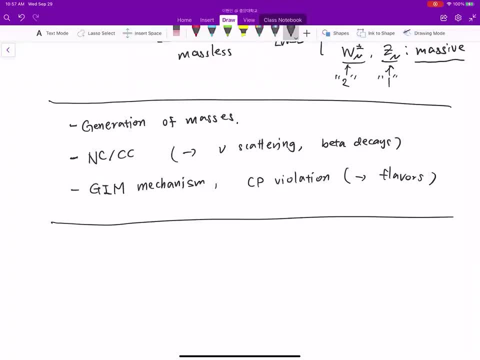 Okay, do you know Jin Young's email address? Jin Young, Kim Jin Young, if you can send a message to her. So if she is missing this lecture, I don't know if we can follow the coming lectures. And then also there's another student from Professor Ha's group, Sunhee Shin. 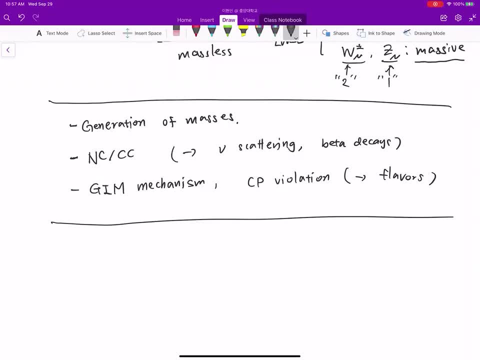 So she never. She has never taken my class Until now. I don't know what what's going on. So if you have during the break time, maybe you can send a message, or if you have a phone number you can talk to Jin Young. maybe Jin Young knows about the other students, okay. 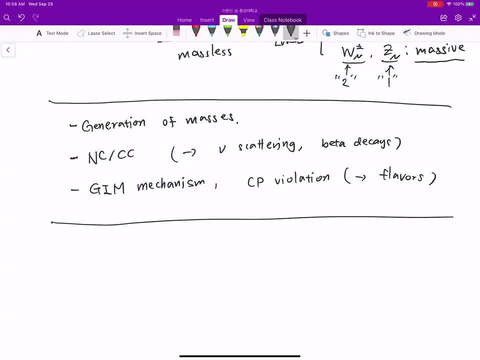 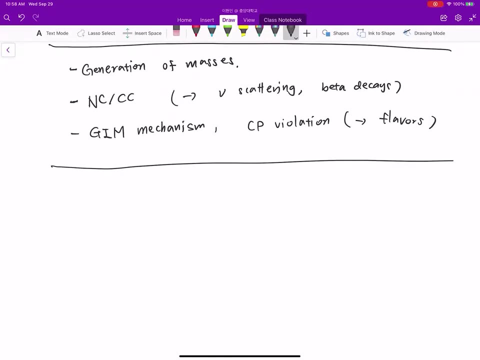 Some, some, some of you, if you know them. Okay, so me. Do you have any question? Okay, So, let's go to the next, And then generation of masses. so, So, there are generation masses that you have. you may already familiar with that. 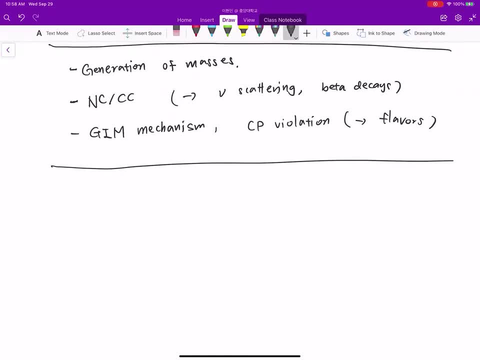 First, let me start from start, simple. So I think the use of the mass is more than a mass. you know you have a mass of elements Like: what's the mass of the target half? Is it Okay? Yeah, 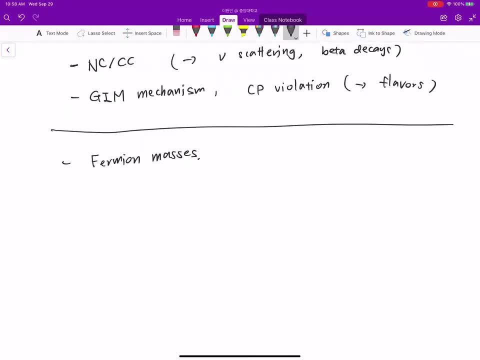 if you extend the standard model including dark metal, i think almost the same story we need to follow. so i think the if you, if you are familiar with standard model, i think that there is no problem for extending the standard model. so i think it is important. so formula math we choose. 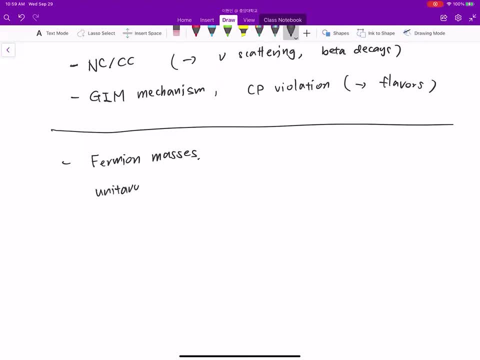 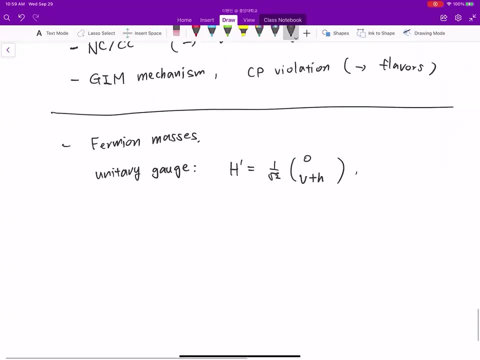 the unitary gauge. so then the yugawa interaction. uh, we are choosing the gauge transformation, we are making a gauge transformation such that the higgs doublet takes this simple form. and then yugawa interaction, written should be written in terms of the prime, prime quantities right in this gauge. so 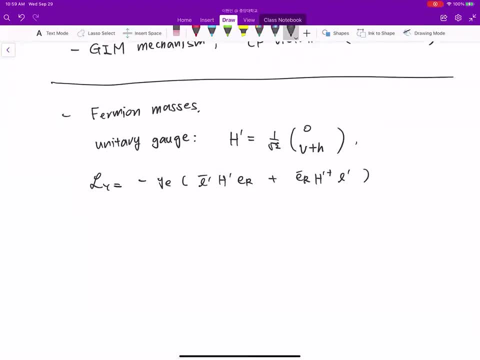 just prime. we have a prime for lepton and doublet higgs, doublet and just put the uh matrix form. so doublet is a neutrino, an electron right, and then h bar is the square root of zero h and the right-handed and the other part is just the permission conjugate. 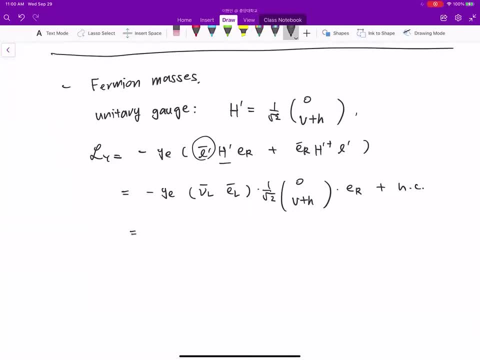 so just this matrix multiplication you have to do right. so this one and this one electron only survive. the neutrino does not appear. so even if you have an interaction to neutrino- it looks like there is interaction to neutrinos in the unitary gauge- there is no interaction to neutrinos. 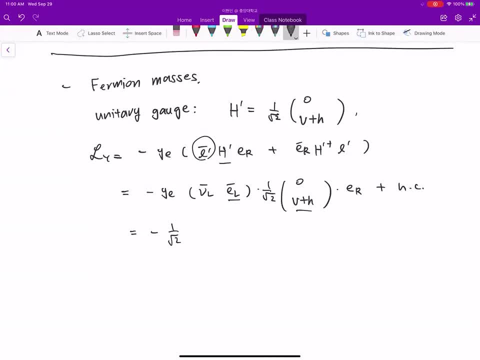 but certainly i think there is a kind of neutral whether or not neutrino has interaction to higgs with gauging dependent statement. so at least we can say that in this gauge there is no interaction to neutrinos, so you can expand it then. so just multiply this, one right and then another. 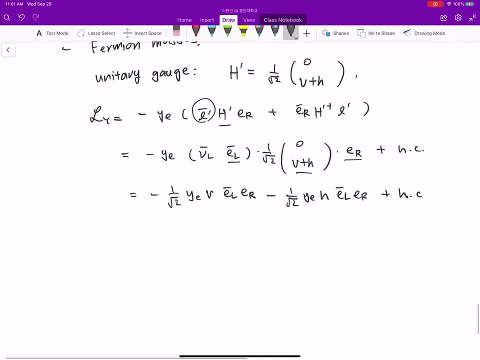 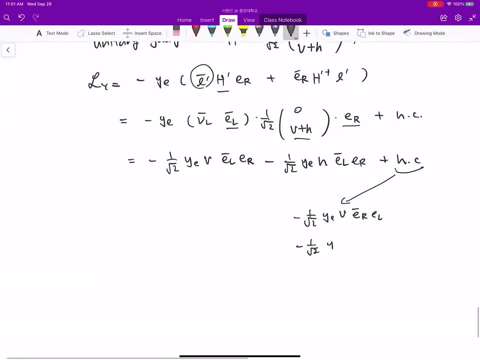 so how many? conjugate contains minus y, e, v, e. the left and right interchanges right, so that's why the same coefficient here we have a left, right interchange it. and this and four component notation we can write down in terms of this projection operator for right-handed and this one also projection operator. 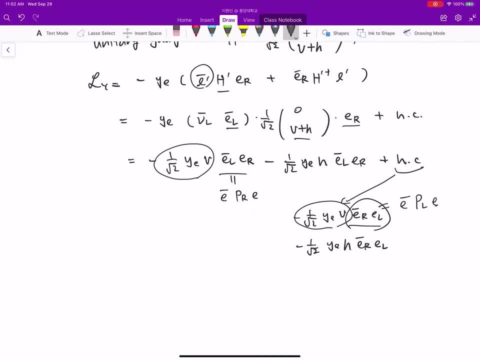 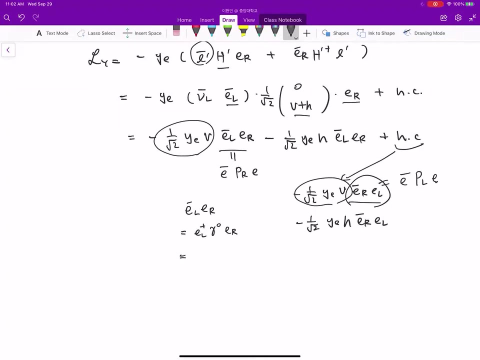 with the left-handed. so, because you have to remember that there's a gamma zero, so e l e, this is the e dagger gamma zero. okay, so because of that, um, you know that this is the in terms of projection operator. you can write down this way: and this is the. 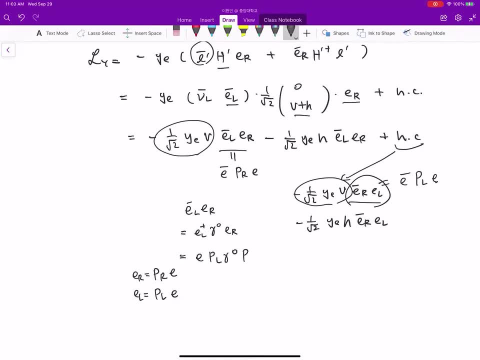 e, p and comma zero, p? r e. so, in terms of four components, vena e, if you can see, after interchanging this becomes this one, and also p? r, square equal to one, and also p? r p? r square equal to p? r. so because of that, 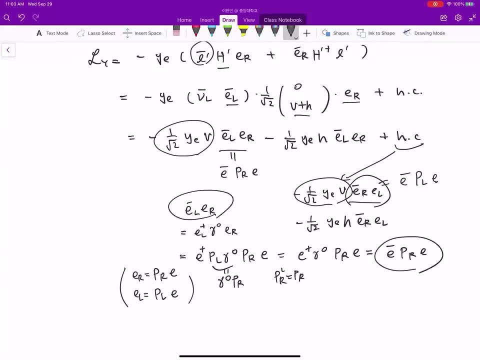 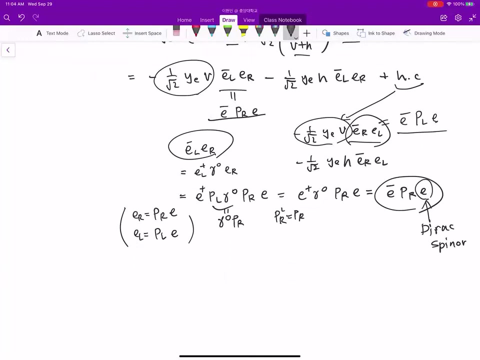 we can write down this: l? r spinner to this, uh, in terms of dirac spinner. so this e is a dirac spinner with the projection operator. so because of that, we have a projection operator, p? r and p? l appearing with the same coefficient, so p? r plus p? l, equal to identity. so because of that, 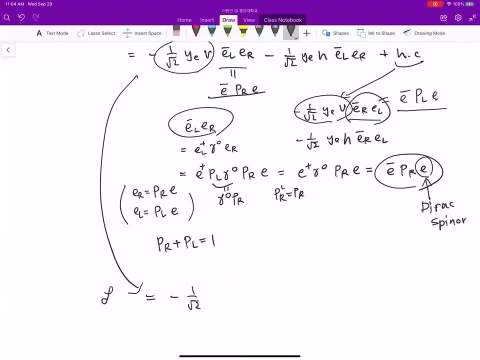 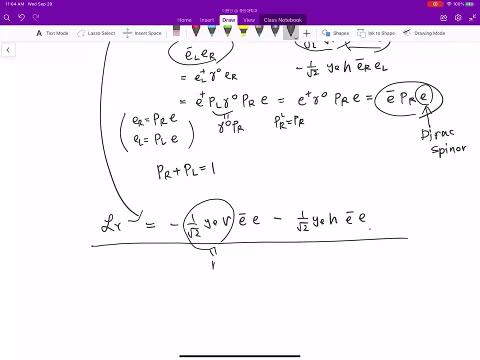 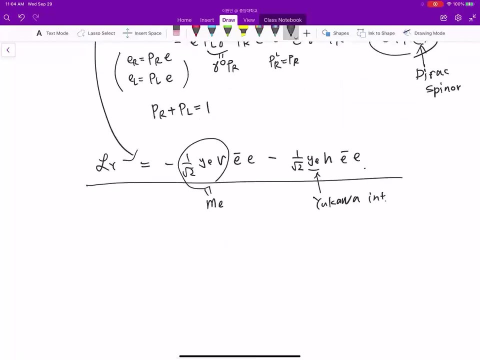 this can be written down. so you have our interaction, including the complex conjugation. thank you, it's in. this is a simple form, very simple, and the formula: masses can be identified, electron mass is identified with the coefficient and this y is ugawa interaction. so you've got interaction, uh. 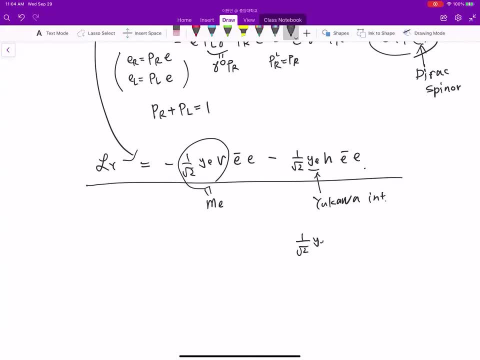 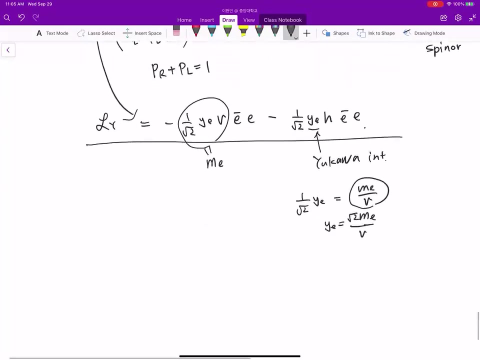 square root 1 over square root two, two times y e and here from the electron mass. so y e equal to in terms of electron mass. here, yes, because of that, the ugawa interaction can be written in terms of the electron mass. so, as you, if you have a larger masses, then you have a larger. 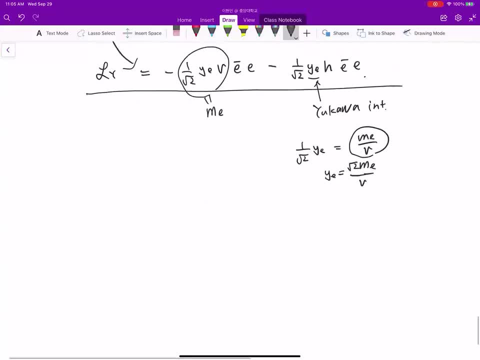 coupling to Higgs. so so Higgs-Ugawa interaction depends on the particle mass because of that. so if because top, in the case of top quark, the top quark is the heaviest particle, you could have strongest interactions between Higgs and top quark. so this discussion can be also applicable for 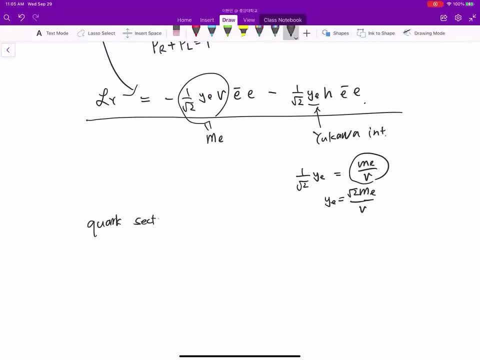 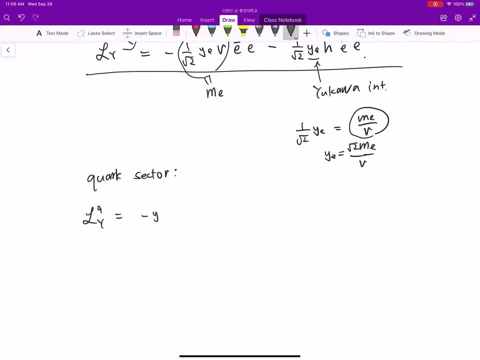 the quark sector. so quark-Ugawa coupling. you can introduce in a similar way. first let me introduce down type quark, because the so in the quark sector. so let me first write down the representation: so quark. it is more complicated, right? so this way: 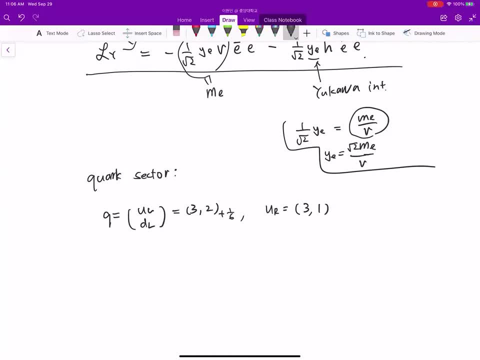 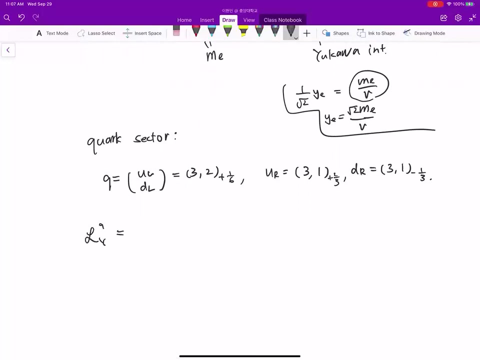 for the lateral sector there is no right-handed neutrino, but here we have a right-handed for both up and down. so this representation and then you can construct the most general renormalizable. so renormalizable, because here the renormalizability is required, otherwise you can keep adding more terms. so renormalizability. 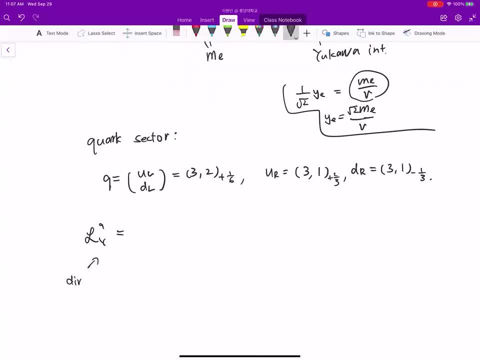 so dimension. so we are constructing dimension, we are constructing the bande in relation to the normalization of these two constraints that I have mentioned in the first part, and that is the in the great operator. so in the last part of the training we already discussed that this constraint does not apply to lower and upper walls and that the operator is smaller than 4 or equal to 4. so because of this constraint of the operator, smaller than 4 or equal to 4, so because of this constraint, is super-renormalizable or is super-renormalizable or is super-rассle-able or is super-relevant or relevant and marginal operator. 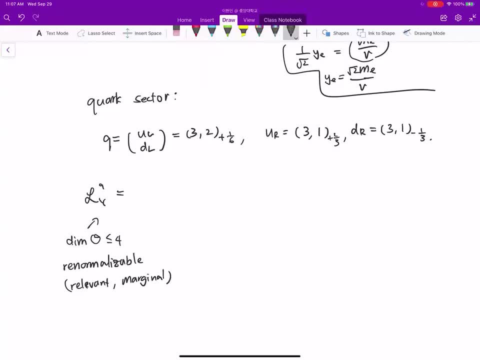 and marginal operator constraint, then this is the most general algorithm you can think of. so first down. so i think the structure is the same as for the leptons, in the case of down type, you are coupling, so down top, you are coupling. so instead of lepton doublet, quark doublet and h and the right-handed down type, 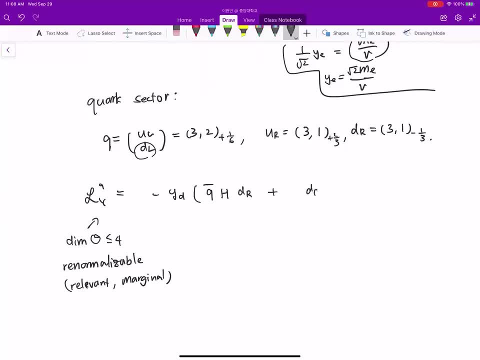 the quark and the complex conjugation, then why you so? for the up quark it's a little bit different, so we need to introduce tilde. so this is it. so also in this case, we consider one generation only. so if you have multiple generations, three generations, then you need to consider flavor indexes too. 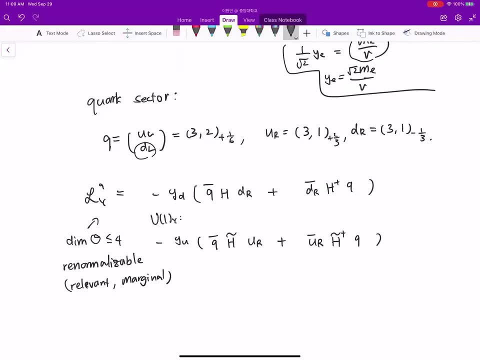 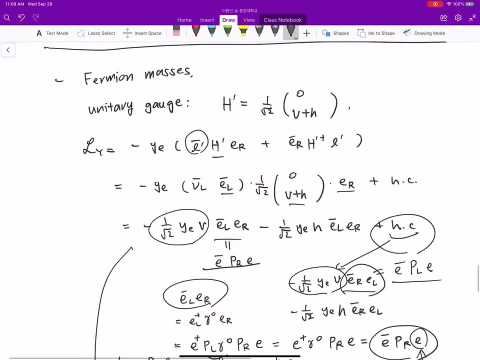 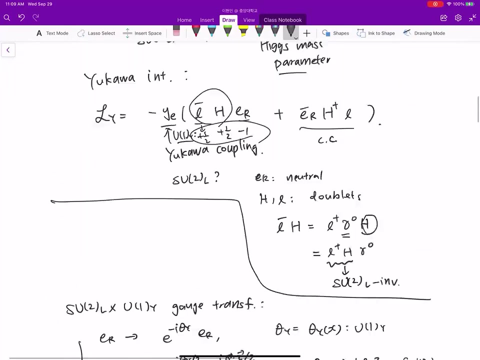 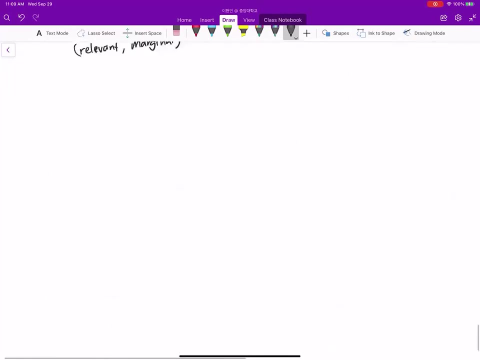 so you can check also hypercharge here, so hypercharge. so hypercharge. so minus plus one sixes. so minus conjugation minus one six. so hicks, was what was the hicks? hypercharge plus minus half, plus plus, minus, plus one half and plus right, so plus one half and down. 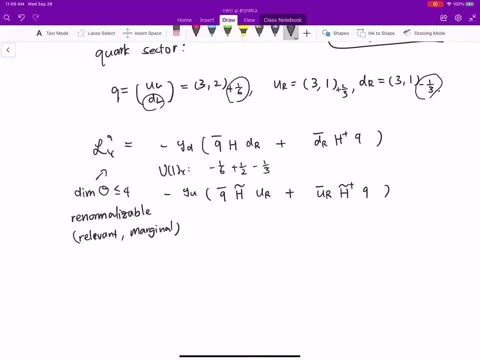 minus. so if you sum up those charges, they are sum up together. so, similarly, so if you sum up those charges, they are sum up together. so similarly, let's say you have a hypercharge, so you have a hyper charge and this one minus six, one sixes, and this h that i just said approaches hypercharge. 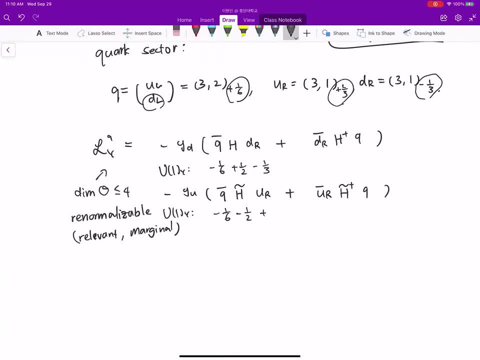 and you are, you are hypercharges here plus the sum up to zero. so these are zero and for su2 and for su2. let's see how that works, let's see how that works, let's see how that works. to just lepton doublet, right is the core, is doublet, is the same as for the hip, for the lepton doublet. 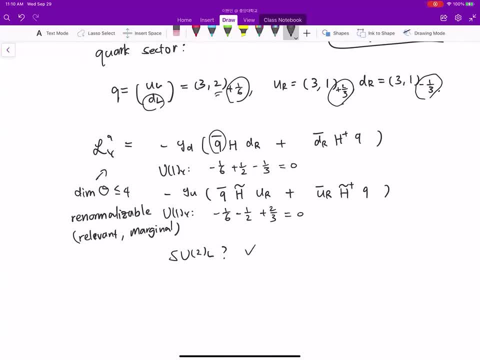 so the doublet sv2 transformation is okay. in the case of quark we need to check the color invariance. the color invariance, uh, the x, w doesn't carry color right. and then this q bar, q is the three. but if you take the conjugate then three bar for q bar and u dr is three, so three bar. 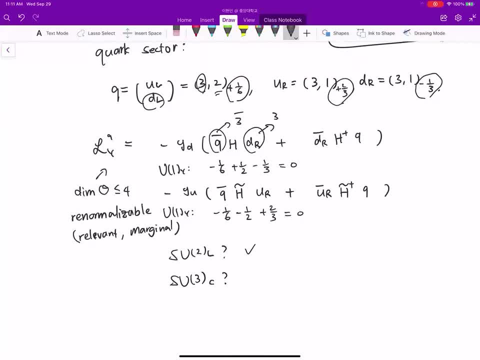 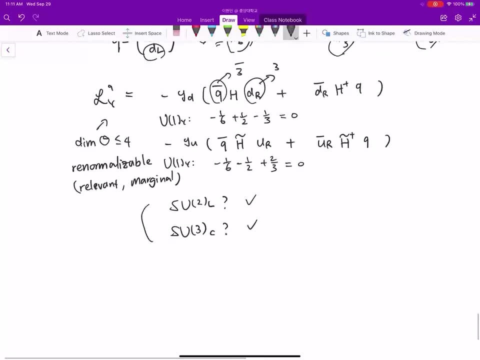 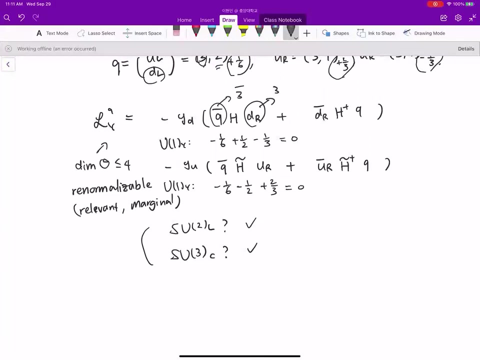 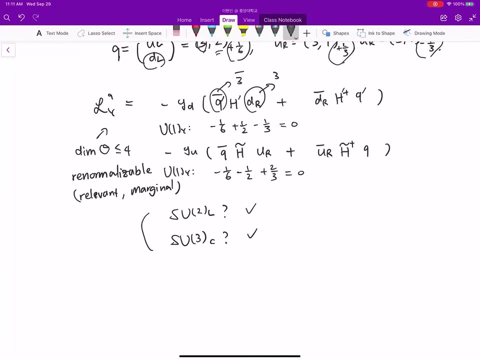 three, so su three, invariant. so this is also- it's okay, so complex- conjugate. so so then just you can follow the same discussion. of course, now in the unitary gauge you need to put prime quantity here in the, in the doublet this way, and just expand them. so similarly you will find that 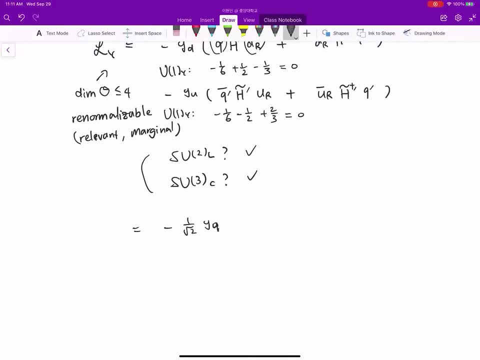 there are a lot of types in this case. the first one is q bar right, because what it is is the gradient, which is the temptation of theurate x. that can be seen if you look at the. the total angle of the gradient is equal to zero and is equal to zero. 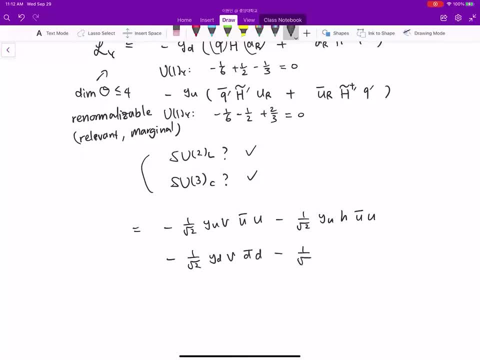 so what you're doing is you're changing your teacher a little bit. the tops that show up right now is the sine, and the bottom ones are simple, so they are just the same thing. so i'm going to remove those and i'm going to add a value to those and i'm going to look at the 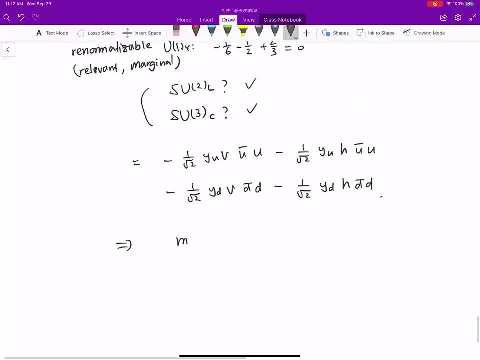 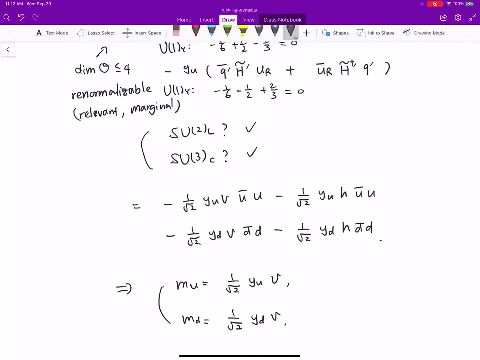 So because of that, the up-type quark depends on Euler coupling and down-type quark depends on another Euler coupling. So we don't know. We don't know the. Of course we can accommodate non-zero masses for quarks, but we don't know. 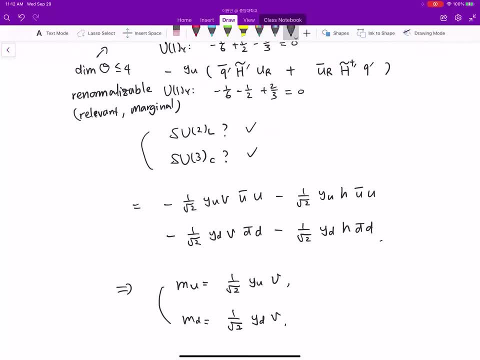 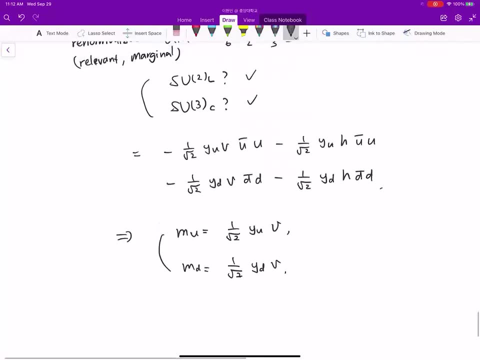 We cannot explain the quark masses. why the quark masses are so small, for instance, for first two generations, for instance? Just, we parameterized the quark masses by the Euler couplings. Let's make a short break and then we can continue to discuss the gauge-vogel masses. 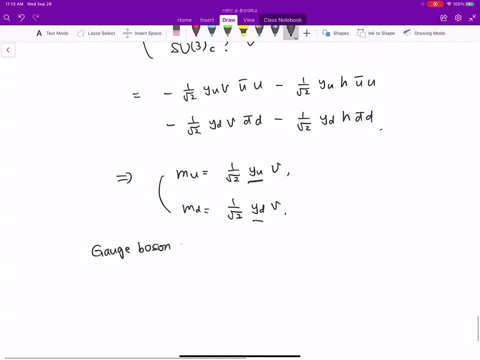 kg. Okay, Gauge-vogel masses, and then neutral current and charged current interaction. I think that for today, I think almost all the interactions we can cover. I don't know about the CKM matrix, but let's try Okay. 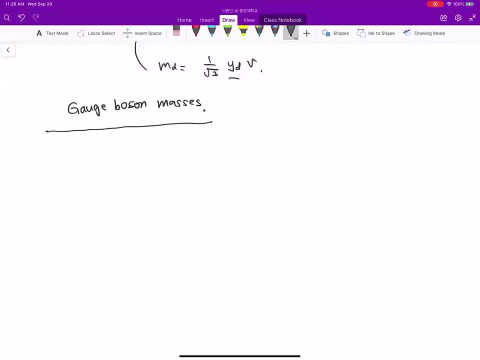 So for the standard model, but also for the extended model with the new gauge symmetries, it will be a good exercise for you. So, again in unitary gauge, we are working in unitary gauge. Okay, Okay, Okay. 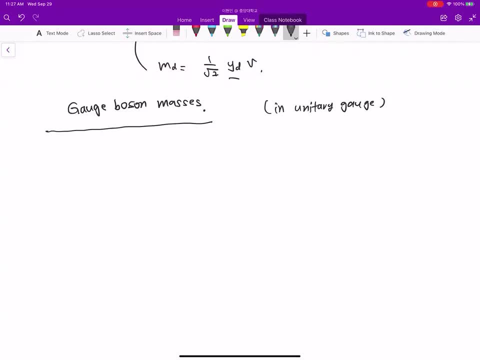 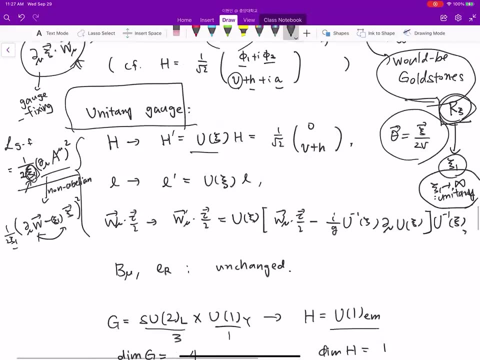 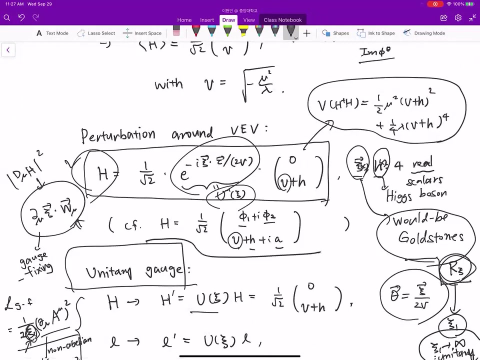 Okay, Okay, Okay, Okay. So any, I mean this unitary gauge is because I choose particular form of the Higgs doublet in this polar coordinate. You can choose this Cartesian coordinate for Higgs and then for the general gauge, not. 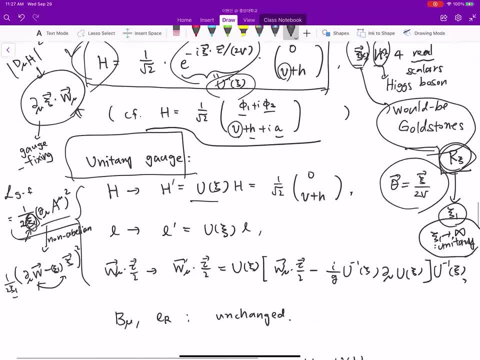 unitary gauge general gauge. So the general gauge depends on this psi one, this gauge fixing parameter- And then you will see the gauge-vogel masses- depends on this psi one. I think that this has to do with this second term in the gauge fixing parameter. 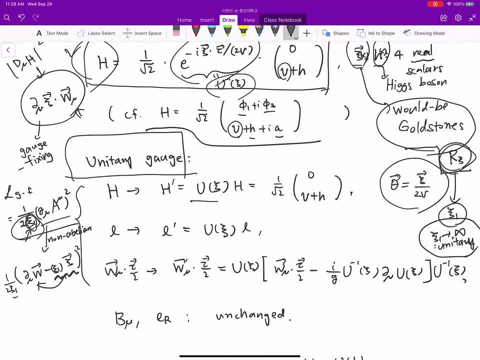 So if we expand that, you have a psi square. Those correspond to masses for the Goldusten bosons. You can say that the Goldusten bosons are Okay. You can say that the Goldusten bosons are massive, which it depends on the gauge-vogel. 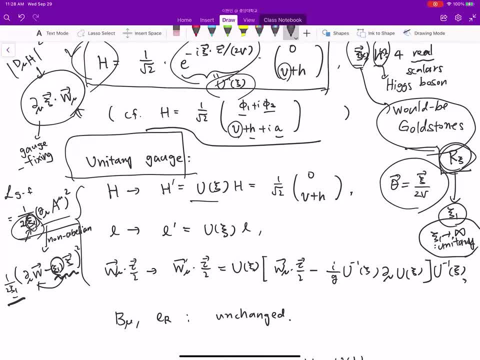 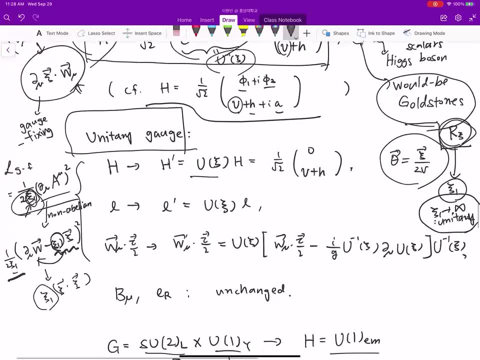 masses depends on psi one parameter. So from there, after expanding psi one, because I Sorry for the same notation- for gauge fixing parameter parameter and golden stone bosons. so because of this xi1, so the golden stone masses, are proportional to xi1. so then, if you take xi1 to infinity, then you are going to the unitary. 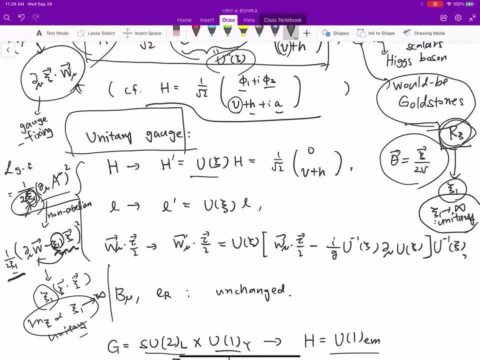 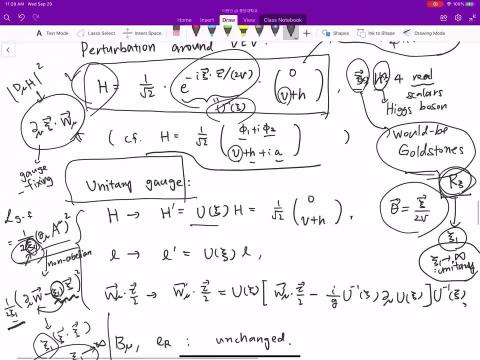 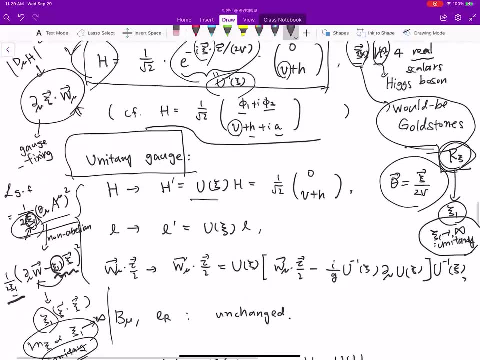 gauge. so then golden stone bosons are decoupled, then that corresponds to setting this xi equal to zero from the beginning. that that's precise, and you can. if you don't like the polar coordinate representation, you can choose this cartesian coordinate and then you can introduce the. 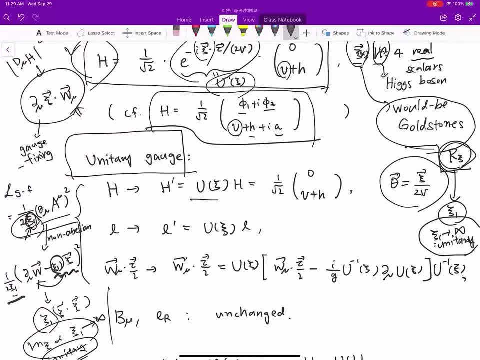 gauge fixing parameter appropriately, then you can cancel the mixing for golden stone boson. and at the expense of eliminating the mixing, you are introducing the masses for golden stone bosons and the golden stone boson can be- uh, can be infinite. then you can eliminate all the all this uh. 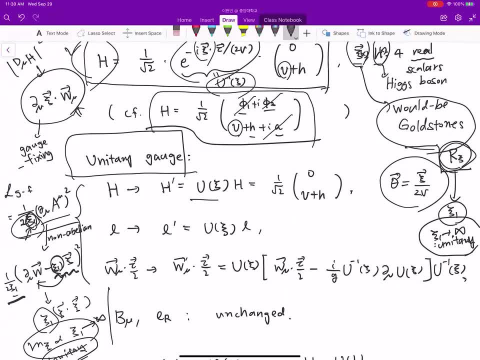 heavy degree of freedom. and then you are going to the unitary gauge. so it's basically independent, so it's a, it is the gauge fixing condition that tells you, uh, whether the golden stone bosons are kept or not. but there is independent, even if you don't cap, you don't keep the good thought modules, just to, i think, just to, you need. 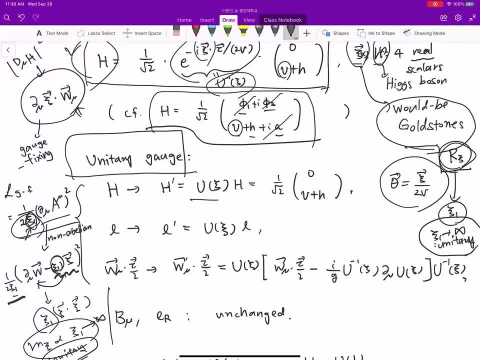 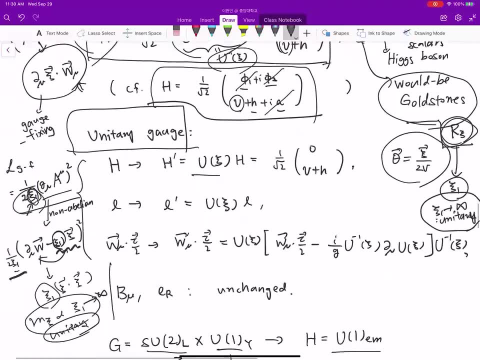 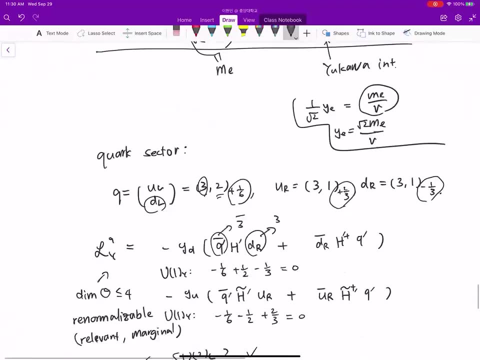 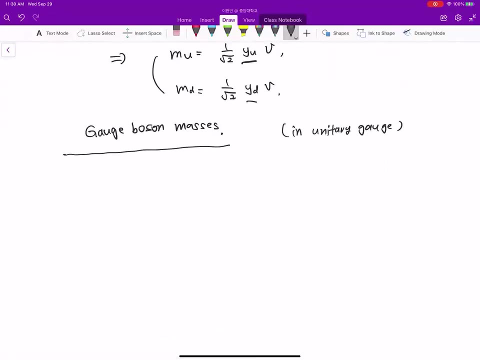 to consider. um, all those stone interactions too in the five-man diagram- uh, i'd like to finish here- are more complicated, but there is also issue with the unitary gauge. so, but okay, it's interesting issue in crafting. so gauge water masses comes from the covariant derivative term, so Higgs. 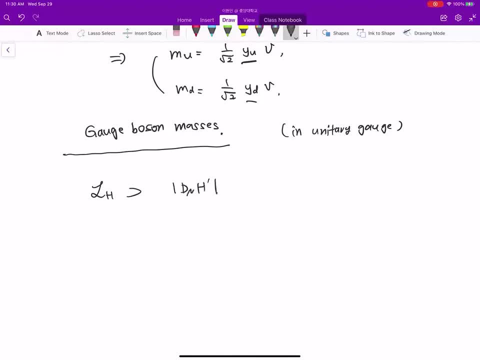 Lagrangian contains covariant derivative and unitary gauge, H, prime and this, so W boson primed right in the unitary gauge because we transform the gauge transformation. but let me drop the prime before, just for the convenience. this prime gauge boson contains longitudinal component, so it is different from 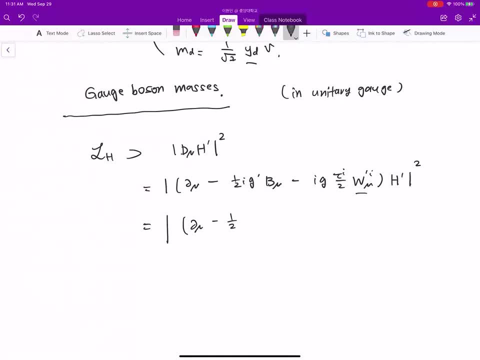 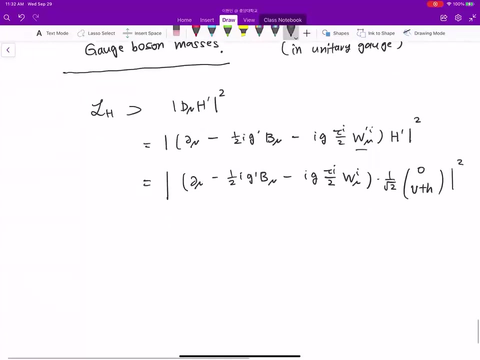 unprime gauge field. but for just convenience let me drop it. drop the prime and H prime is now between this one and then. if you expand that because this Higgs field is real, so this quadratic term gets simpler, it's a simple form, so just the derivative. when derivative act on the Higgs field, you have only connected term for Higgs. 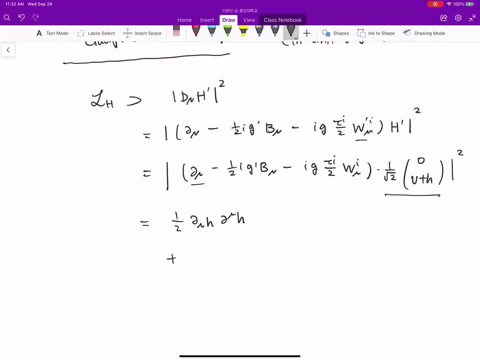 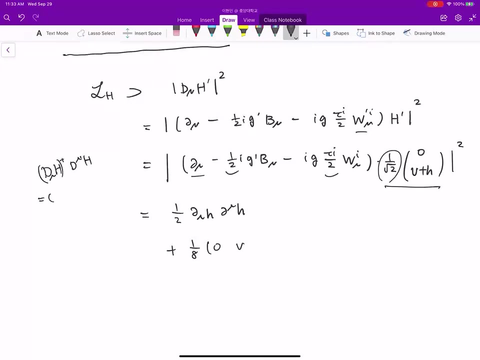 boson and we have a square and one over one one half factor. here we have a one half factor, another one half factor from after square we have a one eighth in front of it, and this is the matrix multiplication. so d H, mu d H, right, so this country, so this data. 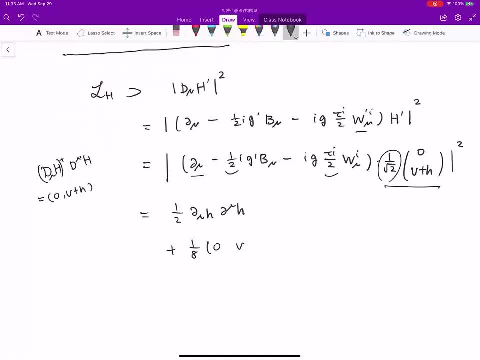 and then and then also, and also other other things also. take the country and also I'll do it- that data H prime. so in this way, right. so because this so absolute square means in matrix multiplication in this form. so because of that you need to calculate this. 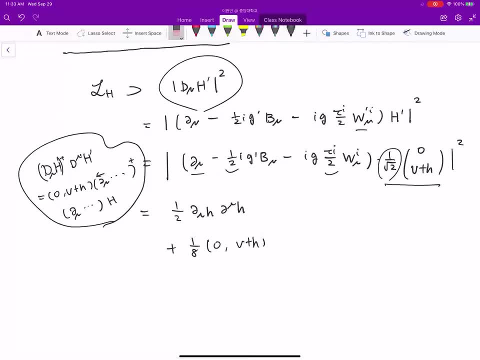 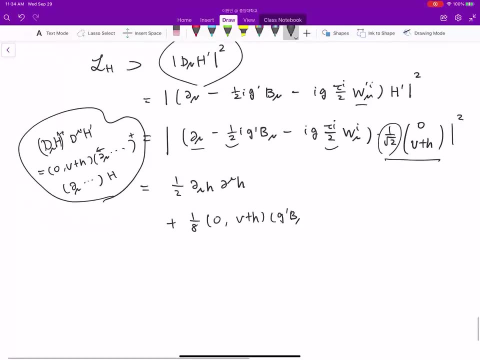 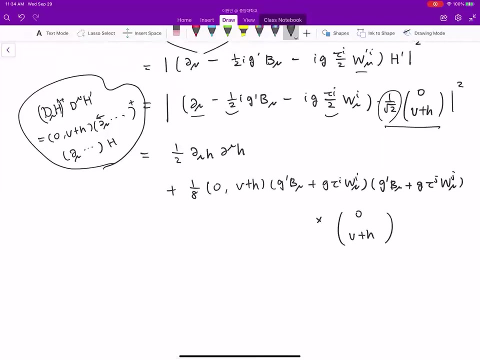 and then to to consider write down the extra term in this form, and these are g tau i and g prime, mu tau j. Let me introduce another summation index for SU times. so only these two. And then the second term contains everything for the gauge versions. So if you have one more, 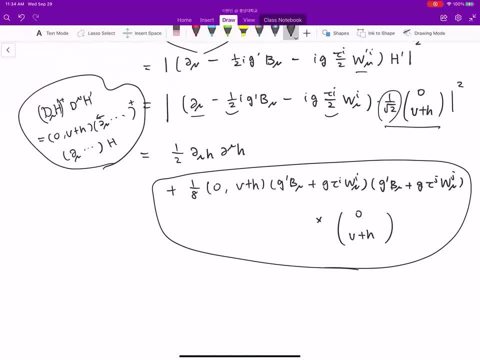 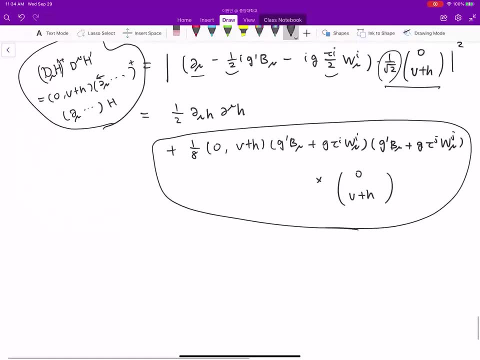 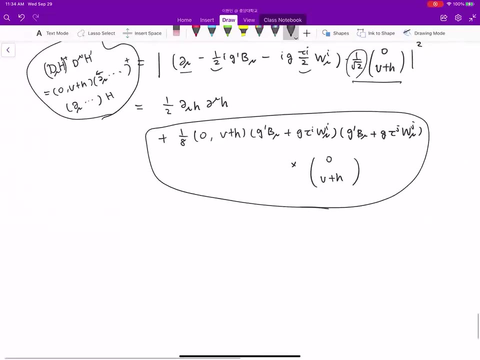 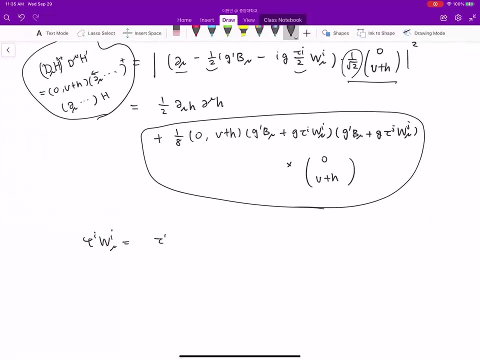 Higgs doublet. you need to do the same similar calculation. Then you will change electroweak gauge for the masses. if you have an extra scalar, extra Higgs doublet. Let me expand the SU part. Let's see the part. Let's return this one right, Tau two and then. 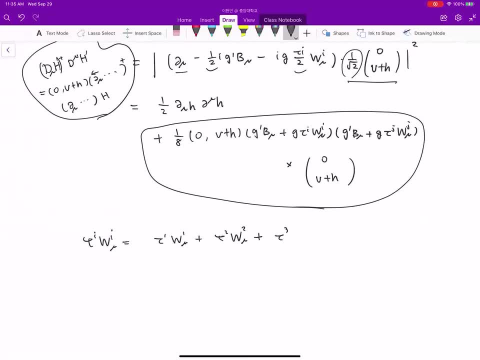 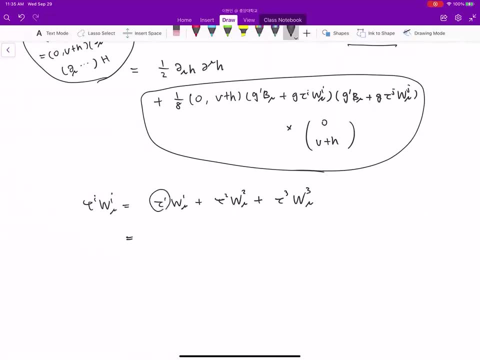 tau three, So it's the Pauli matrix, this, this, this right. So the first two, zero, and this just changing Contribute, contributing to the diagonal component W. Then here the off-dial component, the sum of the real gauge field- we call this plus charged W. 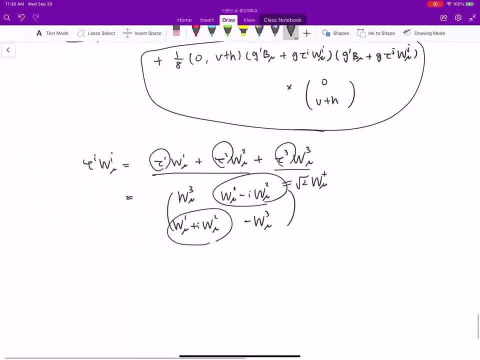 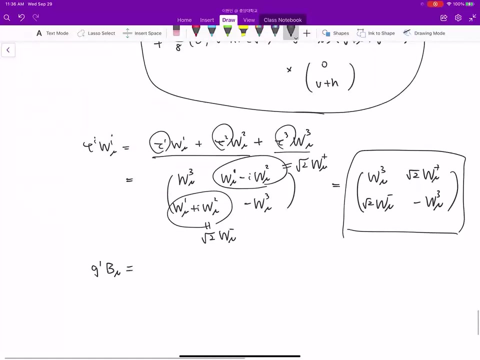 W And the other off-diagonal component is the minus negatively charged W. So we are able to write down- Let's do the part in this- two by two, matrix form And G prime, the hypercharged part. as I said, there is an identity, two by two identity, So just G prime Because the hypercharge 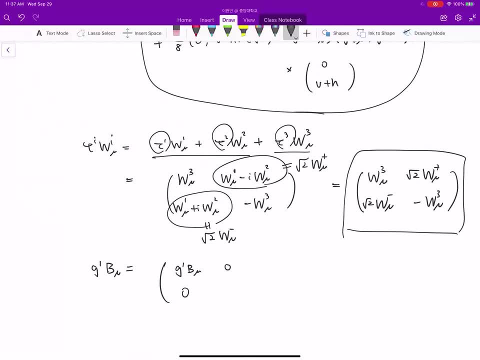 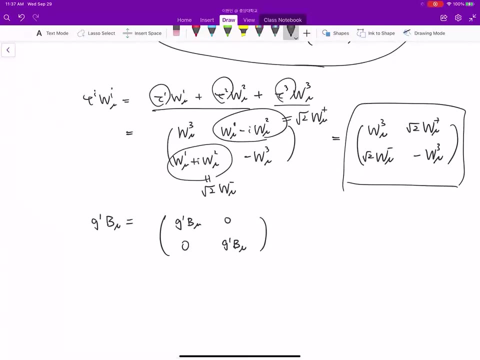 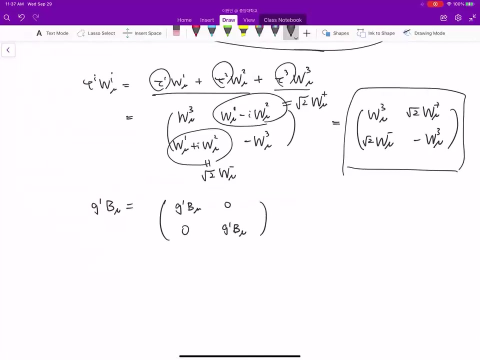 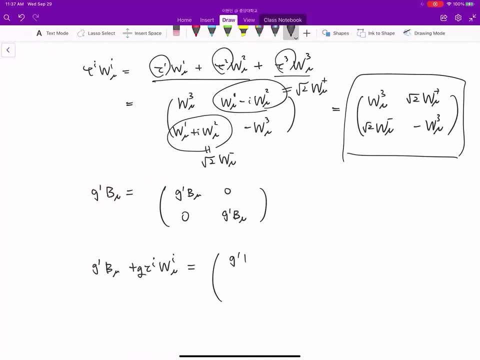 down, up and down. I mean in the doublet you have the same hypercharge for up and down. So You can write down this in this matrix form: Just the sum of them, Then just the sum. So we have a gauge coupling, sorry, G SU, two, SU, two, gauge coupling in front of G prime. 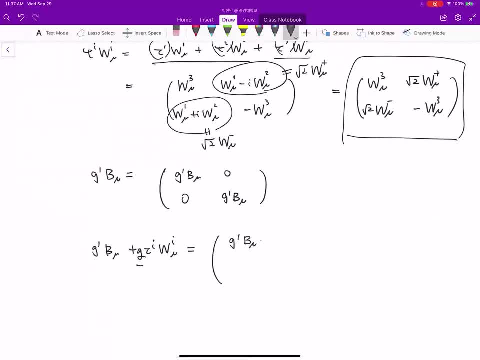 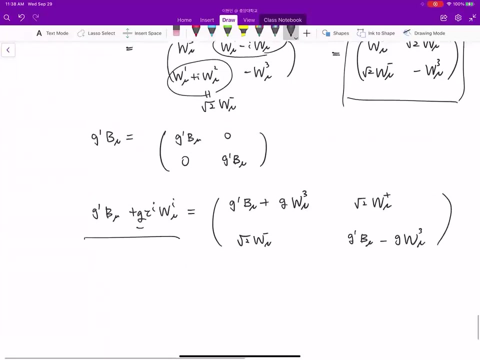 The gauge coupling in front of it. So in this simple form, So matrix form. So, because of that, this, this, these, there are more. so, because of that this, there is of course one, Dadelli, Isn't it? 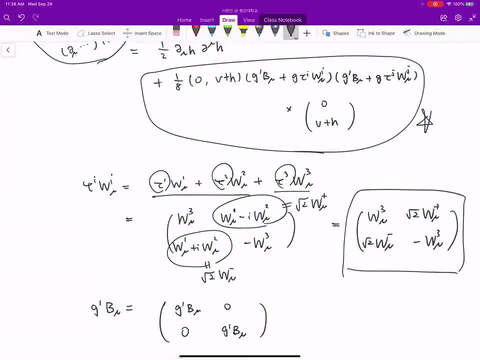 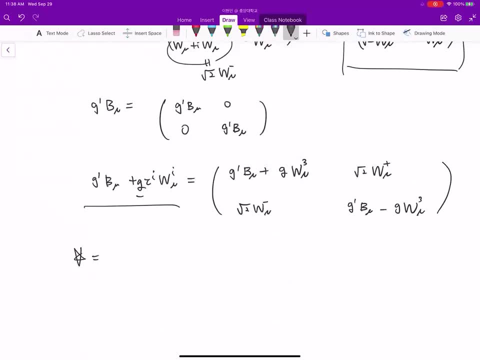 the star term. second term can be written expressly: so: zeta term. sorry, this is star term. so one-eighths and the square of this, the square of this one. instead of taking the square, we know that we have same term appearing twice. 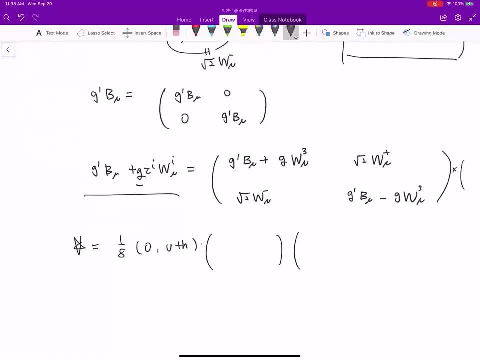 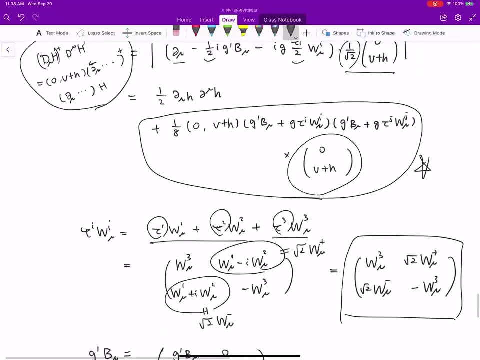 but here this one will be multiplied to this one right, And this this here. So I don't want to do this square. instead I do this one and this is just conjugate, the transpose right. This is the transpose. this is, let's say, this is the psi, then this is the psi. 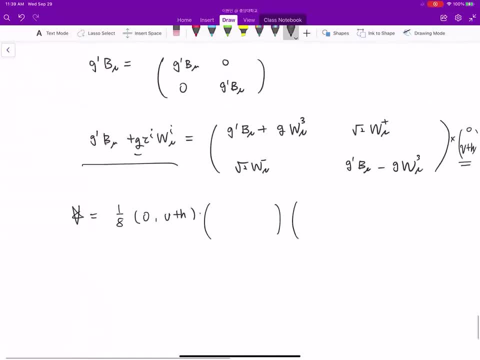 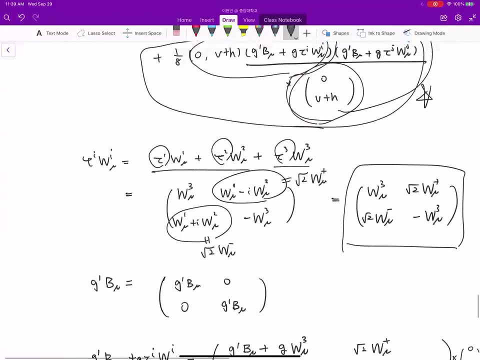 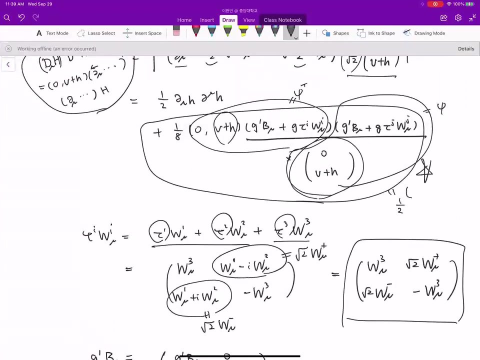 So then, this is psi and the psi. this one is psi, So psi is the and this is psi, equal to two. but by the way, this, actually you can write down, this one, let me call, let me call this psi. 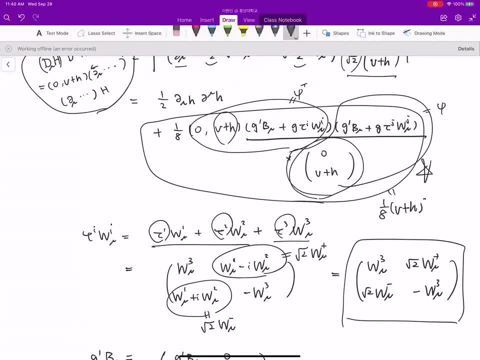 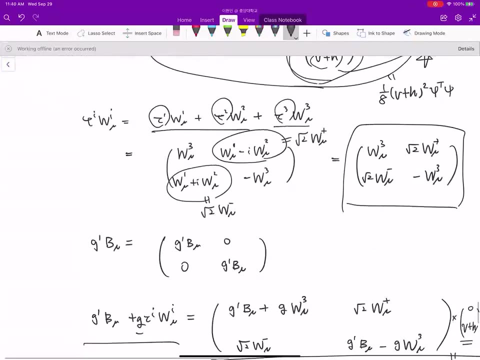 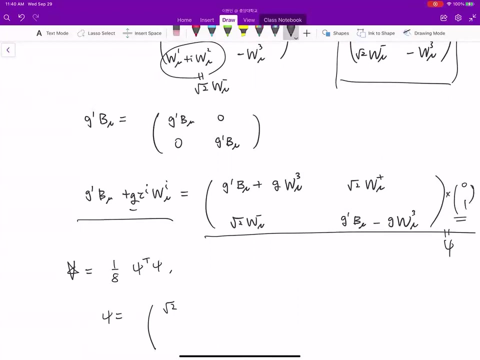 one-eighths v h square psi. okay, So psi does not contain this v of three plus h. so because it will, it will be factorized. it's over factor. okay, Zero, zero comma one for the column vector. 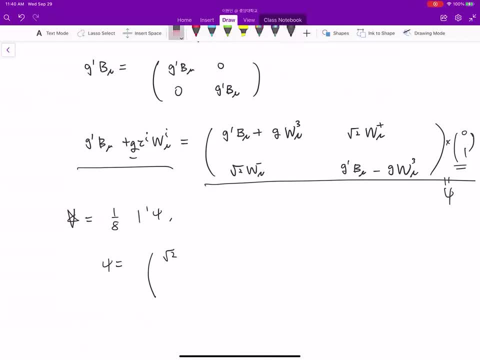 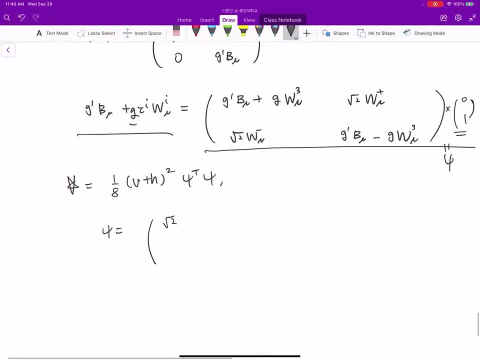 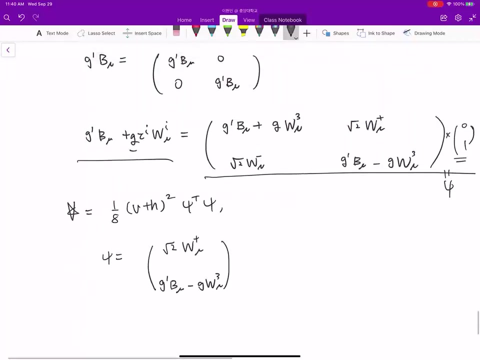 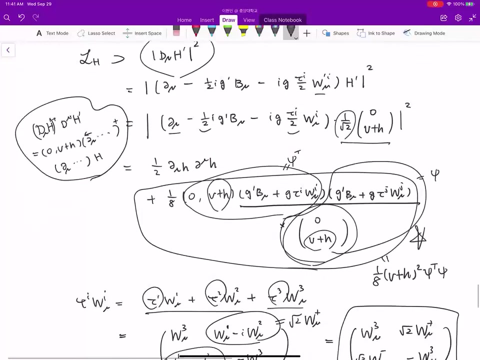 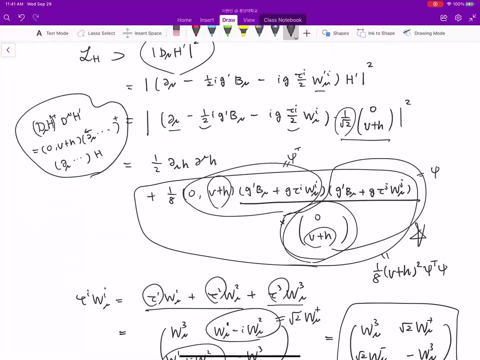 So so then, after matrix multiplication, you will see you have this one. probably you may have, let's say, you have this one. sorry, you might have this one, this one, this one and this one. 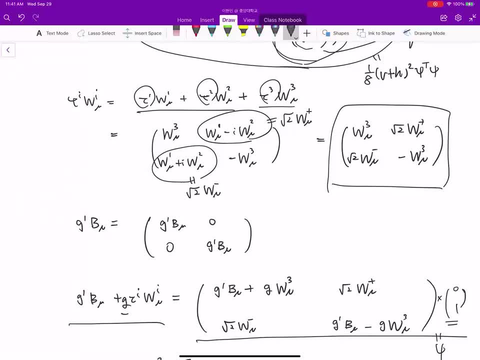 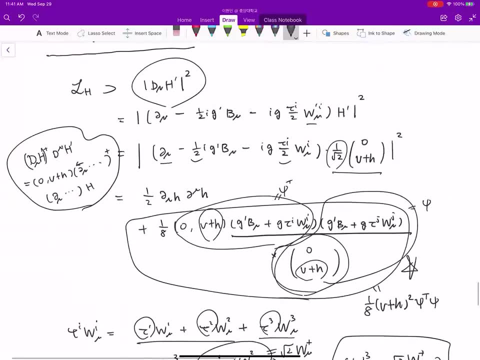 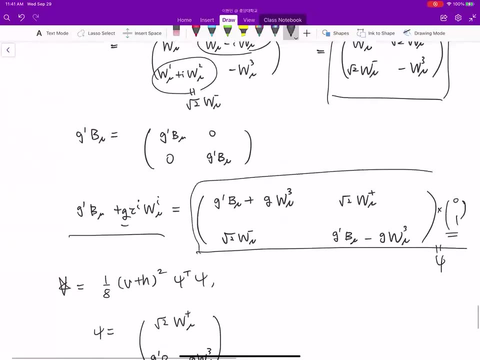 and this one, like you see the integration, not like this one and this one, this one, right, they're not also related, you know so so so so this, this is not the real uh matrix, because this we have a plus and minus, so it is different. 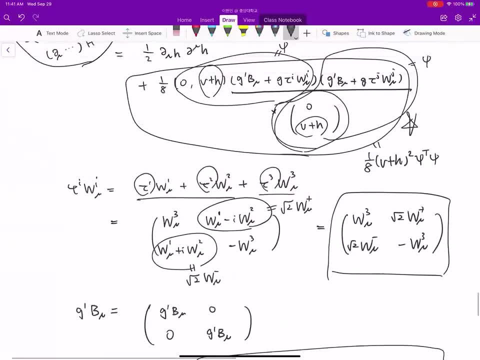 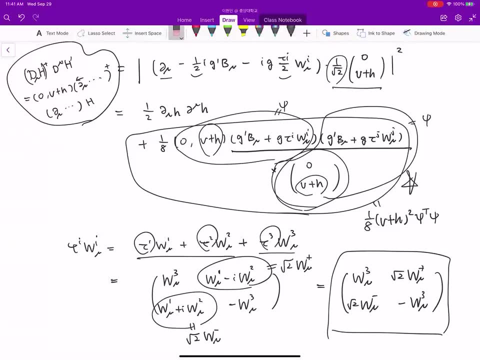 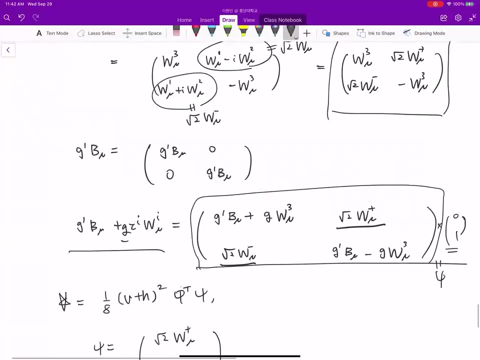 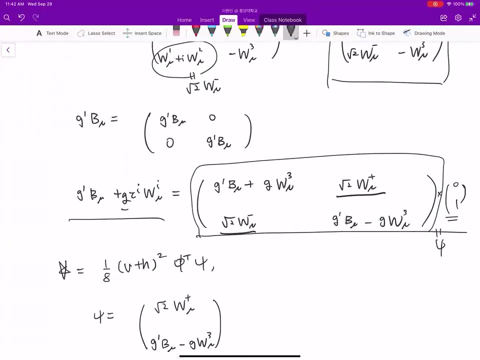 different one, sorry. so, psi, yeah, we have to. yeah, this is not exactly this one, but i don't know how to go. i don't know how to call this. it's not the same, sorry. in any case, you can multiply. there's another combination, another, another term, another factor. with this combination, multiply by zero comma one, right. 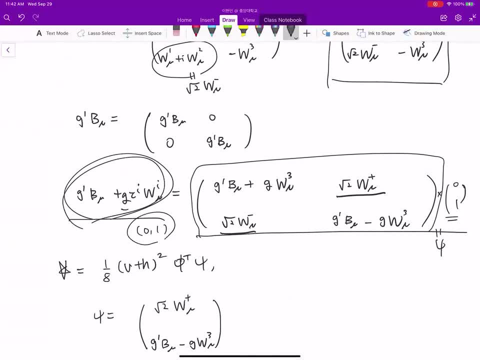 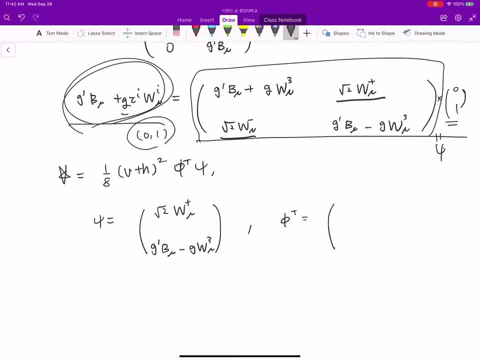 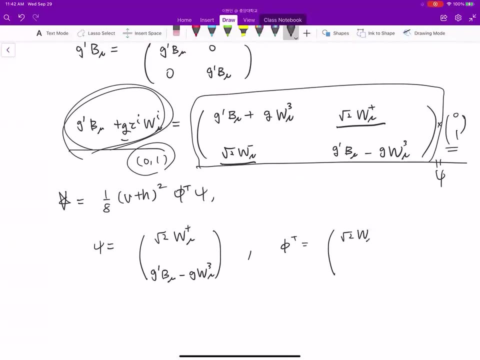 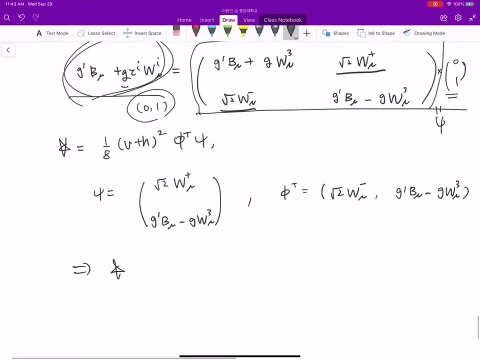 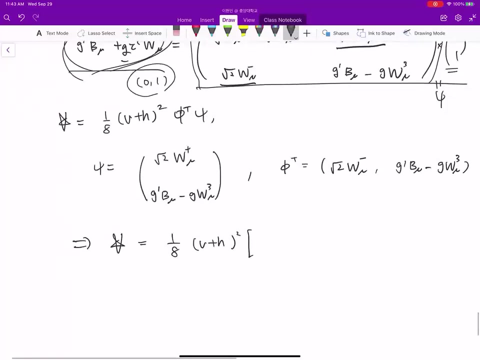 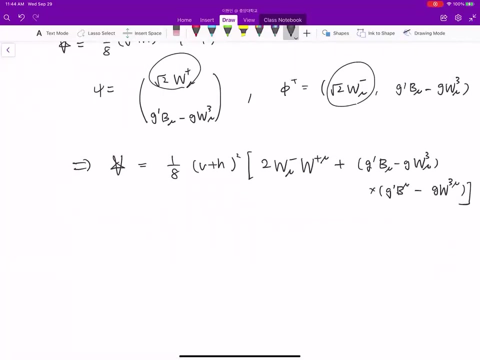 so this is the one that we have to do that and just to no, no, yes, okay, then star. so this product of this and this one is, um, yeah, yeah, Yes. so you have several terms appearing here. the second term: you have a mixing. yes, mixing. 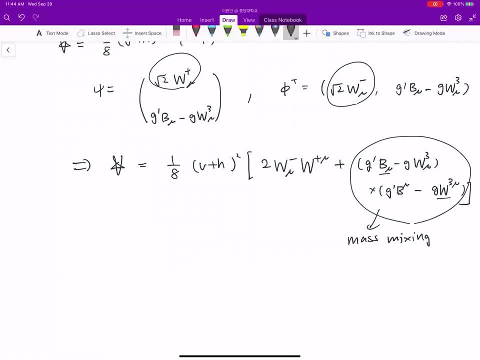 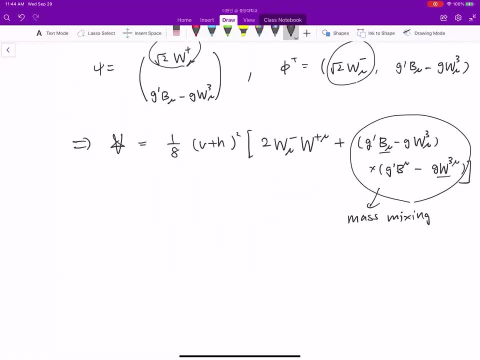 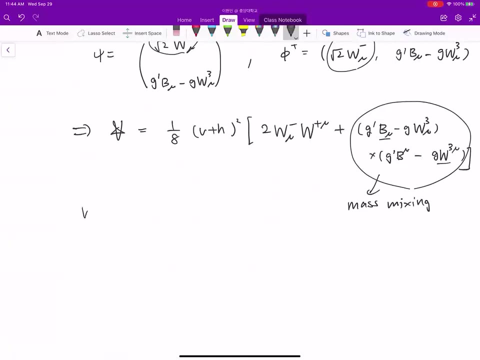 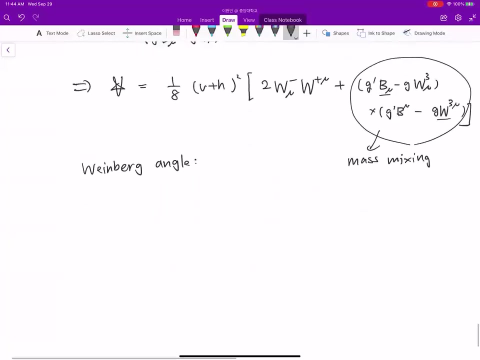 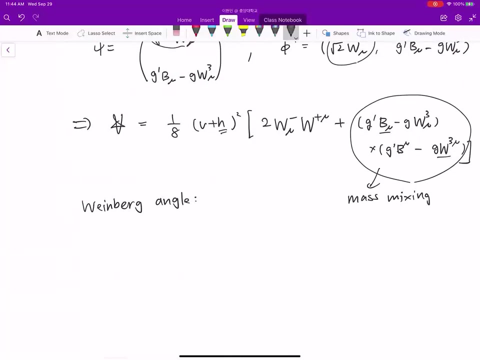 because of B mu, W mu, W3 mu. they are mixing, so we need to diagonalize this neutral gauge version. In order to do that, we introduce Weinberg-Anchor. So these are mass terms. when you ignore the Higgs version, this corresponds to mass term. 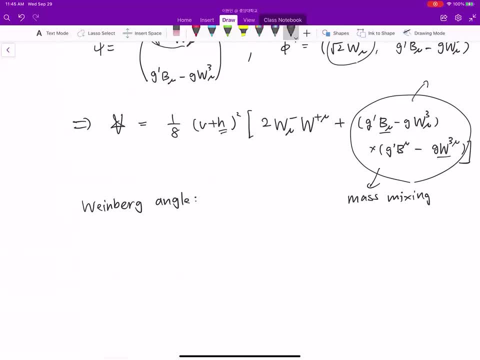 for neutral gauge version. So this should be diagonalized and you have a G-version mass after diagonalizing. So because this combination must be G, G-version must be proportional to in this particular combination And there must be orthogonal to that. the orthogonal combination must be photon orthogonal. 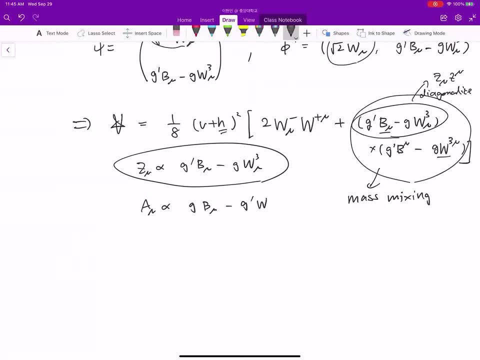 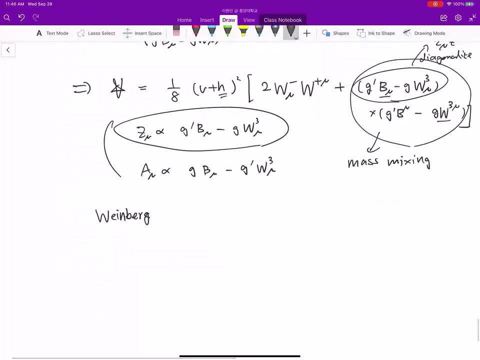 combination must be something like this: And then you need to normalize- if it is orthogonal transformation appropriately you need to normalize this transformation. That's how you obtain the Weinberg-Anchor. So Weinberg-Anchor, the standard notation. there's some sign difference of two sign difference. 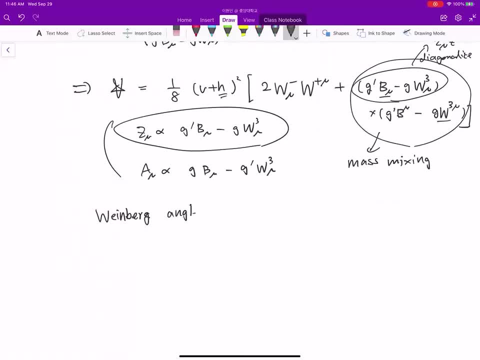 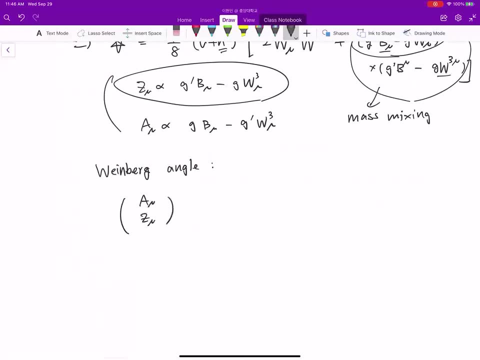 but it doesn't matter much. So photon and flexon, this is the problem. and now, if you remove this, this is the problem. Yes, This is the problem, Right? Yes, hypercharge and the neutral component of the electroweak gauge version. 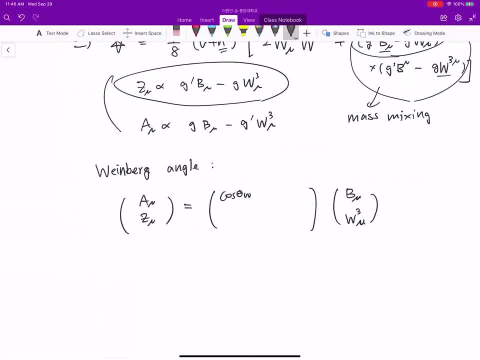 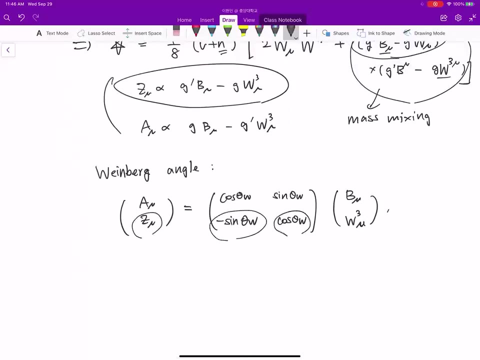 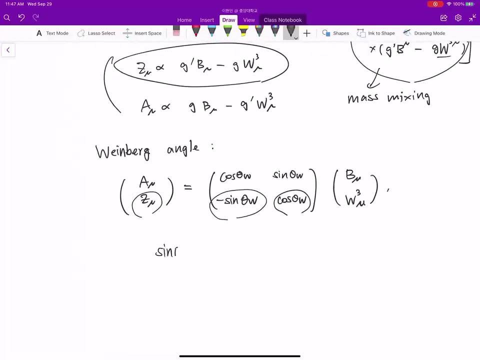 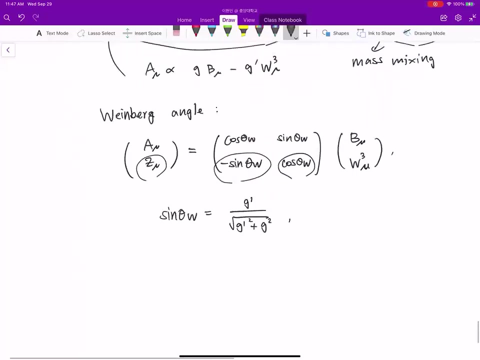 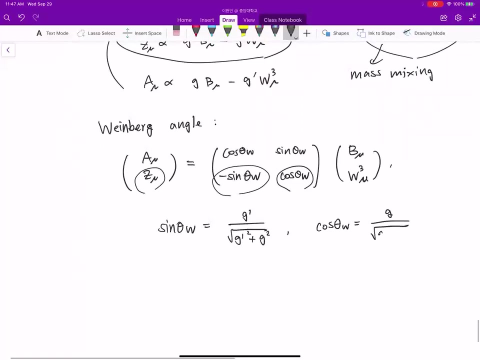 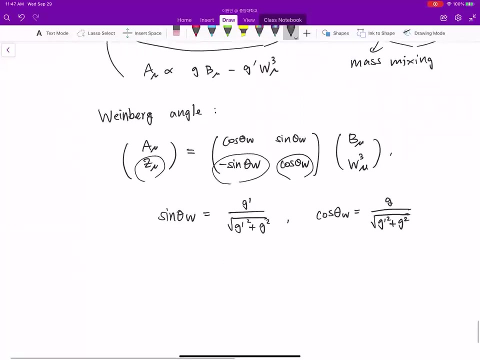 okay, so this is cosine, this one, and here you see the. the g version contains it here, b minus w, something like that, so you can identify the weinberg angle. normalized this one and then cosine, oops g this way. so i think the in this way, uh. 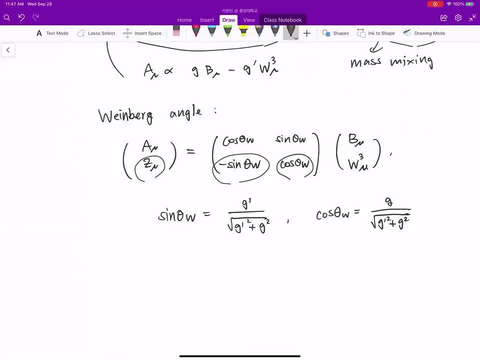 uh, i think the at the weinberg angle kind of mix mixture kind of determines the mixture of neutral gauge versions. and if weinberg angle equal to zero, then weinberg angle equal to zero, then the photon is just given by, would be given by this hypercharge only and uh, g version would be given. 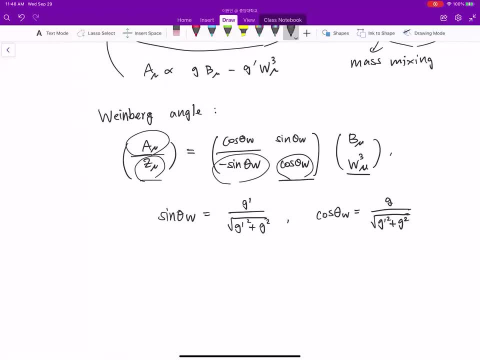 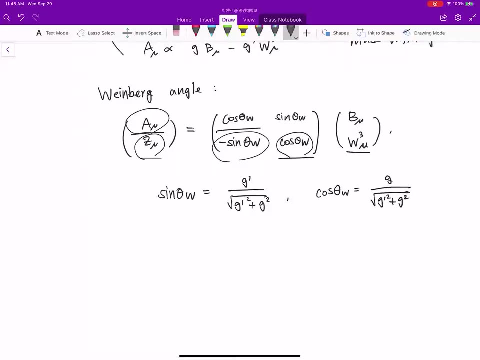 by uh neutral component of the sd PHT gauge versions, but in nature. in nature is why mowan angle is different, fromavored so, and then it has been measured precisely so. basically, that is theẽs how we normally measure. w Because of that, this combination appearing in the mass term can be written down in this: 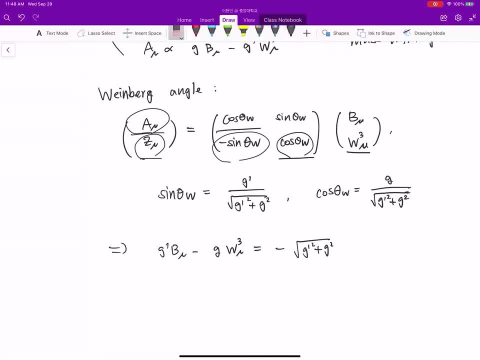 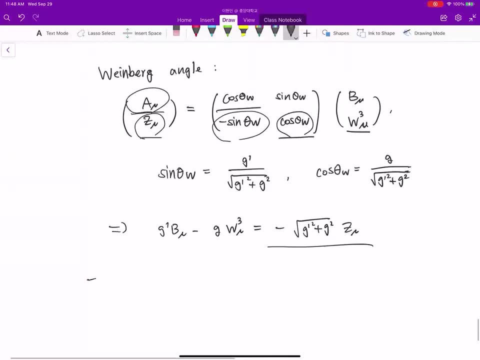 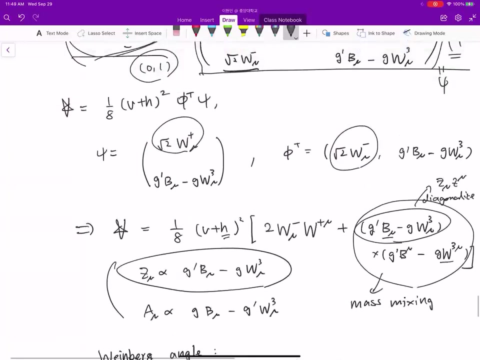 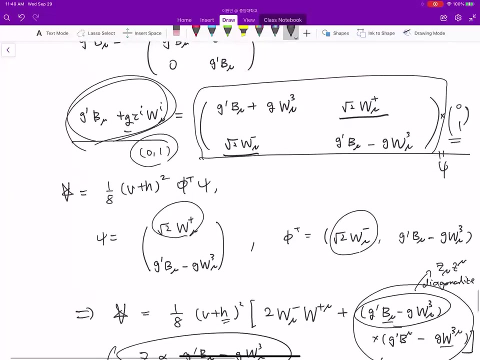 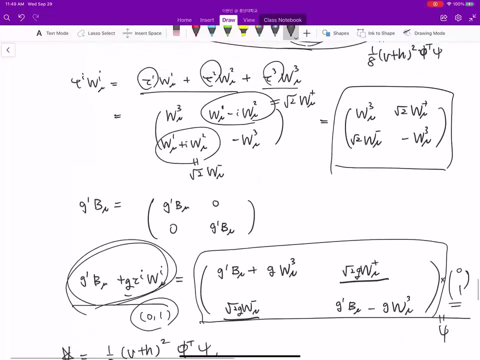 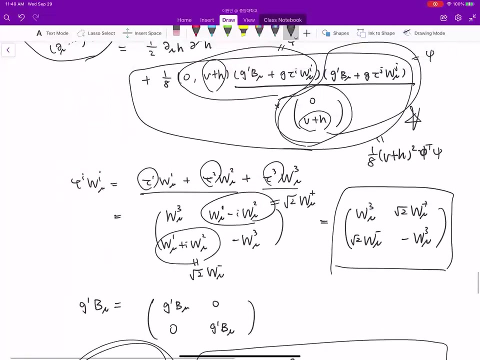 form, only the g-version, And the photon doesn't appear because of that. Maybe there's some. I forgot something. Is there any? Oh, I forgot the g-coupling here, g. Here we need to multiply the g-coupling, here, g. 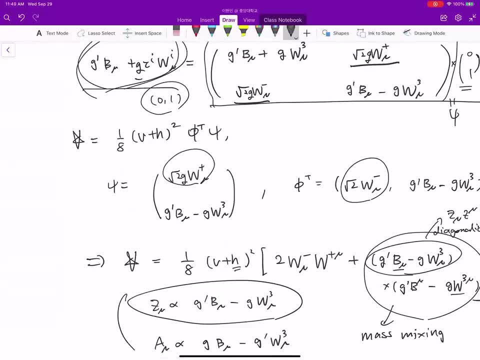 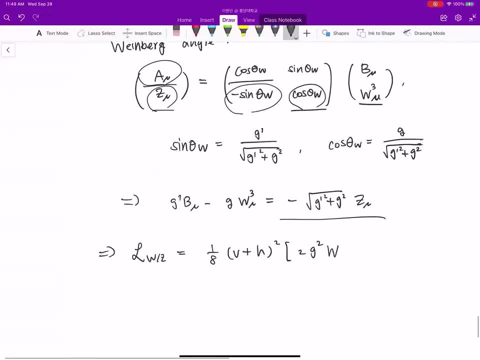 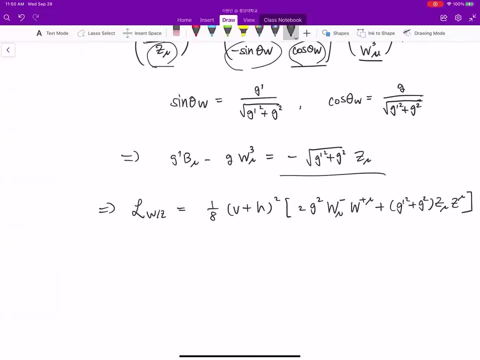 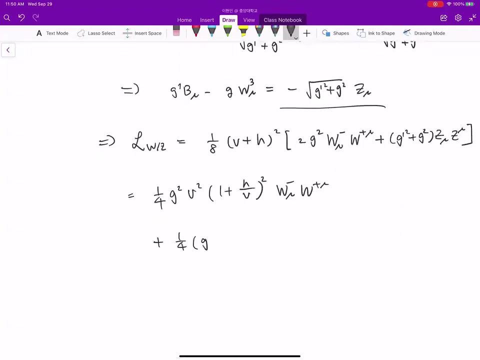 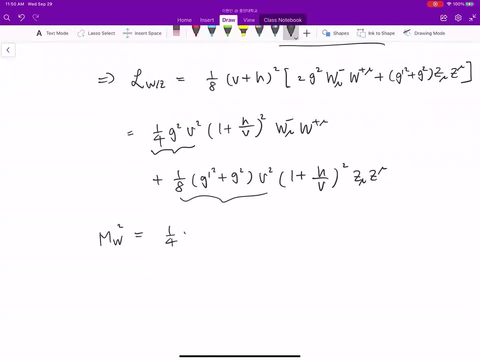 Also here g. Okay, So we have fully diagonalized the electroweak g-version and this is the. then we can rewrite this form This way. So the coefficient identified, Okay, with the gauge boson masses. So w boson mass is square equal to this one, because this is: 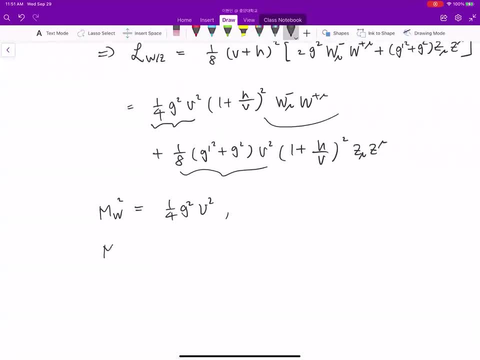 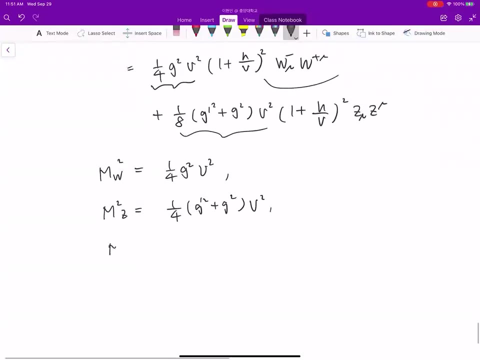 complex field and g boson mass is also this way, And then the photon mass is equal to the photon mass. So we can explain the difference between weak force and this is the electron magnetic force. It's a long range And it's a short range. Before that, all the gauge 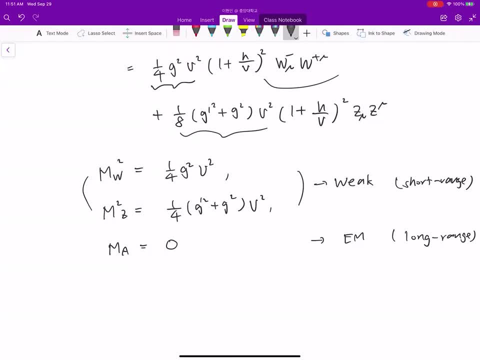 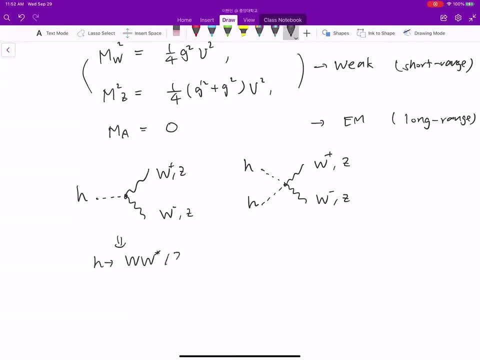 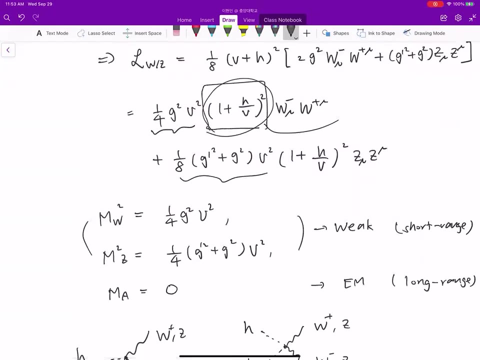 gauge boson masses are massive, All the gauge boson masses are massive, All the to wwwdjstop. And the important thing is that the Higgs appears in this particular form. So in general you can parameterize this like a 1 plus 2. 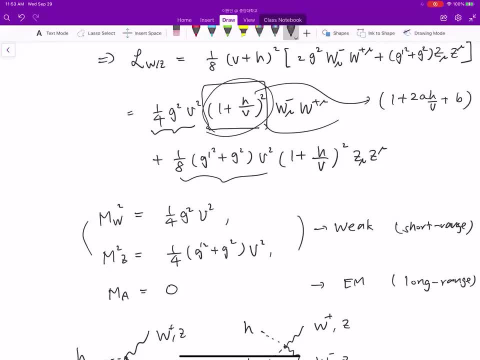 a, 2, b plus b: The standard model. you can compare whether this is the standard Higgs or not. If a equal to b, equal to 1, then this is the standard model, But if different from that, then it is not the standard model. 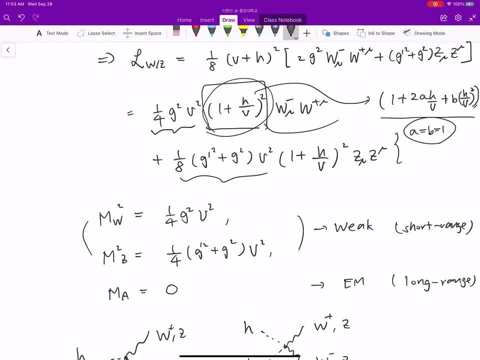 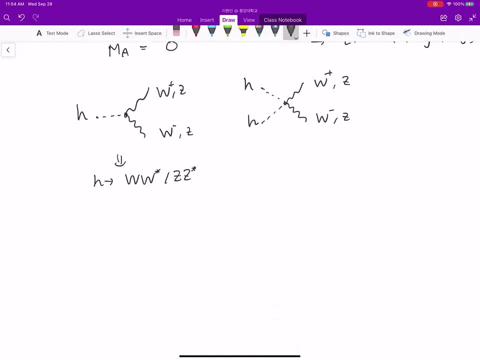 And also- so this is Higgs measurement, and also unitarity. Unitarity: it is important to satisfy this condition. Unitarity- Maybe this is not quantum QFT course, so I don't know, So you can just let me mention it- And also Higgs interaction, Higgs potential. 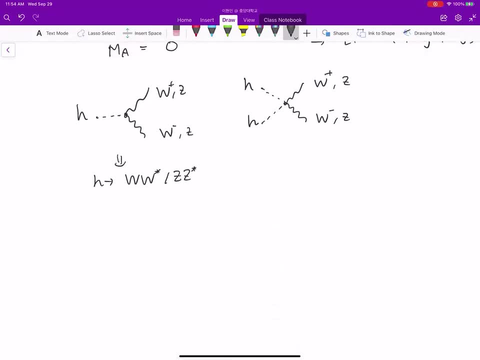 you can also also identify Hq- H40 interaction. So maybe just let me skip over to different discussion, because this is not that difficult to identify. So neutral current and charged current interactions. So first, neutral current, neutral current interaction. Let me focus on leptons, and that can be easily. 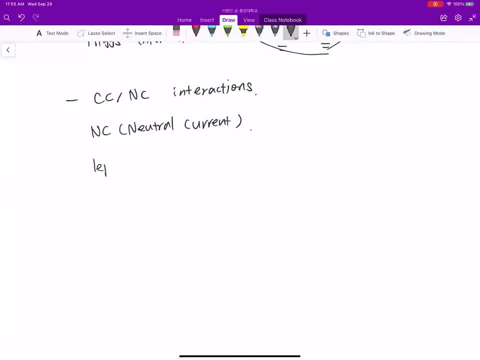 generalized to the case of quarks. So we have from the covariant derivative, we have covariant derivative of the spinors. we have this, this, this, this, this spinor spinors. we have this interaction to gauge field for the lepton singlet and also lepton doublet. 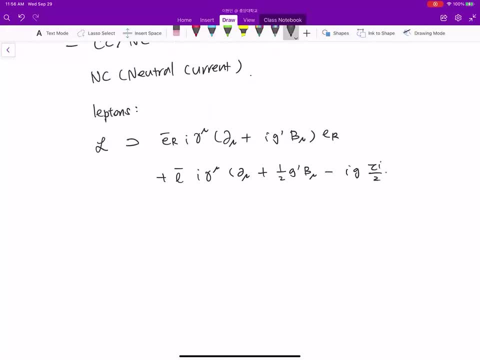 I think just we can keep track of all the interaction term. alright, then. so this? this contains both this. this term contains both neutral and charged gauge volumes. so in this, if you remember this, what was this and what was the w3, w3, w1- Iw2? 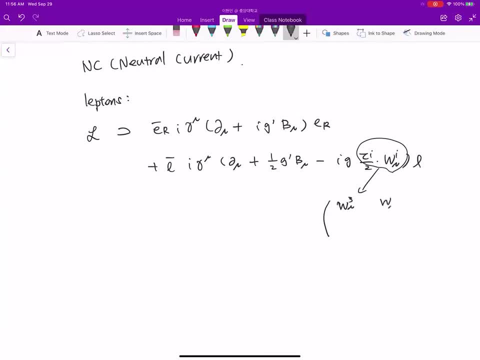 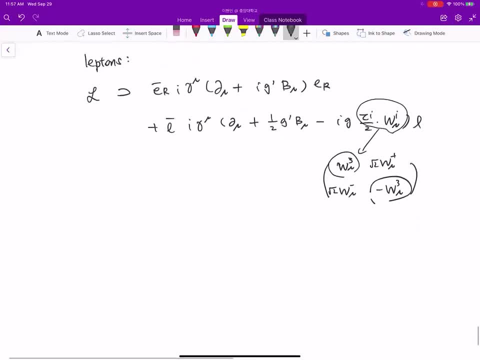 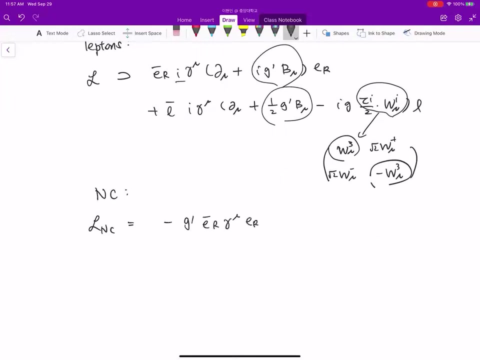 okay, so So the neutral component, we keep this hypercharge as well as neutral component of the SU gauge motions. So neutral component, therefore, we keep interaction only. So interaction just to expand the second term, to get the first term and the second. 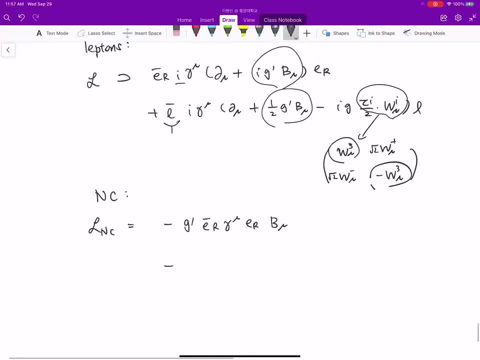 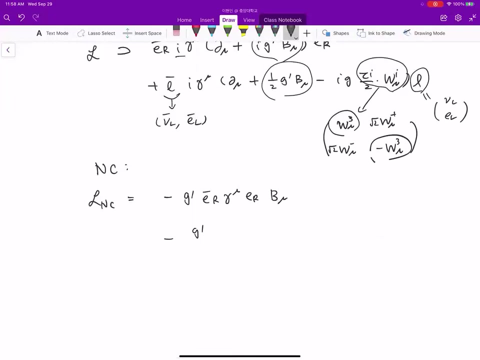 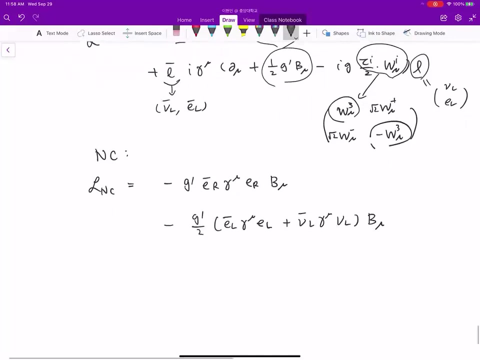 term. Second term, just you replace this by lepton doublet also this one, this one, and just expand that, Then hypercharge. hypercharge is the coupled to neutrino and electron in the same way, And W3, W3 perp plus. 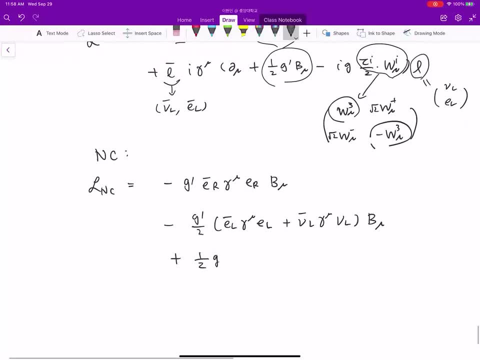 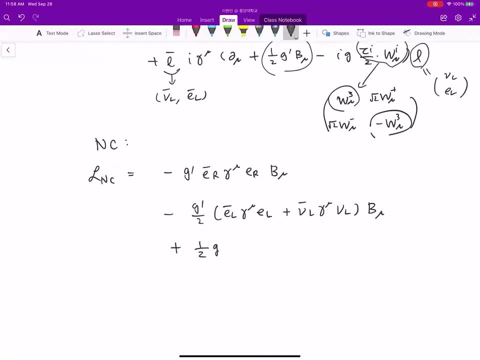 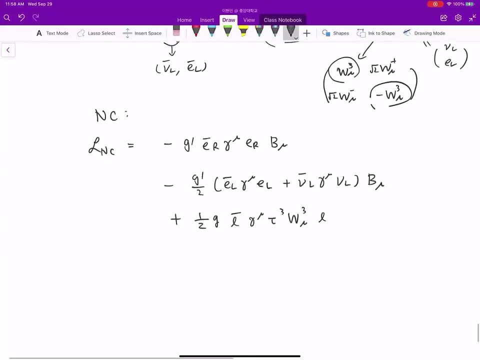 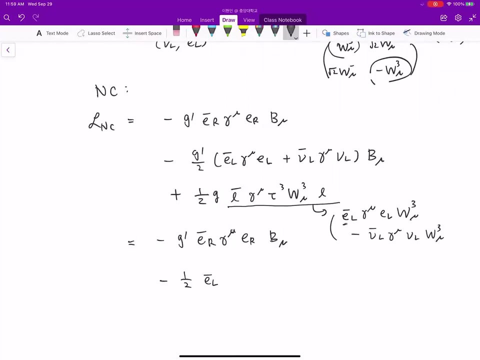 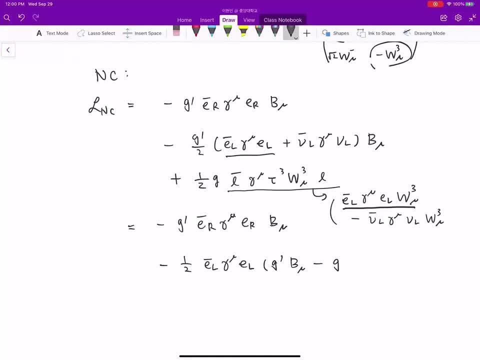 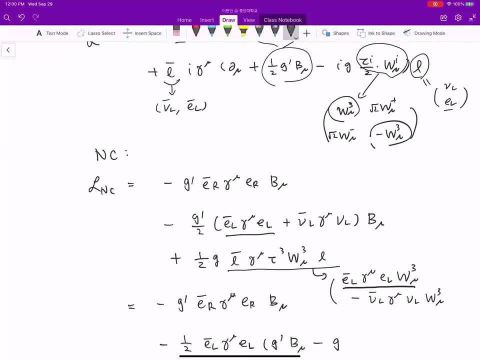 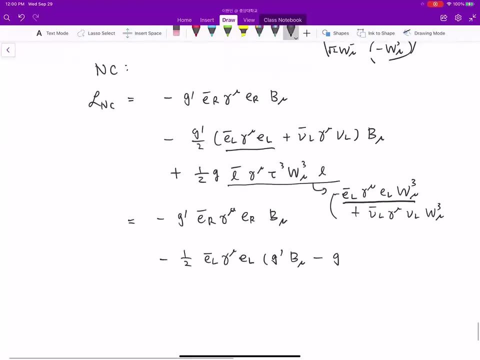 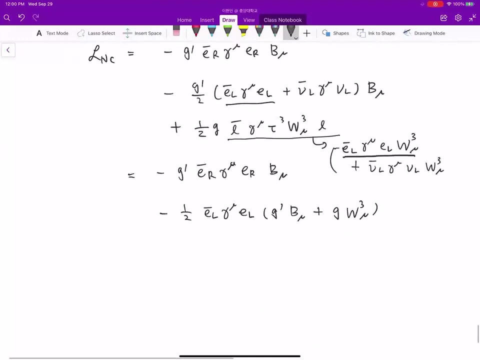 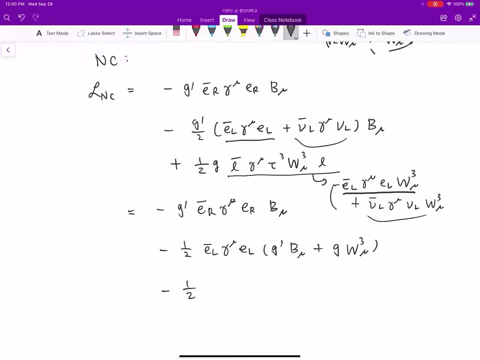 um, I don't know where was the. uh, there was some. yeah, okay, so the lepton is up, uh, is the down downstairs. so, minus the sign changes. so this one plus g, okay, and that's and neutrino. we have a neutrino, also another neutrino, so 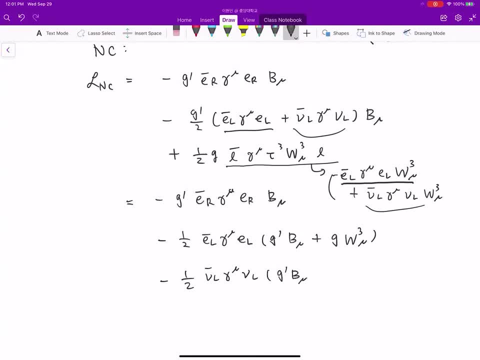 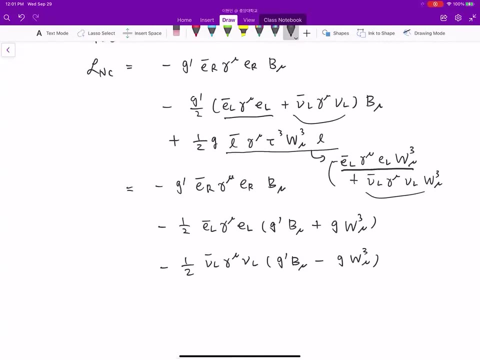 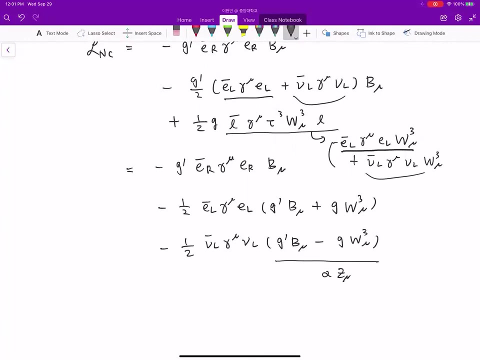 um, in this case minus. right, this is minus. I think. this is everything. so, uh then, um, so, yeah, then I think that in this combination, this is the proportional to the neutral uh g version. the neutrino does not couple to photon, but this second term contains both photon and neutral. 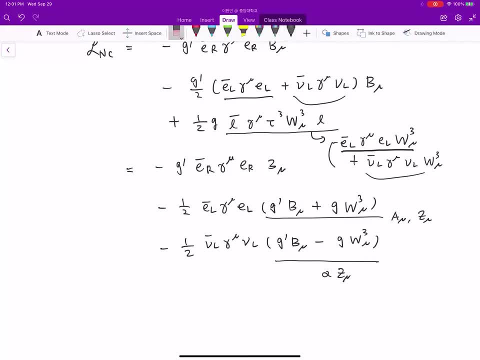 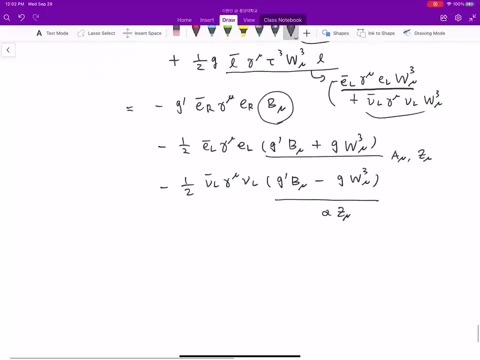 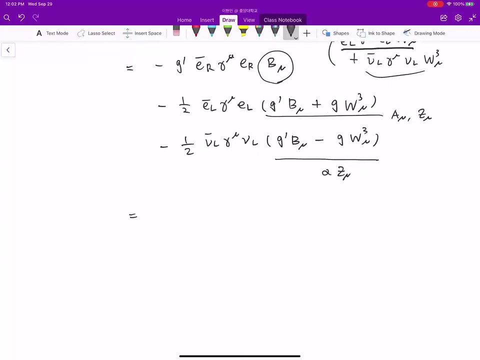 g version and also this hypercharge also contains is a linear combination. so we need to expand them and then fully carefully following the details, and i mean we need to take into account the weinberg angles. then in the end you can write down uh explicitly. it is nice to see that. 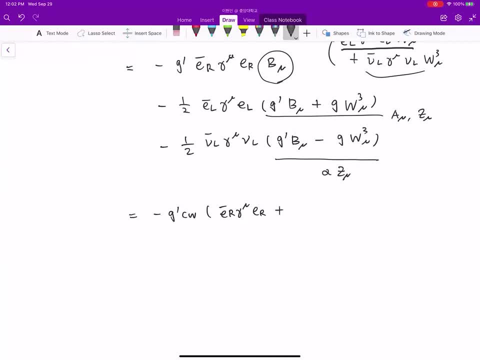 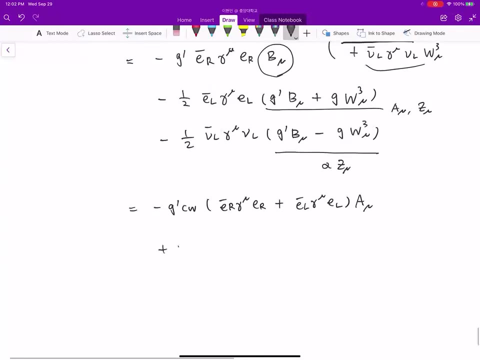 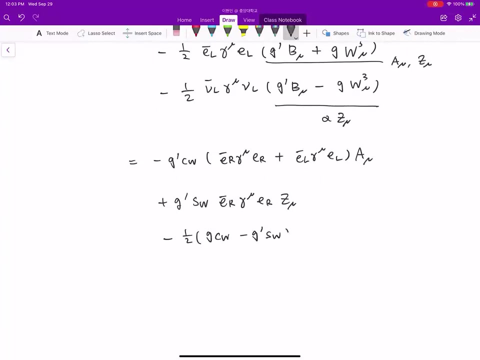 uh photon does not distinguish uh chirality. the photon couples to left-handed and right-handed in the same way and plus g and electron couples to g boson, but you see the coefficient are different, so left-handed and right-handed. so g boson distinguish the chiralities. 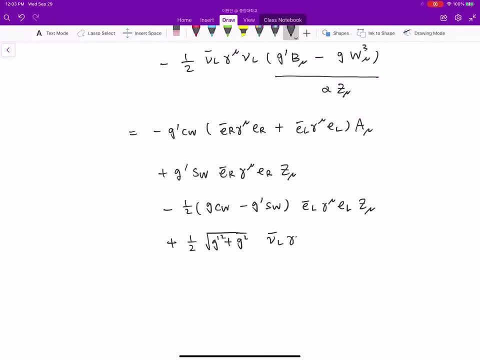 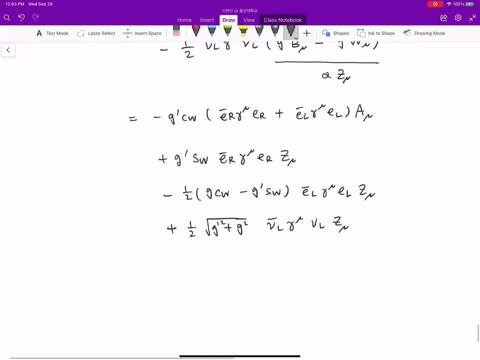 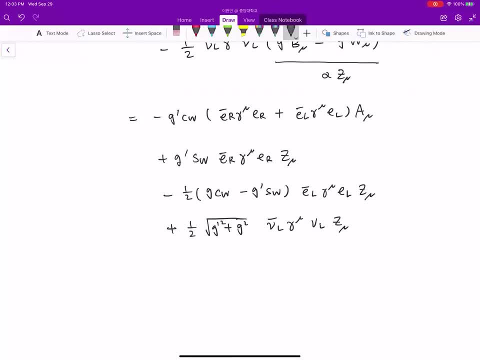 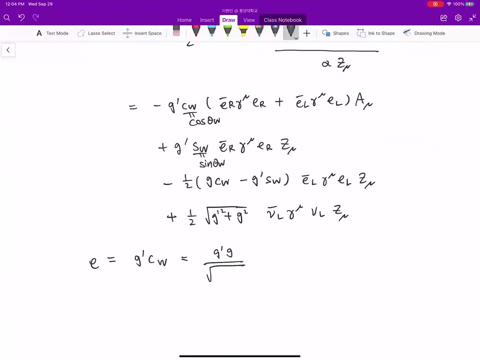 directly measured g prime, we need to change it to physical parameters. so because of that, electromonically charge is g prime sito. The CW is the shortened notation, cosine theta W. Also sine W is the sine theta W. So then you can write explicitly: G prime times CW. 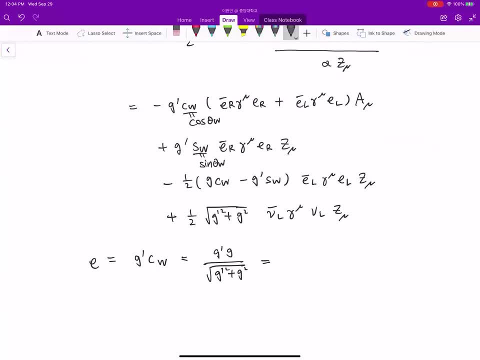 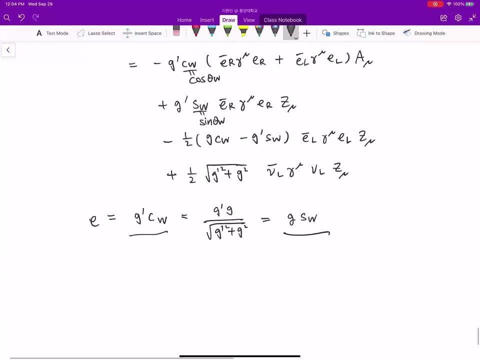 This way, then this is nothing but G times sine W. So you can either obtain electromagnetic charge from either from G prime coupling or SU coupling. Because of this sine I mean Weinberg angle. So this is the electromagnetic charge, This is the observably measurable quantity. 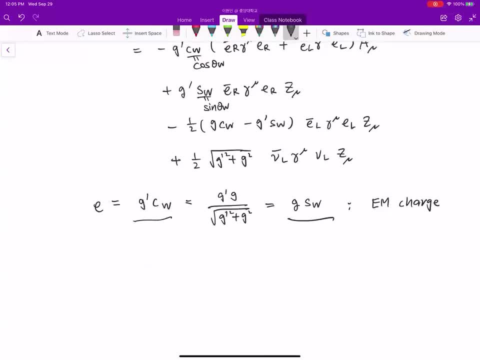 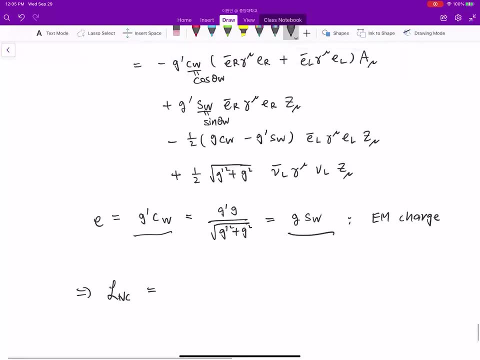 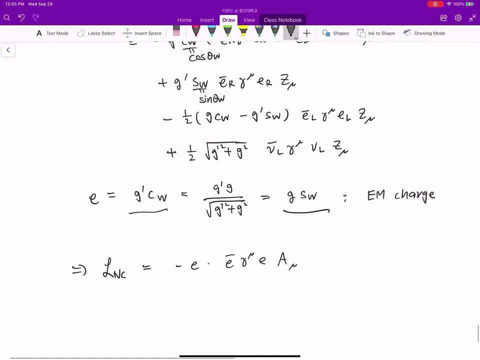 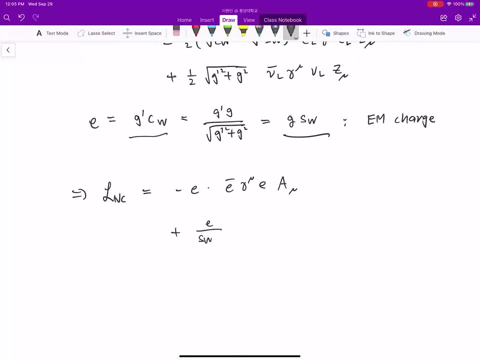 And then you can also massage the other terms and eventually neutral current turns out to be minus B. This is, I guess I still have Diskussion about the. I'm writing this in a more you know small wii知道 anything. I'm writing this in: 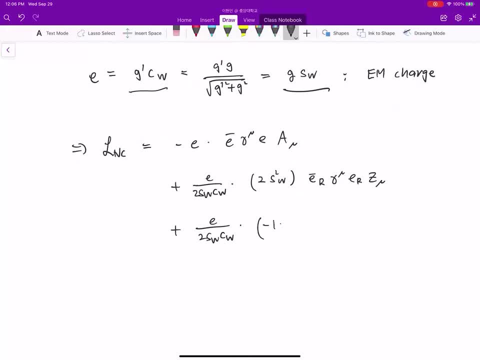 Um, I'm writing this in a more, you know, convenient notation. So these are neutral current actually, these are electromagnetic. the first term is the electromagnetic, the other three is the neutral. we call this neutral current actually, but the electromagnetic interaction also neutral in the sense that the mediator does not carry. 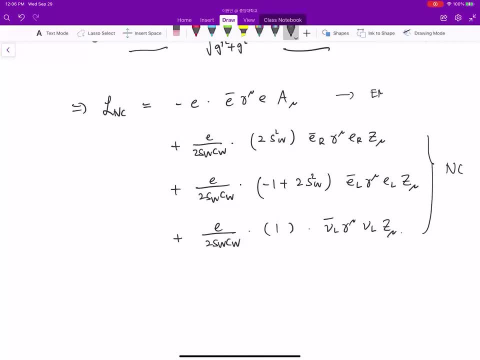 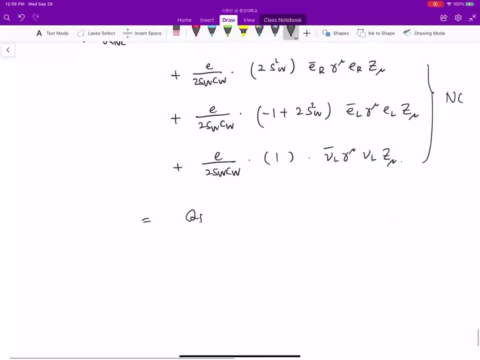 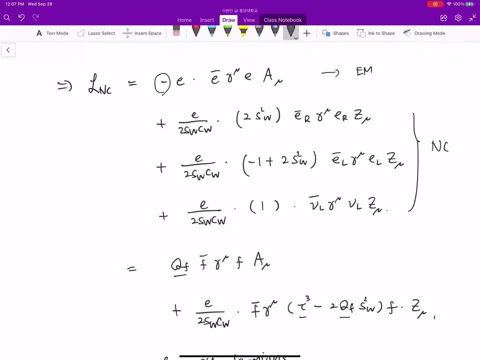 electromagnetic charge but the electromagnetic charge. Then you can write down this in a more general form. So this F run for the standard model, All the standard model formulas. The interaction term depends on this tau and electromagnetic charge. So the electromagnetic charge for electron, as you can see here, minus one right. 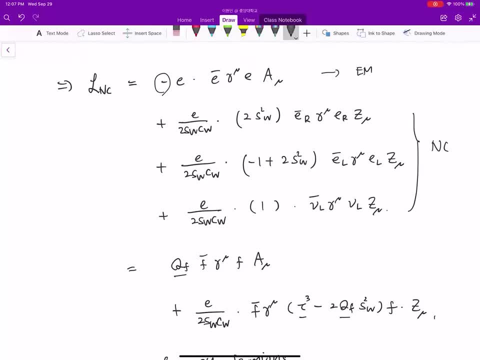 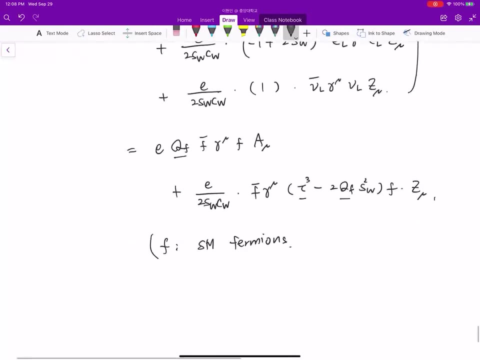 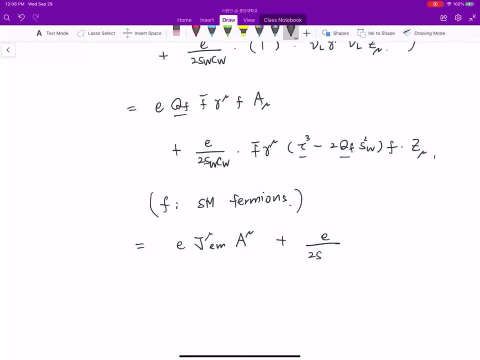 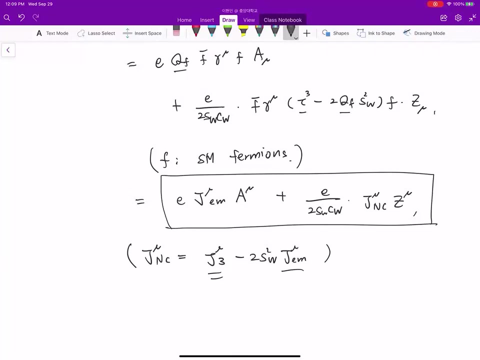 Plus, Not rule contour. Well, And this neutral current can be written as the third component of SU current and the electromagnetic current. So this is a simple form of the neutral current interaction in terms of the current. And here tau three is the Pauli matrix, one with one minus one in the diagonal entries. 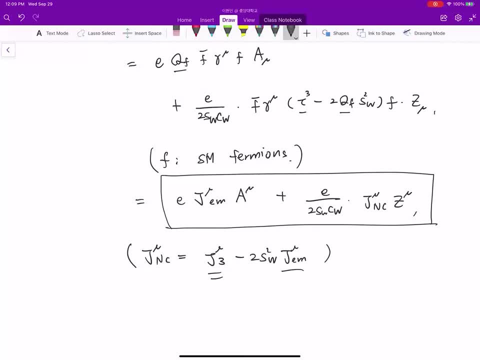 So tau three is non-zero only if F is doubly SU two doubly. If F is a singlet, tau three equal to zero. So if F equal to tau, okay. So lepton doubly: neutrino for neutrino plus one for electron, minus one. this way: 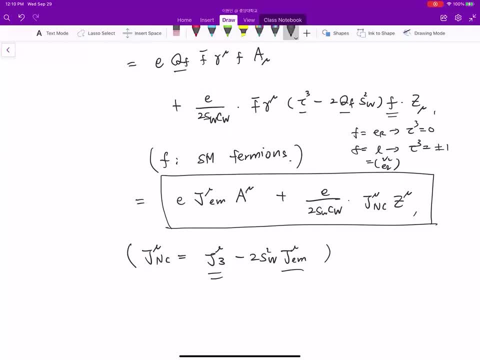 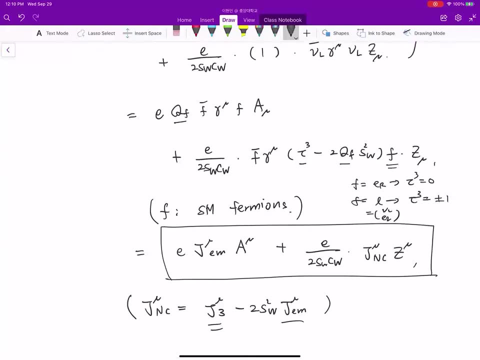 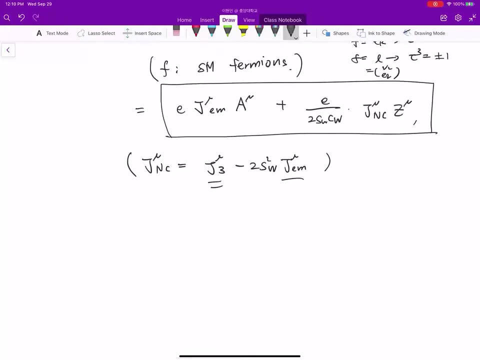 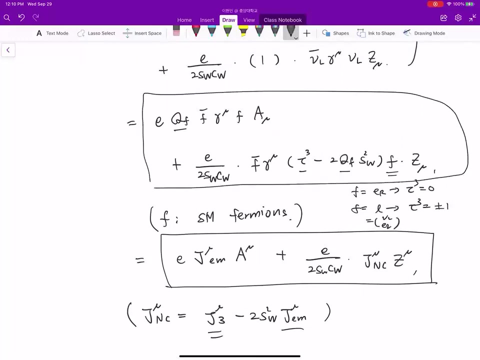 Then you can accommodate all the not only leptons but also quarks, So all F who can be leptonal, quarks or leptons. I think that there are several. I think that this is more. you need to count. what is the? 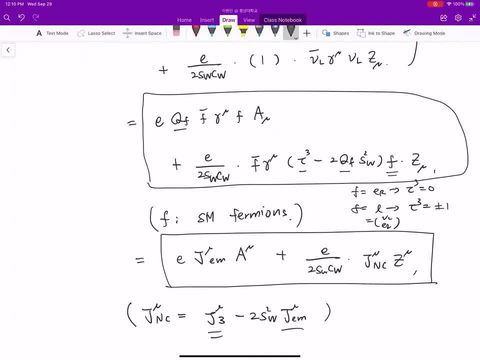 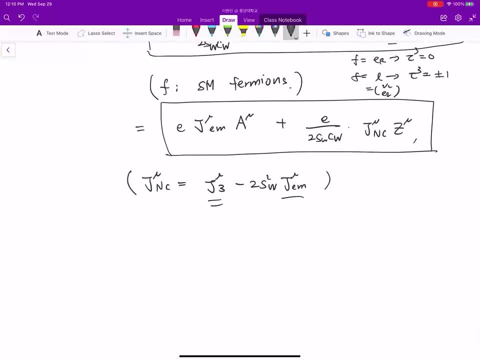 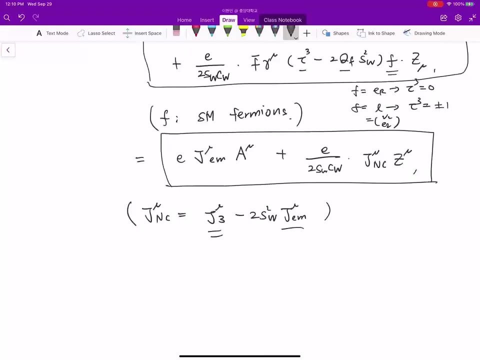 where? what is the value of this? Okay, Okay, So you can see that here this is the mu of tau three and charges, et cetera. But you can find also this neutral current. this form can be written, you know. so just. 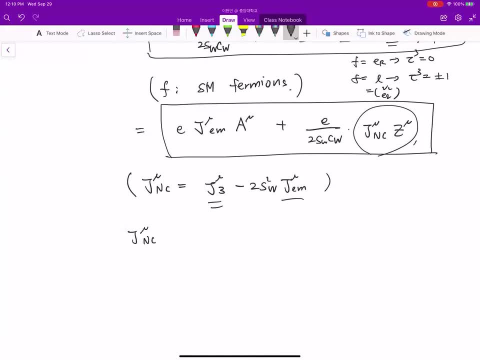 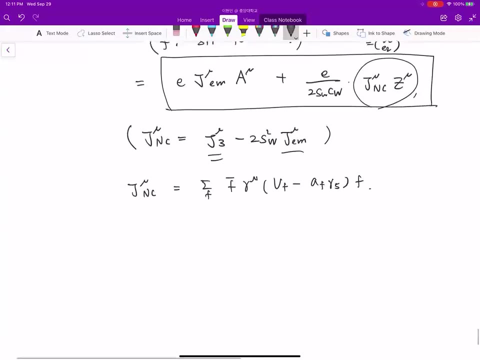 JMU. Sometimes, Okay, Okay, Okay, we are using this notation. so this f, where the this vector vectorial and this is the actual, actual coupling action. and then, in this case, f is the. uh yeah, so deluxe spinner, you can see the tables. so what is the? can take a look. what is that? it's very 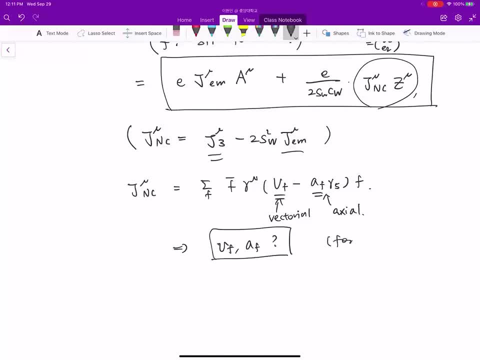 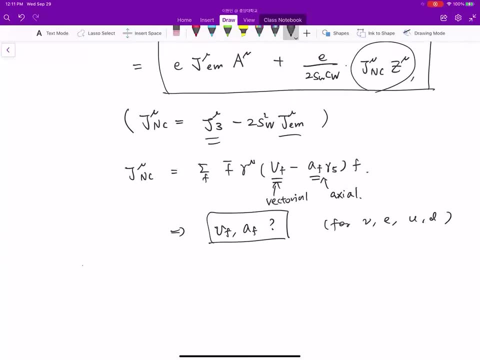 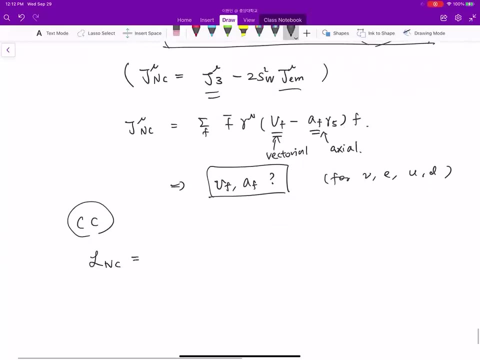 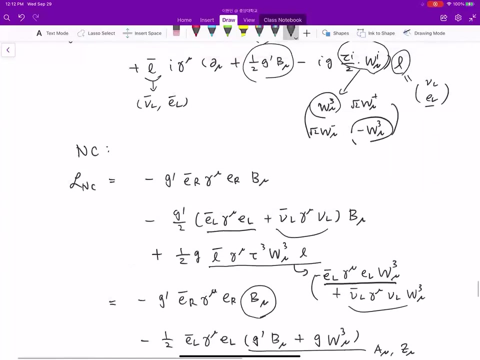 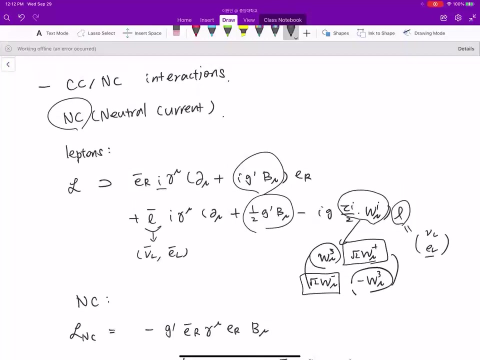 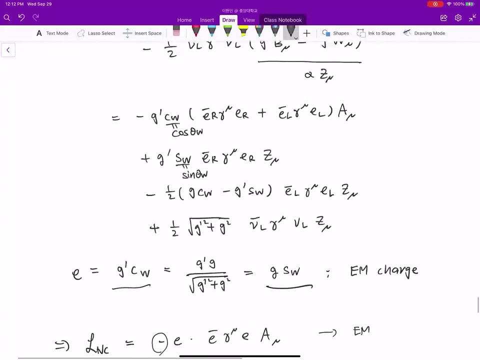 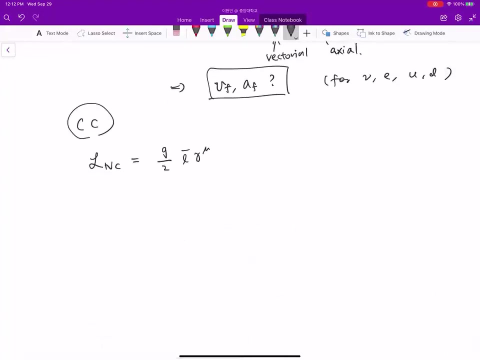 uh, on the terminal electron, you know, down for charged current. uh, uh, it is so simple, the charge current, so let me go back to the this one. so charge it current. here the charge current interaction by the wider value notated: l and c, not lcc. oh okay, sorry. 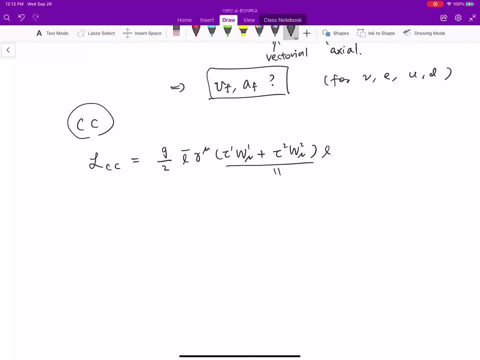 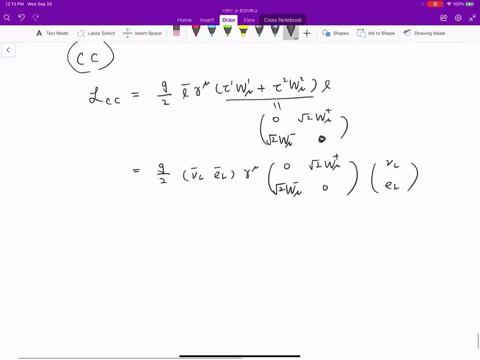 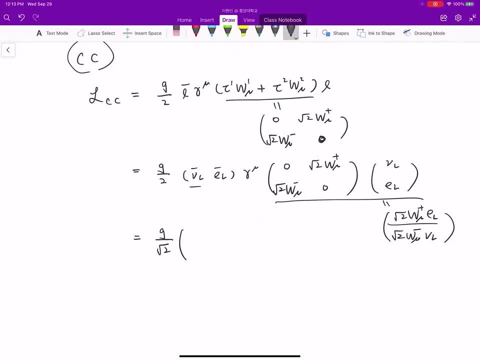 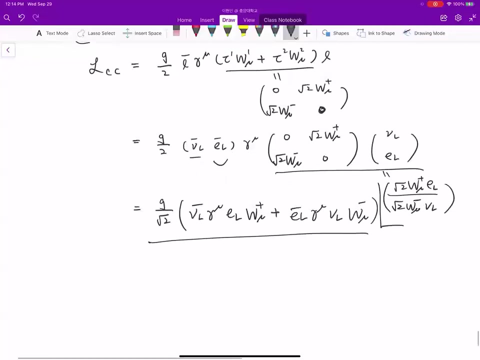 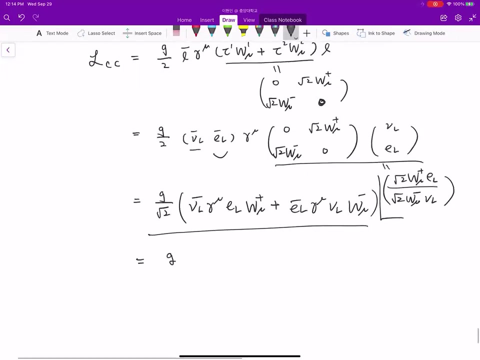 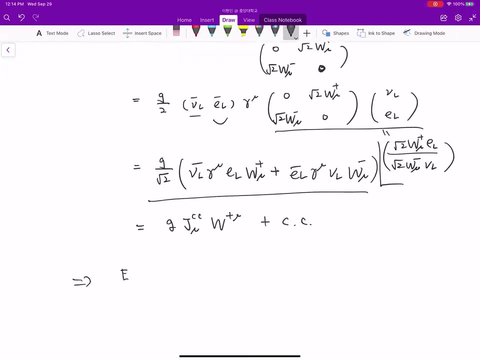 to electron through W-version. The neutrino plus electron couples to neutrino through the W-version. So this charge recurrence we call this, We can think of this also coupling to the current. So because of that I think all the electroweak interactions 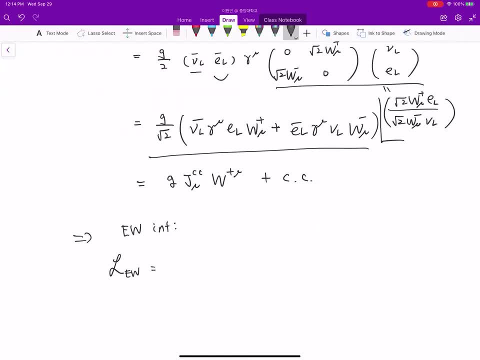 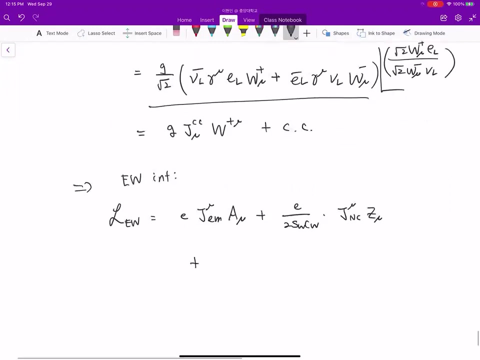 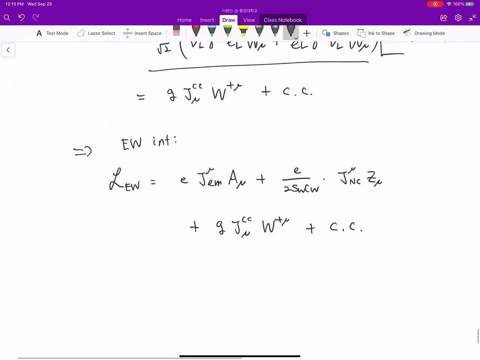 for matter, Or can be written in this simple form. Sorry this one, But I think that this notation is more convenient. Okay, This one, So that's the first one, And then the second one. So this one, So this one. 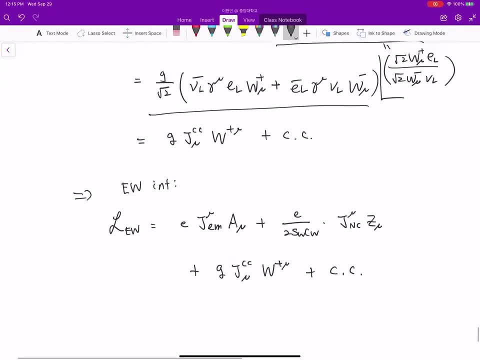 This one, So this one, This one, This one, Okay, This one, And also of course here trial. current contains leptons only, but for quarks. you only have to replace upper or lower entry by quarks. 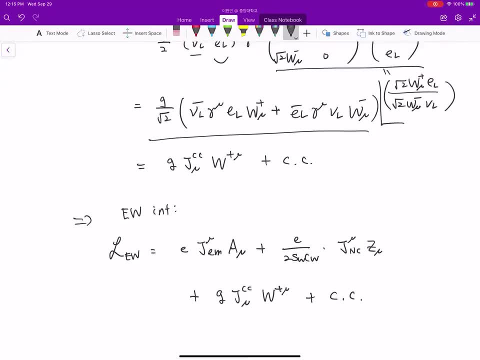 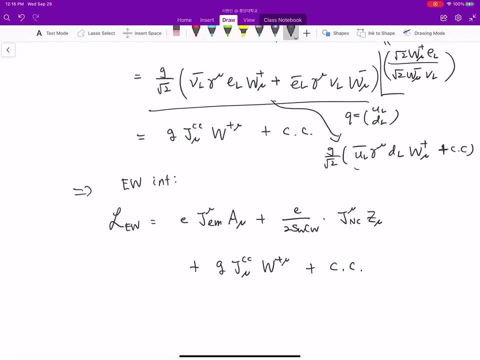 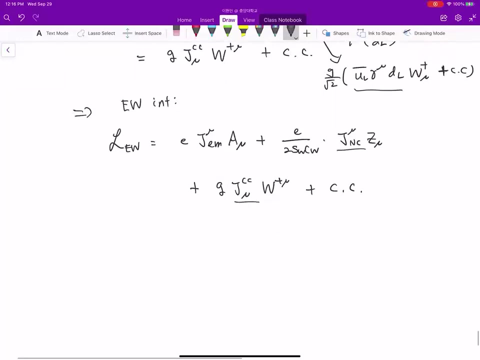 So in the case of quarks, we have a quark doublet, So just this interaction. So neutrino is up, The electron is down, Something like that. That's one way. So this current interaction, this current, in particular, this neutral current and charged current, 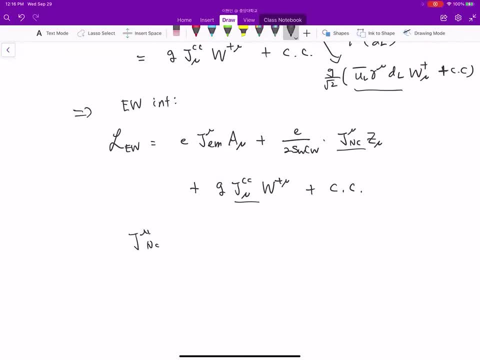 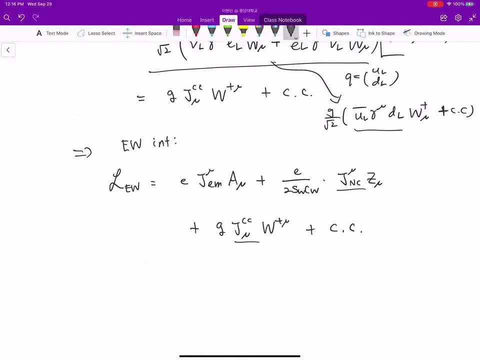 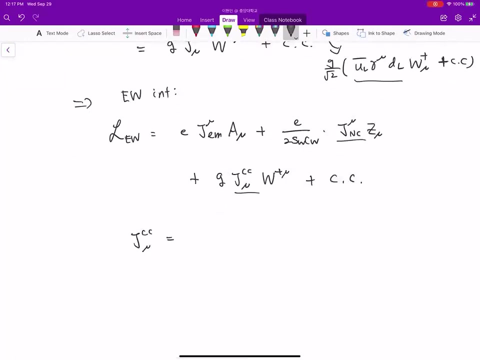 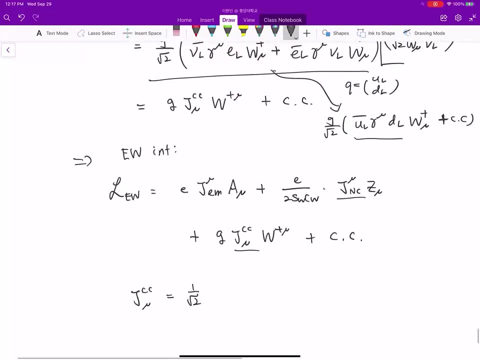 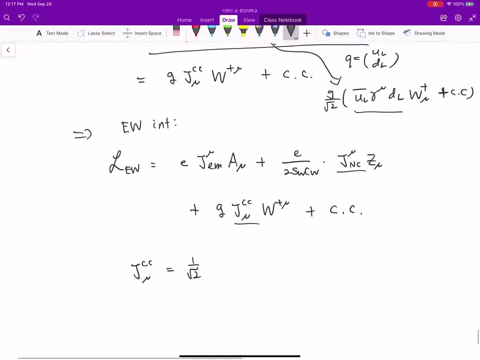 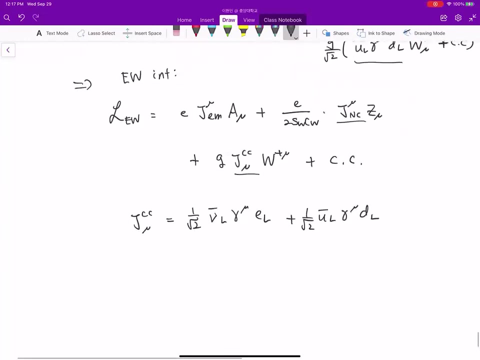 So neutral, current, charged current interaction For charged current. I think this charged current, as you can see, is the, is the, is the neutrino, neutrino, neutrino, which is charged, These two active current interaction, So this. so here there's some projection of right here. 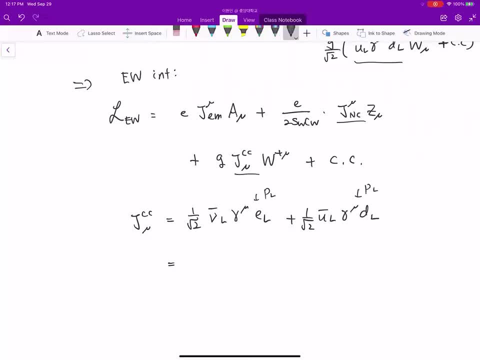 So this is here. So So, because of this, this is the V, the vector and this is A axial vector. so this charging current, as far as the charging current is concerned, V minus A structure is also at the level of quarks. is the V minus A structure. 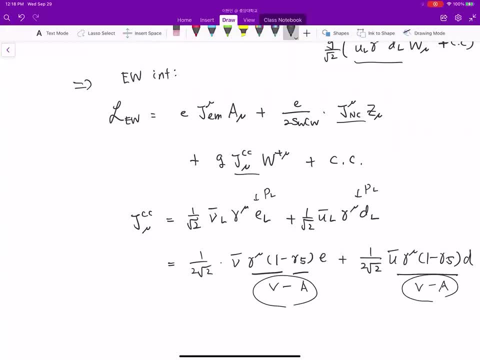 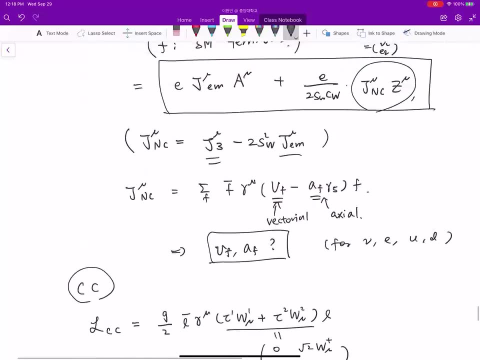 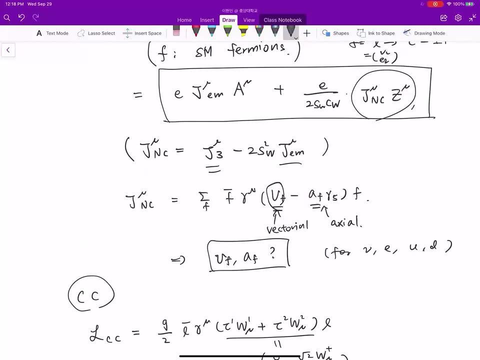 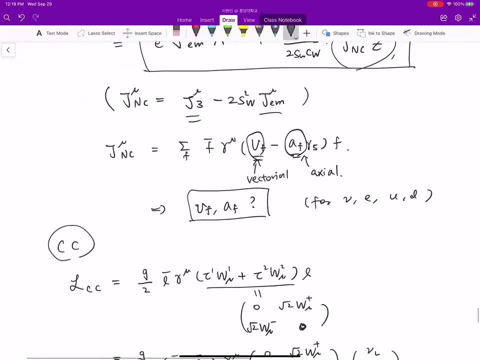 So V minus A structure is very important for the electroweak interaction For neutral current. on the other hand, neutral current, as you can see, this is V minus A, so this is equal. this is V minus A, But we this coefficient. maybe I can tell you, maybe. 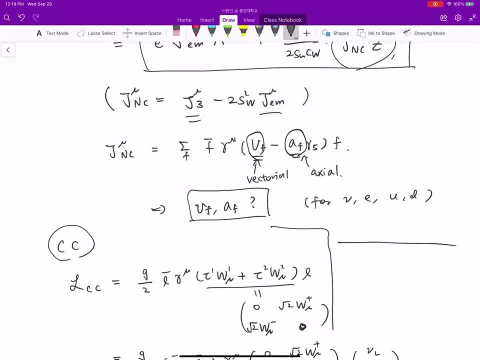 only for neutrinos. okay, So that quark is more complicated Very quick. So neutrino, one half, one half. So in neutral current. So in neutral current, one half, one half In the case of neutrino neutral current, also V-A structure. 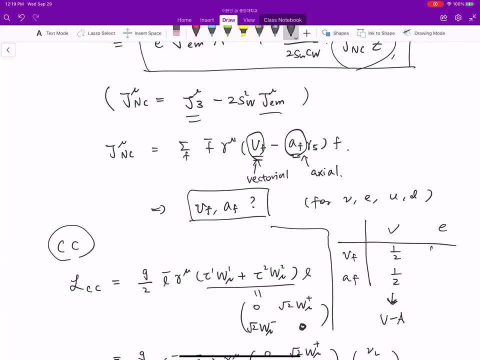 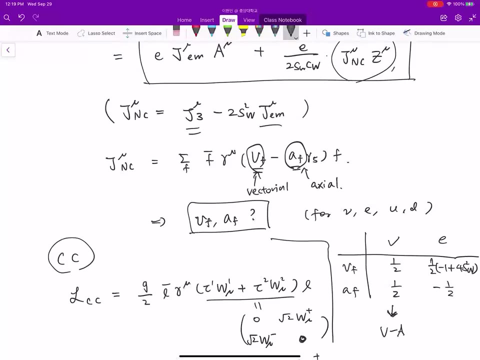 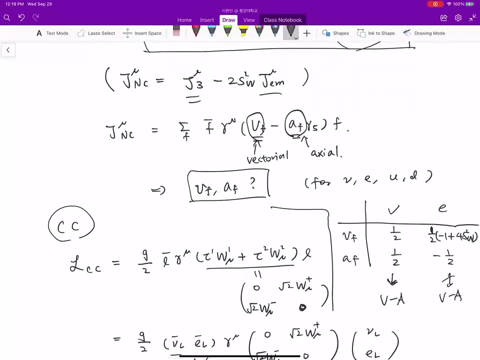 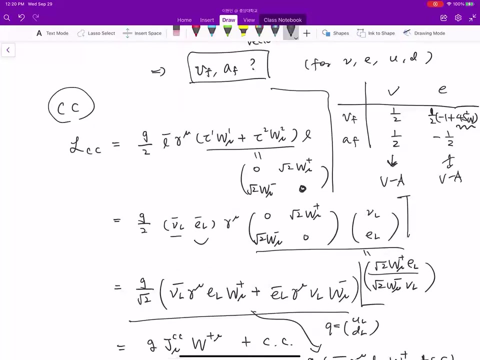 For electron, on the other hand, this is the this one and maybe you can this one, and then, okay, This is almost V-A, but this is not exactly V-A because of this Weinberg angle contribution. This Weinberg angle, as I said, is measurable and it's the Weinberg angle with a W-scale. 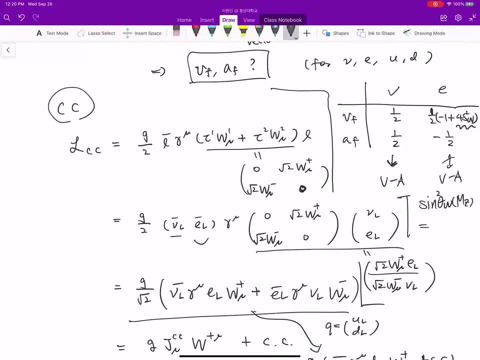 in the deep mass, deep bottom mass scale and it's 0.231.. Okay, So it is a small value, small number, but it is non-zero. So V-A is not precise for electron interaction, but neutrino you can find almost for neutrino. 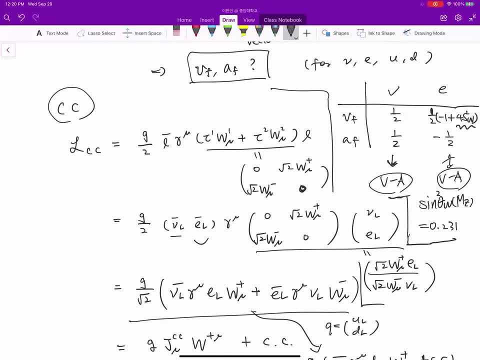 is V-A. So same is true for quarks, The quarks U and D. It's not V-A because of this. So for all the charged particles it is the same is true The neutrinos: it doesn't carry electromagnetic charge. 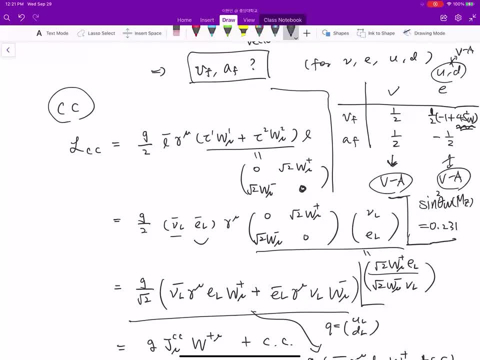 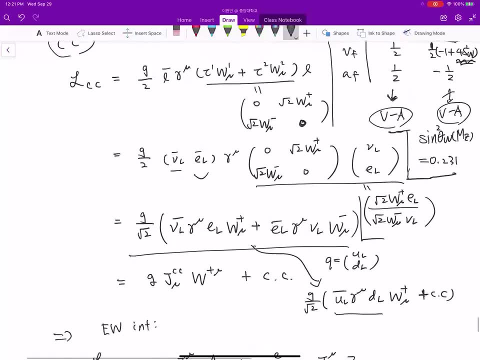 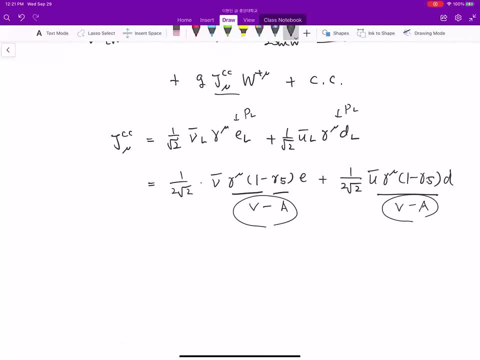 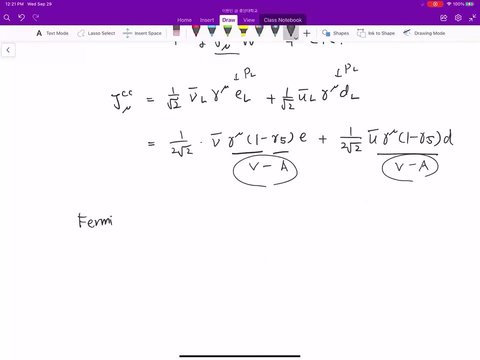 So it couples to G-version only, So it respects the V-A structure, Okay, Okay, So for the. for the rest, munis, and I will talk about the connection to the Fermi interaction, And So in the, in the charge recurrent. 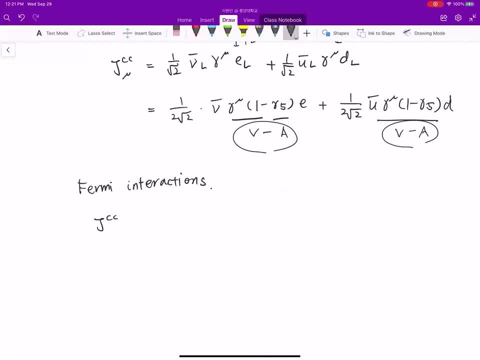 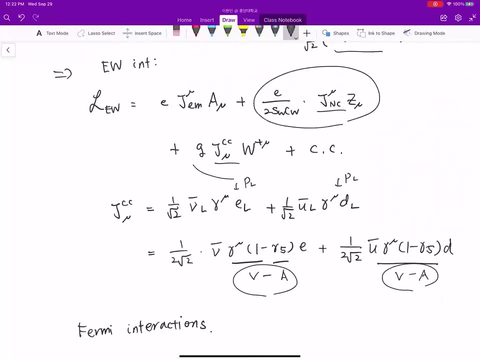 Okay, Okay. Okay. So the Fermi interaction. there are two processes: neutral or charged current interaction. So, in general, where is P, This one, this one? So here this G-version and W-version. they are massive or short range, so we can integrate. 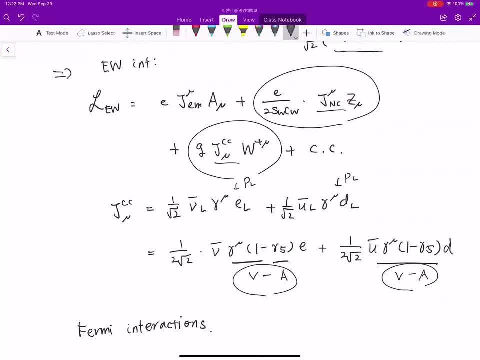 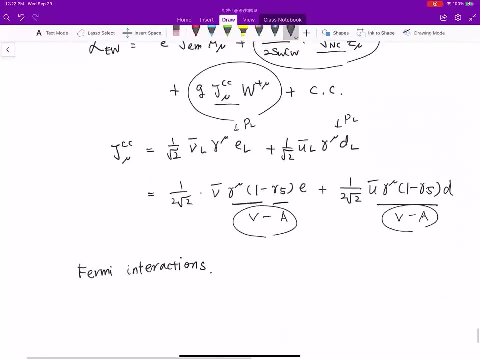 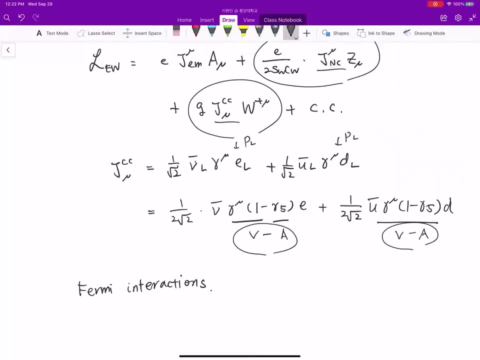 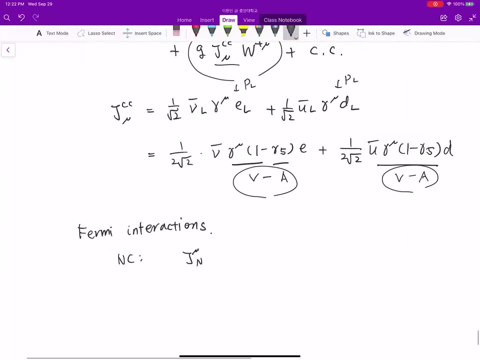 out G-version or the W-version to get effective current interaction. Okay, Okay to get effective interaction for quarks or leptons. So maybe there are several ways to see how to get the effective interaction. The Fermi interactions for the neutral current J mu. neutral current J. neutral current mu. 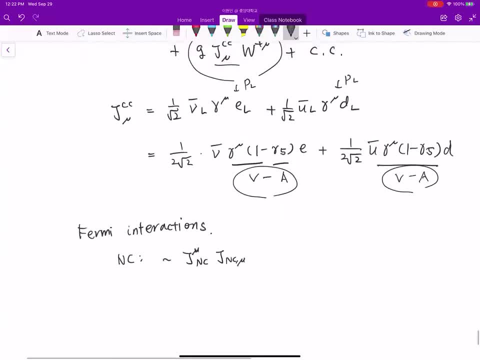 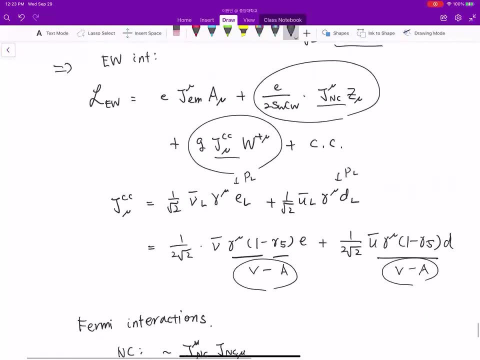 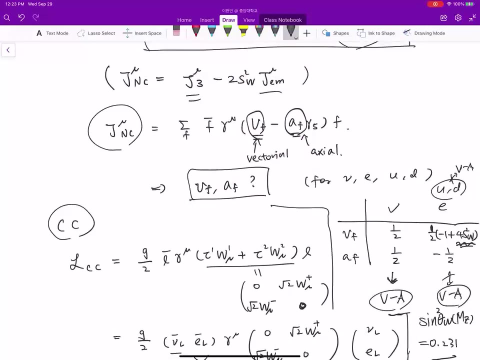 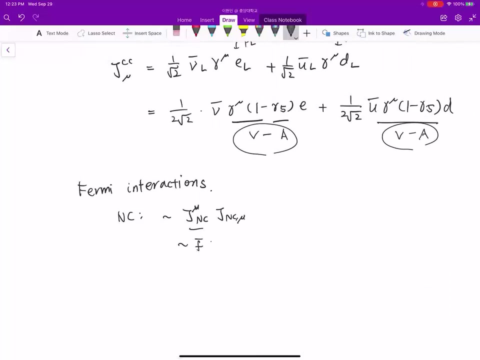 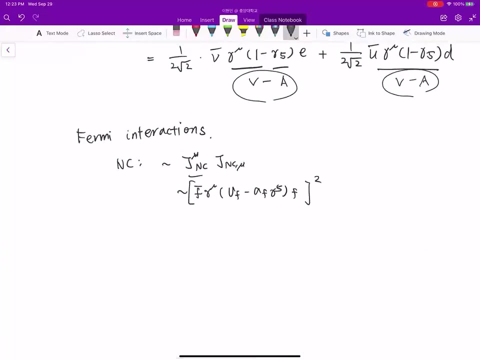 So these are the four Fermi interactions. So neutral current in the case of velocity, neutral current, this velocity. so this is the neutral current right. Neutral current is the F, mu, VF, A, F, just like that, And this is just the scale. So neutral current induced effective interaction. 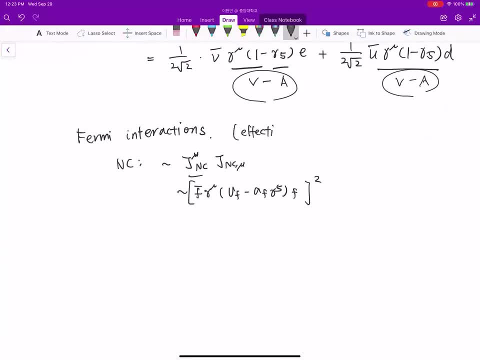 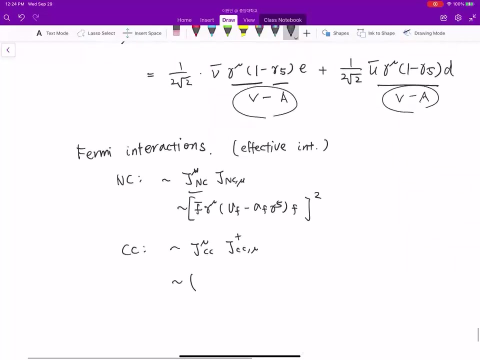 So this is the effective interaction F? uh, if you don't see WG version directly: Charge current interaction is the this one? So this, uh, the charge current. where is the charge current here? So, uh, what is the fine? fine for the J mu Cc for the left one. 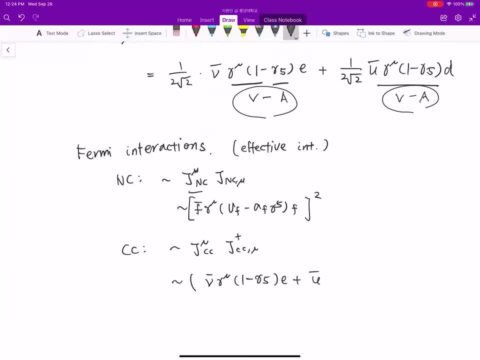 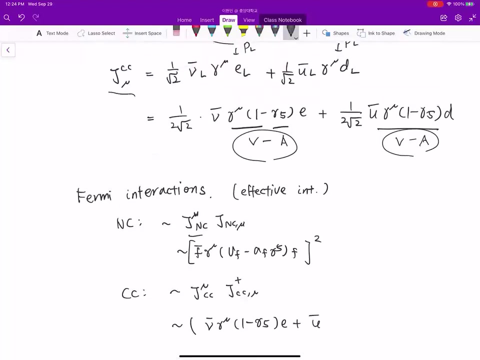 Sorry, I meant, uh, for Cc, one J contains plus, but the other J does not contain any. fine, I was. I am wondering if that minus or plus, Which one, I don't know. This one, The most bottom one, I mean. 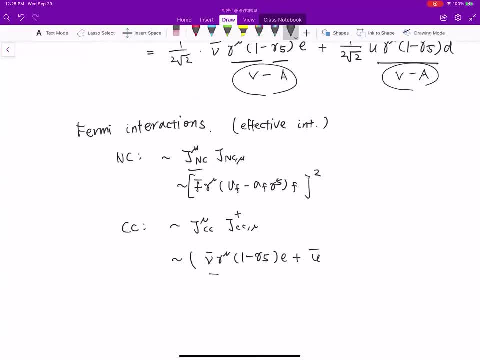 This one, Yeah, The upper side of that. This one, Yeah, The left one, looks like there is no charge Charge. I'm sorry, I I thought the plus. This is conjugate, Conjugate. Okay, This is the. 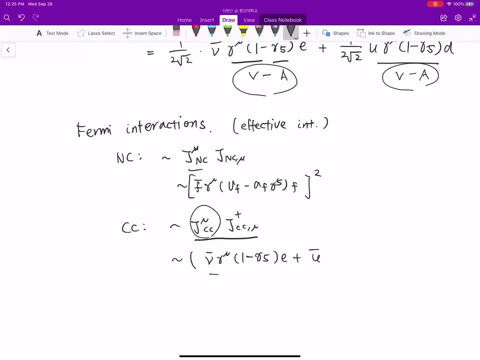 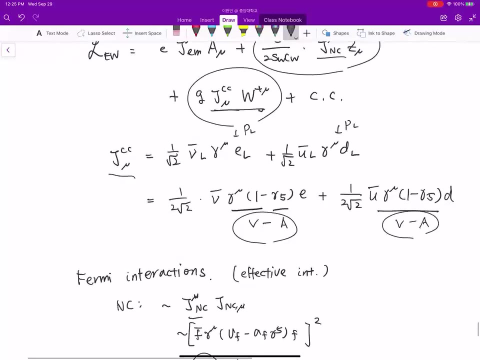 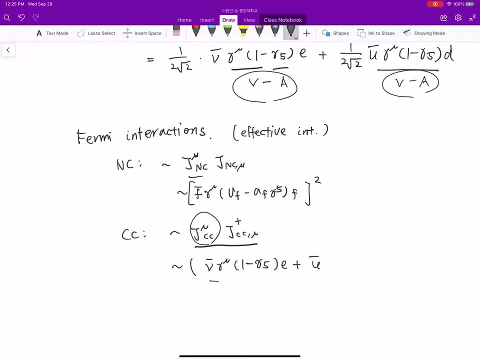 the charging current has a carry certain charge Right Because it couples to W version And a combination of this combination must be neutral, charging neutral. So I think the the charging current to charge it Current target current is complex because of so. 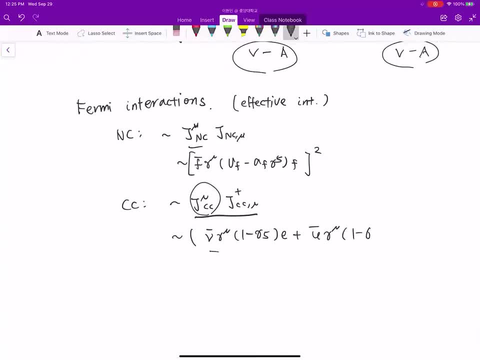 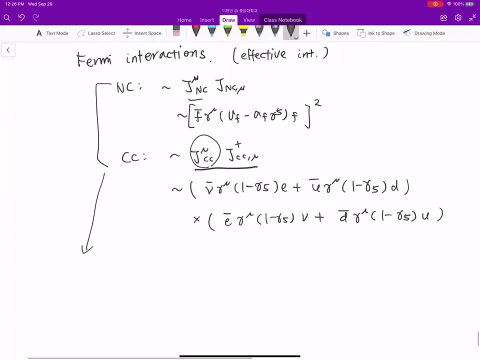 uh. okay, So in both cases, this uh uh uh, this, this is Um uh uh, this, this uh, this, this uh uh, this is uh, probably, this is. 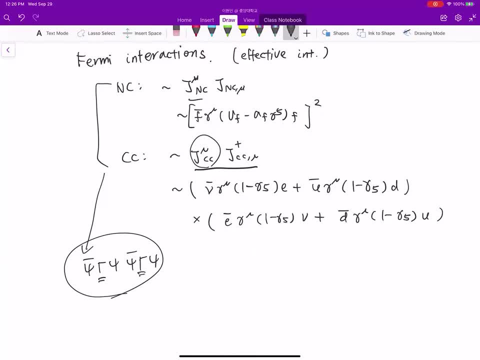 uh, a little bit more complicated. So here, uh, uh, this is the, this is, of course, this is the one. Yeah, I um uh, leptons, or between quarks, or between lepton and quarks. 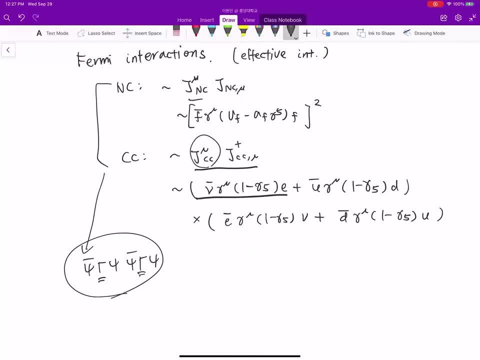 so, so this is the lepton current and this is the hadronic current. but the hadronic current actually, uh, we have to. we are measuring the hadronic current at the hadron level, not in the quark level, so in the low energy, this will be replaced by the hadronic current. 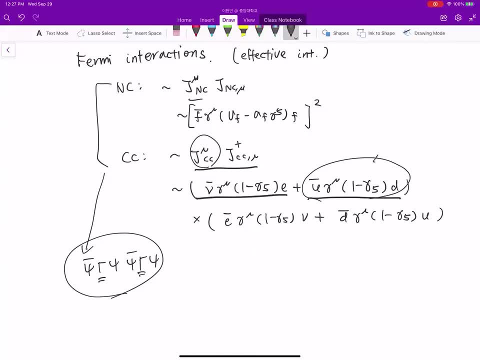 in terms of proton and neutron. so this is the hadron, but the, yeah, just below the electroweak scale. uh, we can describe them in terms of the quarks and leptons. if you go to like a proton scale, then you need to use a proton scale. 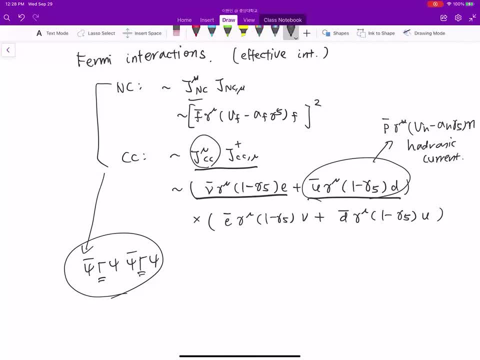 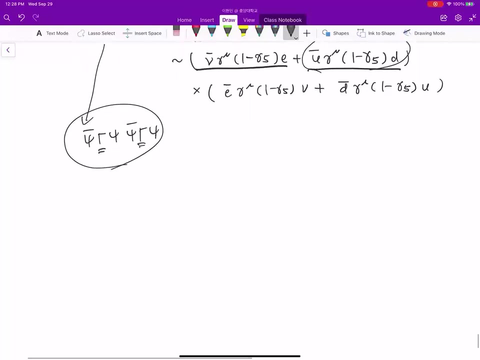 consider proton and neutron instead of quarks. That's the only way to So. this is the effective interaction. this is the neutral current and the charged current, And we can easily identify the coefficients of the charged current and neutral current For muon decay. 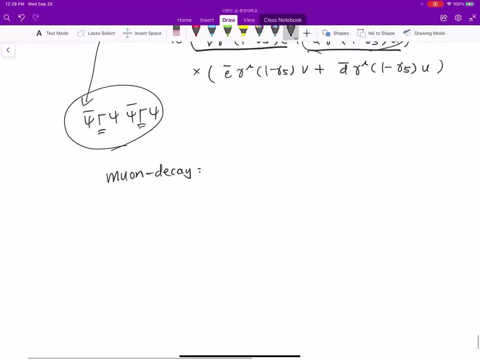 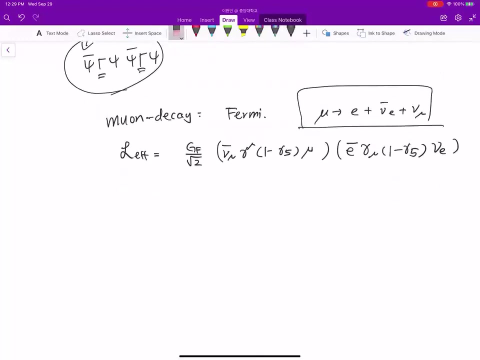 or beta decay. the Fermi introduced effective interaction with the G-Fermi constant. So here muon decay, muon goes to electron plus the electron neutrino. So from this effective interaction you can describe the muon decay In terms of this point interaction. 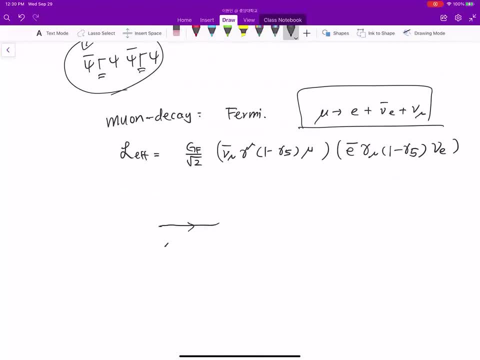 So this point interaction, muon, So muon annulate to create neutrino, muon, neutrino, But these are all at the same point, occurring at the same point in spacetime, Right. So point interaction, So electron, So anti-electron. 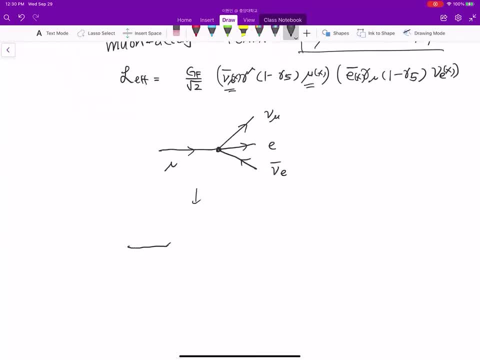 But we know that this can be expanded in this form by including the charged gauge version. So at the level of amplitude you can the decay amplitude mu to E. So this decay amplitude by using the Feynman rule for the charged current. 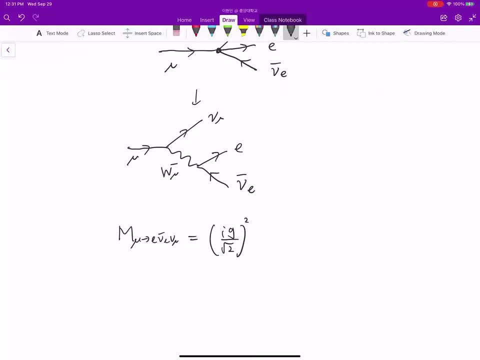 so we have a charged current interaction. So from the Feynman rule we can easily identify the momentum Q square and the force that it will carry. So this W boson carries certain momentum Q square. so by adding this W boson, 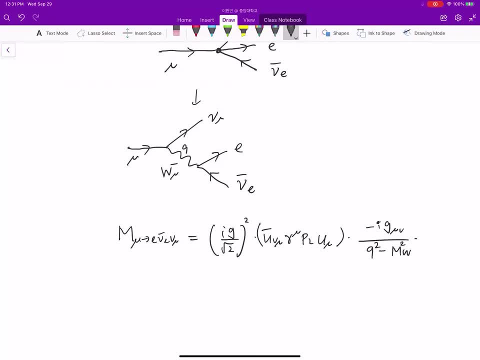 we can determine the momentum Q square. So this one, because today's lecture we have only students from our group, so just I can tell you directly the amplitude, otherwise I cannot tell. So here the momentum of W-Boson is much smaller than W-Boson mass. then you can even out this. 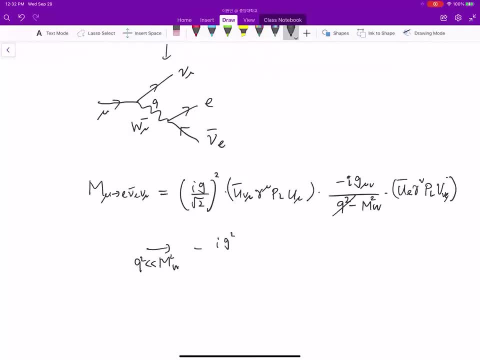 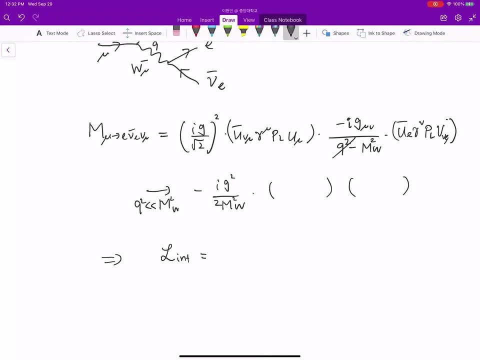 momentum in the W-Boson propagator And you have a 4-formular attraction And this decay amplitude can be written as so this from the Feynman rule. you see, Feynman rule for decay amplitude is just from the interaction times, I so from that I see some. 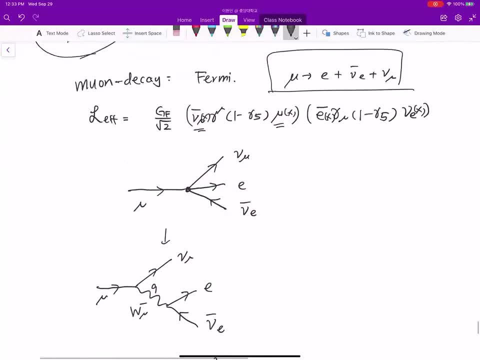 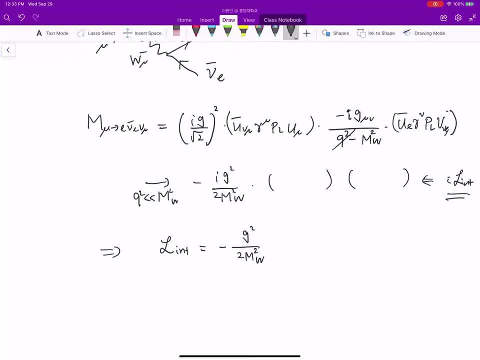 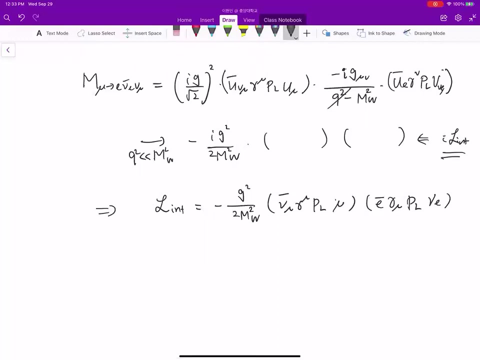 sign difference, so the standard notation. I think that this one was a minus sign here. so there's a minus sign, so this one, in fact, by interaction you can identify from the amplitude and then this becomes minus g for me. 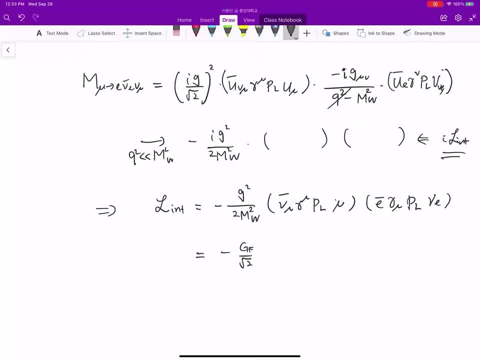 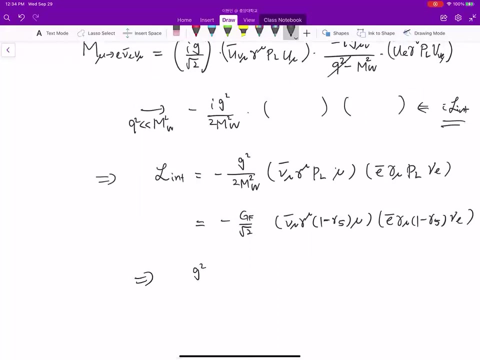 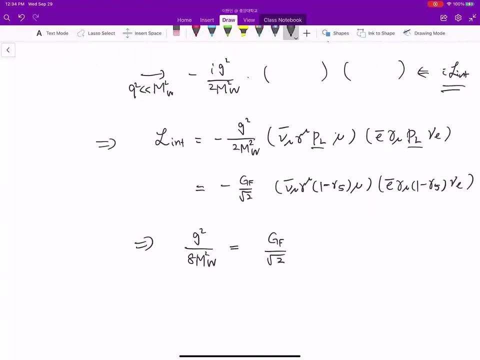 In g for me in the original form written in this V-A structure. so instead of projection operator. So from there you can easily identify. so we have a one-half factor here from the projection operator. So g for me effective interaction to describe the muon decay or the better decay can be. 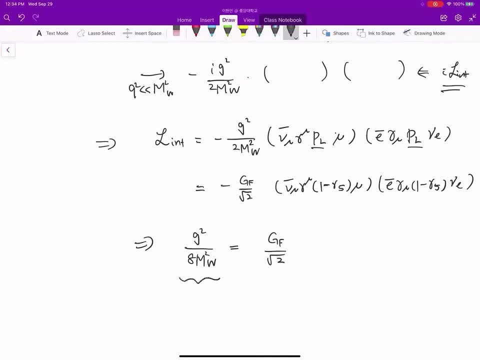 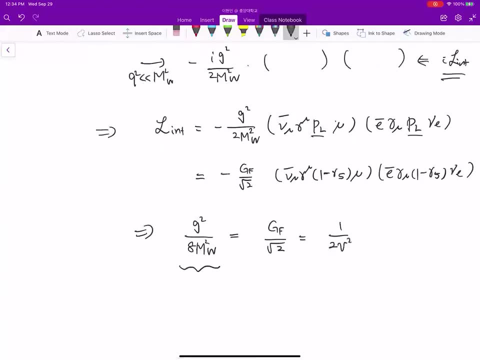 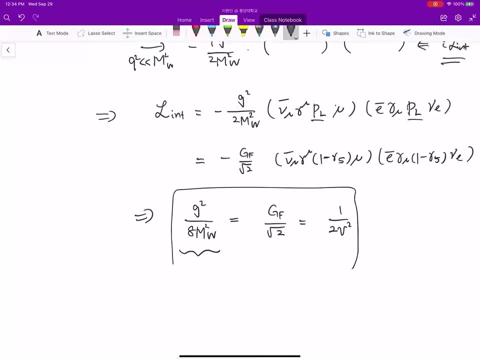 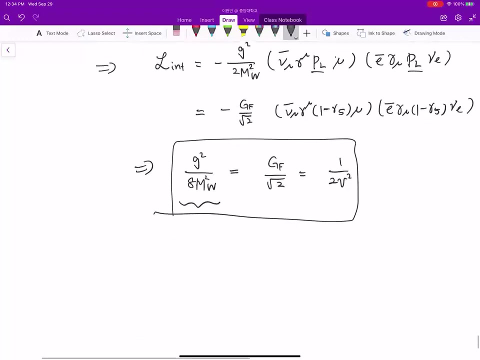 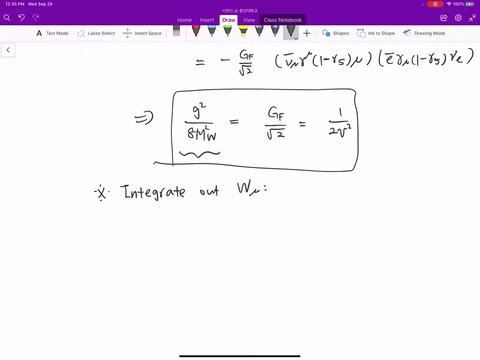 identified with the fundamental parameters in this theory, and the g for me is also equal to electroweak scale g for me. So, Yes, If we have a big say in the equation, Yes, Okay, Great, Thank you. 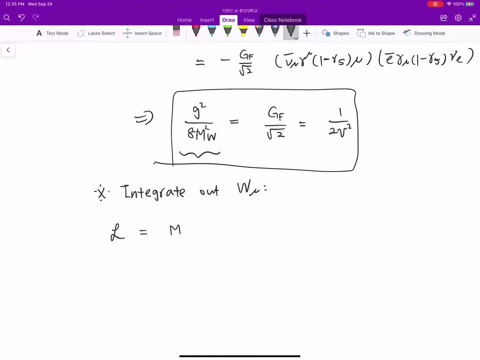 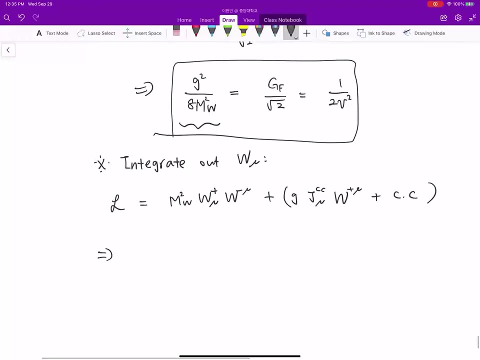 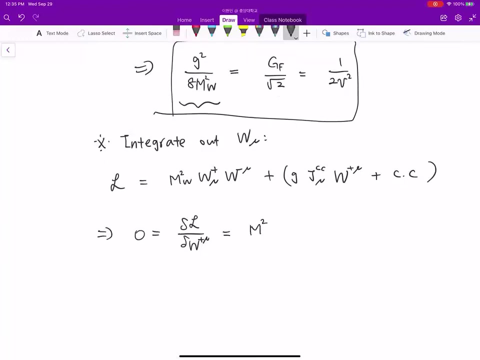 Thank you, W version mass written down here and the charge current and the complex conjugation From there. integrating out means you consider the equation motion for W version without kinetic term and you will get some equation motion for W version. So just you vary the Lagrangian with respect to. 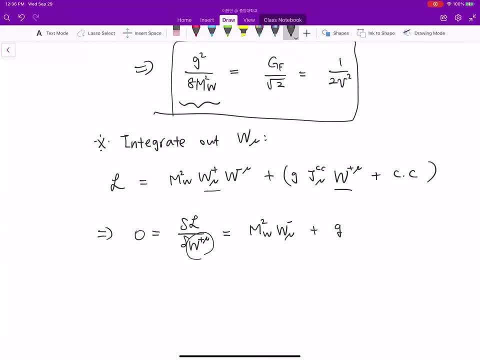 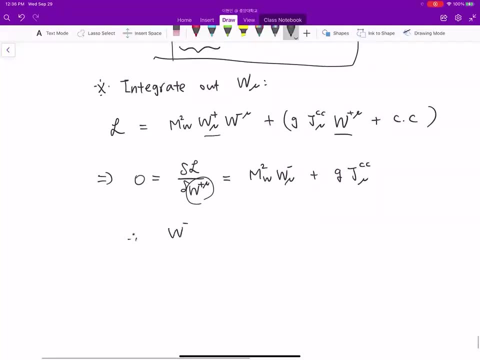 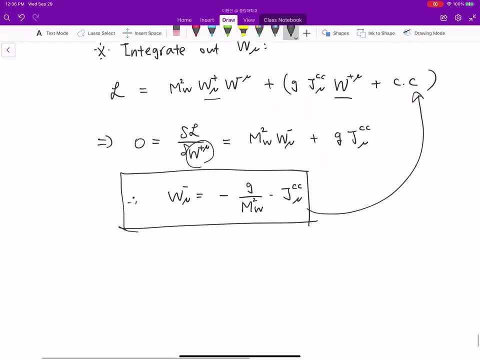 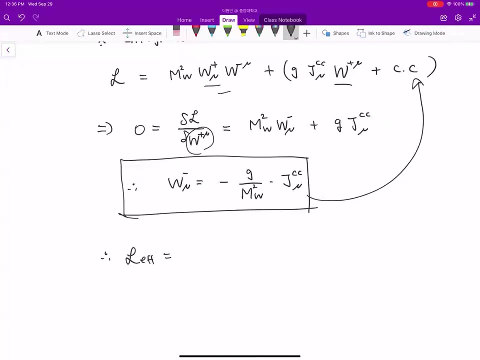 the positive charge. So you can solve this equation for W version and put it back to the original Lagrangian. Then we the effective Lagrangian you obtain, So W version. here we have a square W version, J, J, mu. Then there are same terms with the negative sign. 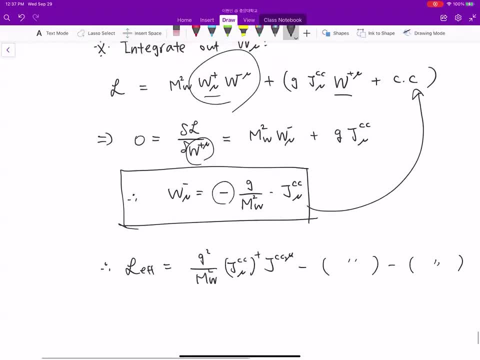 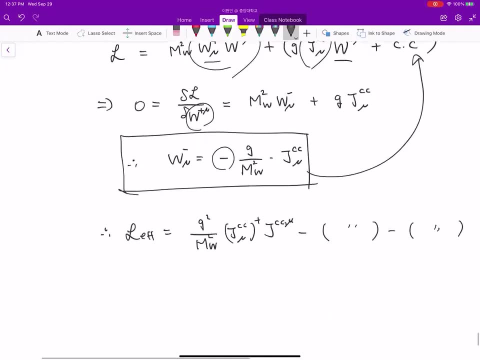 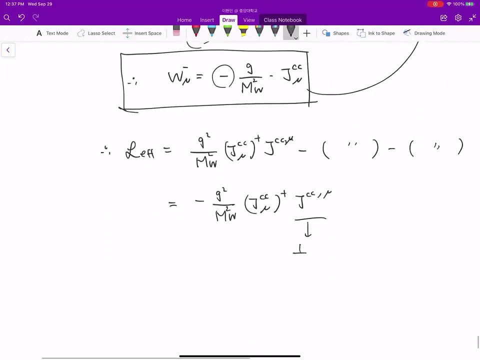 So, because of this minus sign here, when you put it back this second and third term, you have a minus negative contribution. So you end up with this, Okay. so then there's the charged current, There's the contains square root of something. 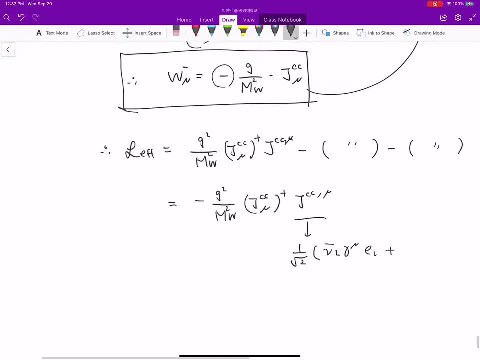 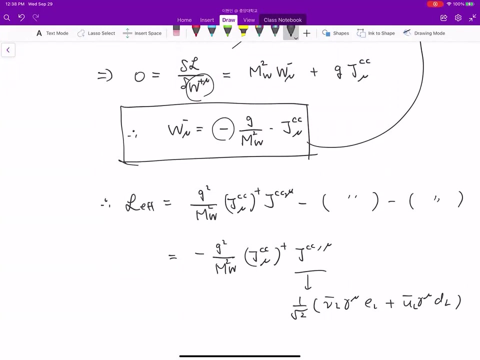 So then there's the charged current, there's the contains, square root of something, And then you write this, Then you will get exactly the same interaction, Lagrangian, as we derived from the diagram Feynman diagram, decay amplitude. So this is the way to obtain the effective Lagrangian, or effective Hamiltonian. 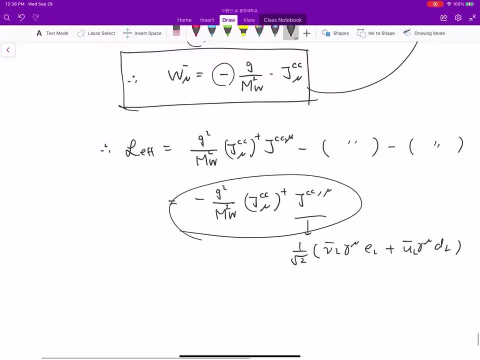 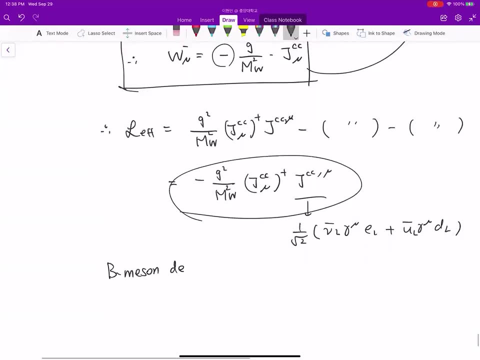 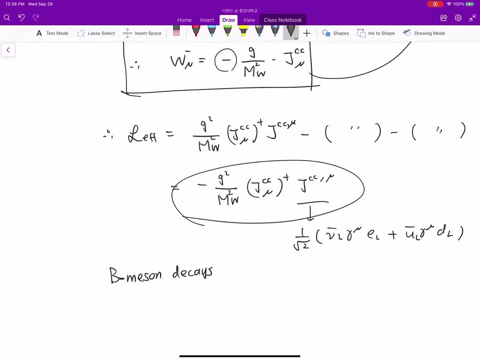 And I think, the B major decay, for instance. recently people have discussed the B major decays Also. we are using this kind of trick And also new physics: When the new particle mediator, particle is very heavy, you integrate it in and out. 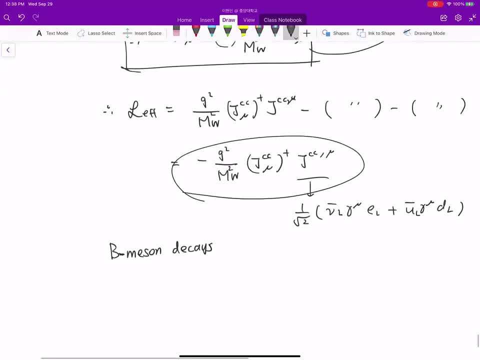 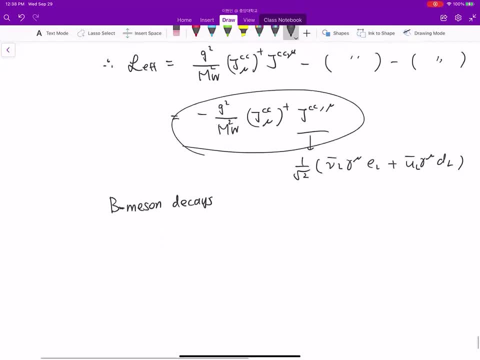 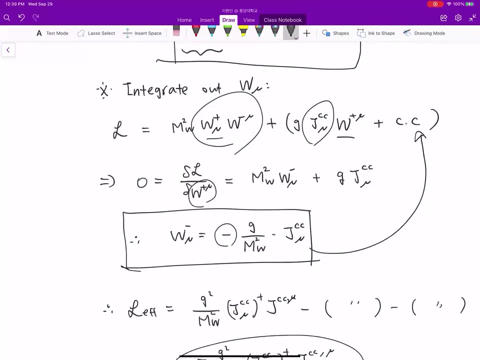 Ok, so so next to next week we are going to discuss: Do you have any question, People? integrating out means the piece are four message before. they are non-block ā, almost not fluctuate. Is that right? Yes, You're right, yes. 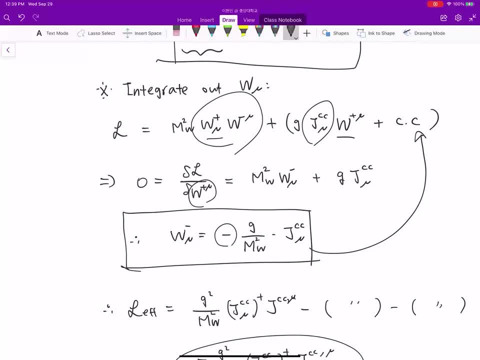 So here almost W, because we are ignoring the kinetic term. so W is the kind of non-dynamic quality of freedom. So you can think of auxiliary field and if you have some field auxiliary field in the Lagrangian, you can use the equation motion for that and you can we call it. 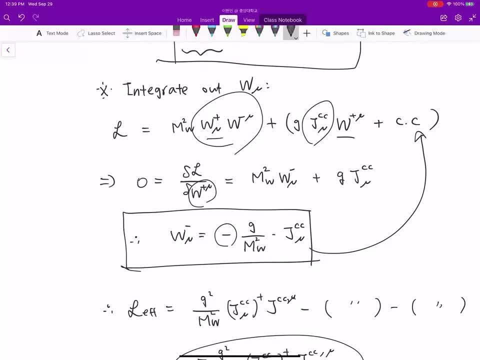 integrate, integrate out at the classical, at the classical level. So I think the Adriana Jisun are familiar with this integrating out procedure in the four-form paper. In the case of four-form flux models, anti-symmetric tensor build is non-dynamic, non-dynamical. 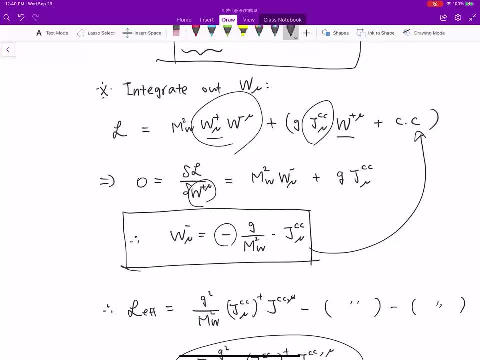 so we integrated out to get the effective interaction. So the same is true here. And if you have a kinetic term, then if you, if you want to include that kinetic term, you know if you don't want to include it in the perfection you want to integrate out. 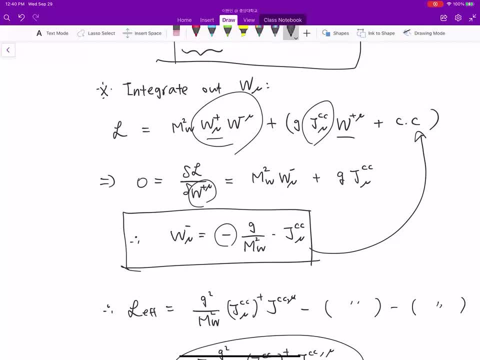 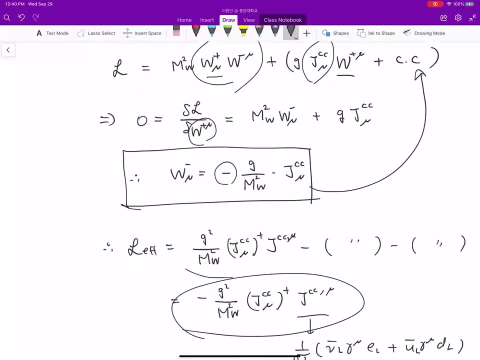 the kinetic term for w version, then I think the maybe you can treat the kinetic term for w version as perturbation. so then in the, in the effective interaction here with this charged current only you don't have derivative term or only field, but if you include some, the 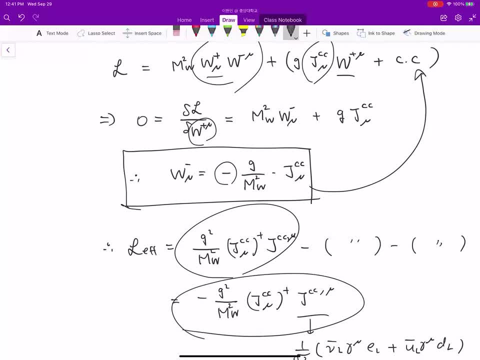 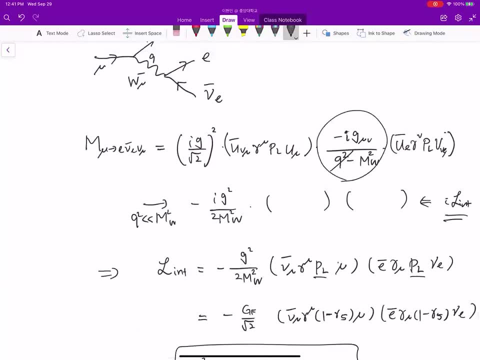 kinetic term for w version. then you have non-zero derivatives. so I think the also in at the level of this amplitude. you can expand this one over q square m, w. this vector can be expanded in this form and just here we are keeping the leading term in this derivative expansion. 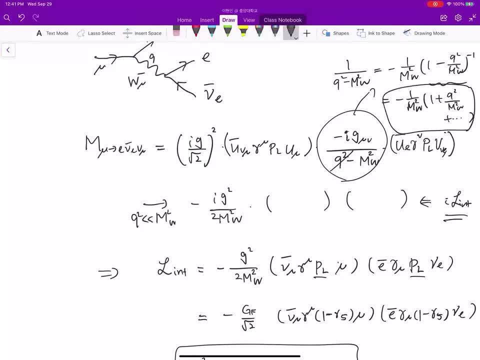 right. so we took only leading term in order to identify the firm interaction. but here we have a high order momentum dependent term. so that is, that corresponds to including the kinetic term for w version for w version at the at the level, at the level of lagrangian. 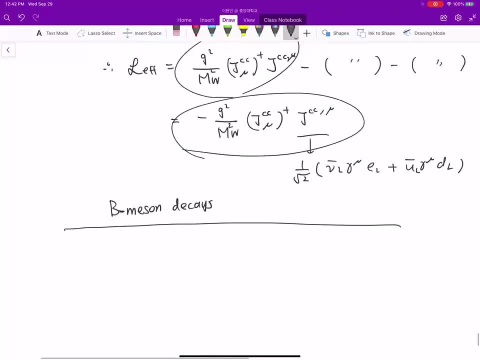 okay, so, so this is a very well-known procedure. yes, so next next week, if you know, if you learn the history in mode detail- I mean history on particle physics, I mean in standard model- is very, very interesting, and the way to construct the detailed structure is also interesting. you didn't know it from the 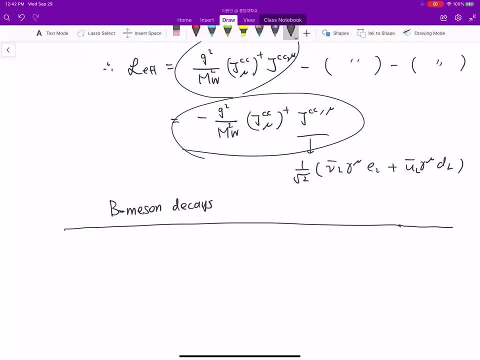 beginning and. but they wanted to explain some experimental data and they figure out some distance of new particle. so I think this is how this behavior works. so I think this is a very good model and I wanted to give you a few remarks about mu and in the sequence that you just saw right now, but there's interesting things that you have to do to find out where the 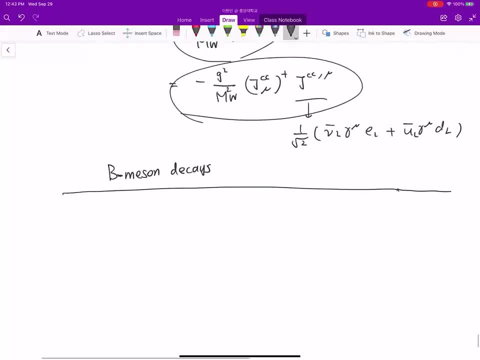 so i think the interesting is interesting, uh, i think the uh. for instance, when people didn't know about the existence of strange core, or charm call, the people knew that this structure from the muon decay. and we know that, uh, up and down core, those exist from proton or neutron. so neutron, proton, the neutron decay. 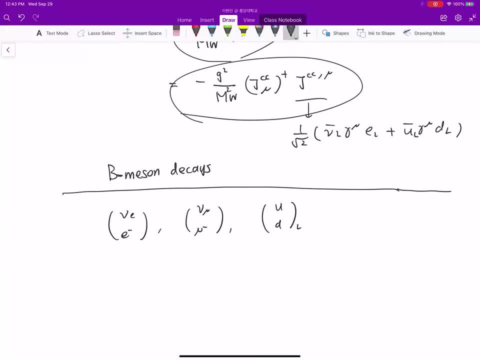 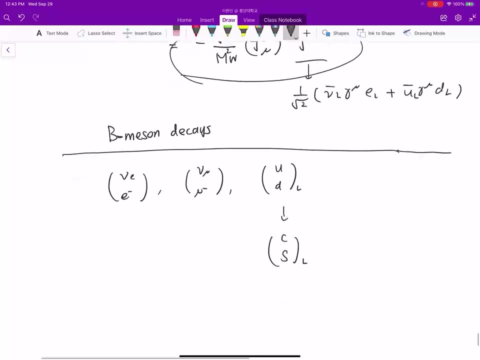 for instance, beta decays can be described by electroweak interactions. then here we are: have to add additional quarks. at the time we didn't know about tau, but there is a important implication for the existence of extra quark, doubling so, which was due to the decay mode. 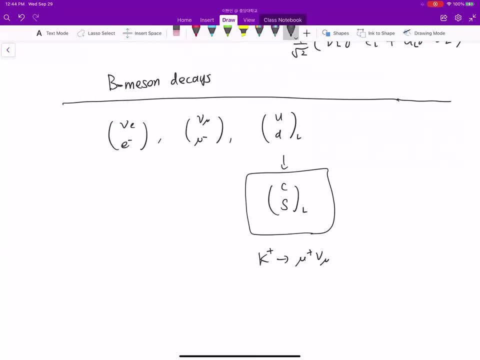 of kaon. so we need the extra generation and also we need one more generation for quarks. so in this case, top and bottom because we need extra generation for quarks. so in this case, top and bottom because of cp violation. so if you don't have extra generation, 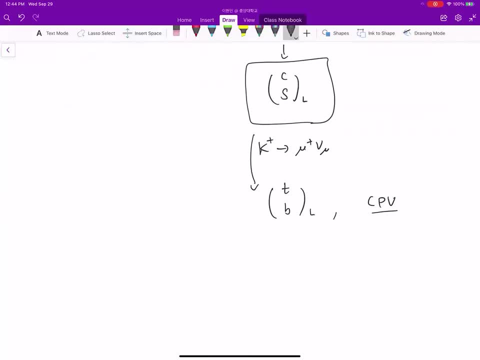 you don't have cp violation. so this is only true when you have three generation oops and also, uh, i think that that this is the the first the k on decay. so we uh have to introduce copy by angle. so flavor mixing is very important in the history of particle physics. 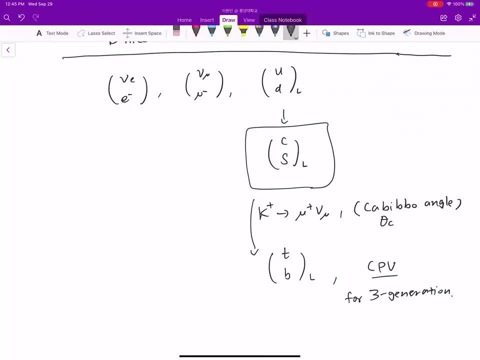 and also the gim mechanism was the pre. i mean the. the copy of angle has to do with the mixed in between, uh, down and strange. so these are mixing between down and strange and the existence of charm quark, of course, due to the su2 structure, but this one is also predicted from the kaon. 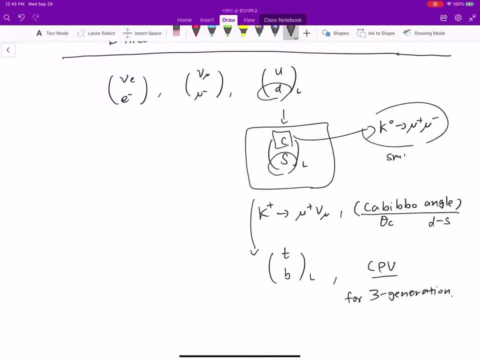 decay, the smallness of decay of neutral kaon. this decay rate is very small. uh, so at the time people thought that is unnatural and that has to do with the existence of charm core, predict existence of charm core and and it is called the gim mechanism, to cancel the leading contribution by introducing additional particle charm core. 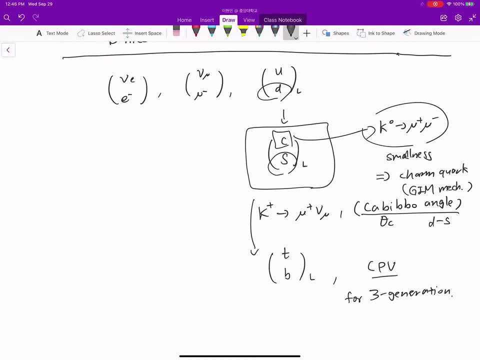 so it's like it's similar to the hierarchy problem. so if you have a large correction to the higgs mass due to top core and you are have extra contribution from support particle stop and then these two contribute to the same quantity to make the higgs mass, uh, small. so this is the i think a very similar situation and i think the many 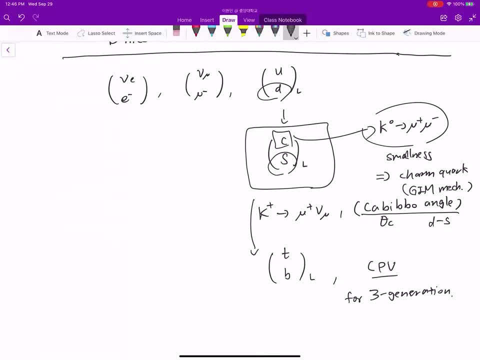 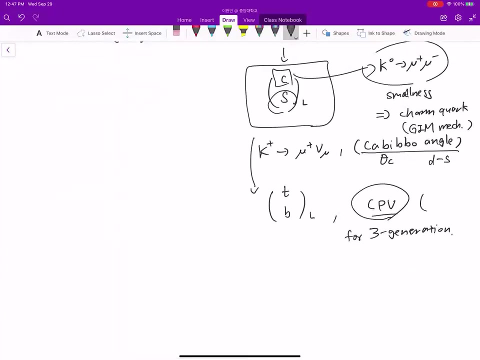 problems with giant gm mechanism and intensity vibration. so next to next week we are going to CKMF has to do with the CKM matrix and just to, I think the Khabibov sees Khabibov, Kobayashi and Maskawa. So Kobayashi and Maskawa, they awarded a Nobel Prize in. 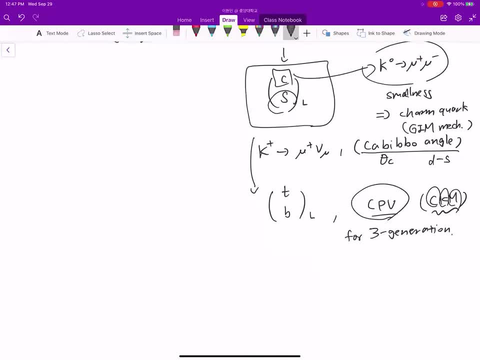 2008 and together with the Nambu. but Khabibov passed away before the Nobel Prize, so just Kobayashi Maskawa. I don't know if Khabibov is still active, but maybe the Nobel Committee did meet with Khabibov before the Nobel Prize. 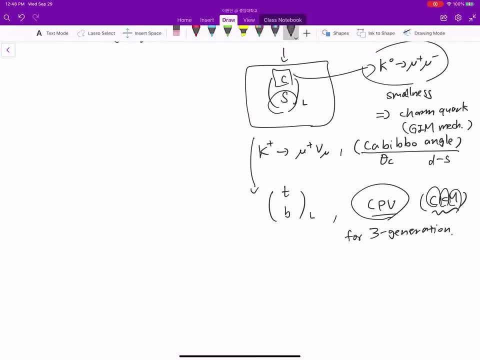 I don't, I probably. yeah, probably Khabibov still active, but maybe Nobel Committee did meet with Khabibov before the Nobel Prize, missed Khabibov at that time and replaced him by Nambu, but there was a, I don't know. 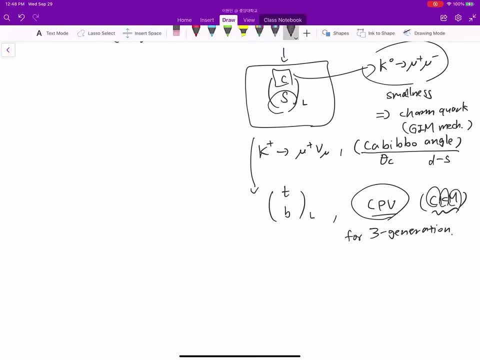 sometimes people missed Nobel Prize. they passed away immediately because they were. they are waiting for the Nobel Prize for a long time and they, if they are not awarded Nobel Prize, they are frustrated, disappointed and passed away. in that case- And also I think there's some interesting for the other guys, the other two students- 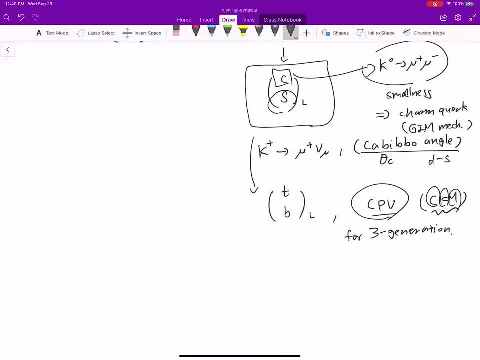 neutrino scattering is also interesting in the low energy processes And for us for dark matter study, neutrino scattering is very similar to dark matter scattering, Except that neutrino neutrinos are almost massless. but so we have to think about similar. 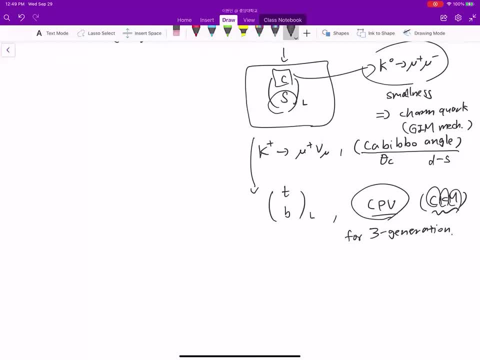 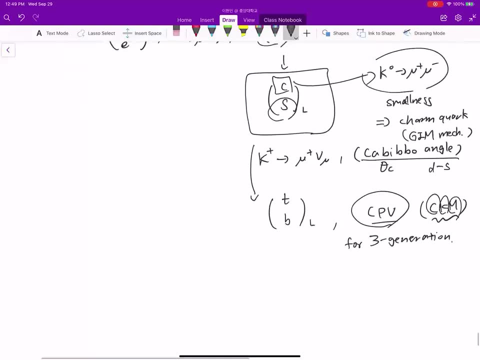 processes, also for dark matter detection. so neutrino scattering will be also discussed after this, GIM mechanism et cetera. so neutrino And also- this is a very, I think, a hot topic in recent years- neutrino, electron. 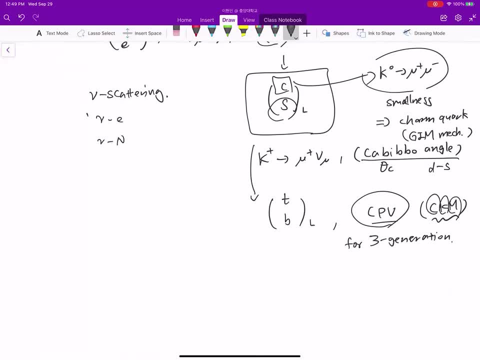 And also this is a very, I think, a hot topic in recent years: neutrino electron, Great question. Okay, cool, Nice thanks. Okay, I richly appreciate you joining us today. I really appreciate saying thank you and yeah, so, yeah, I really appreciate everyone. 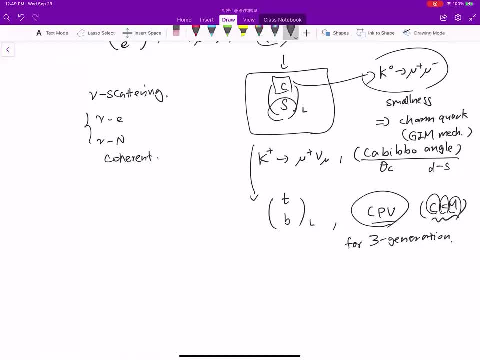 for coming to see me. As such, I really like your services And I'll see you in the next session. All right, thanks everyone, Good bye, Thanks, Okay, bye, Bye. It is composed of many nucleons. The nucleons move as if it is heat. 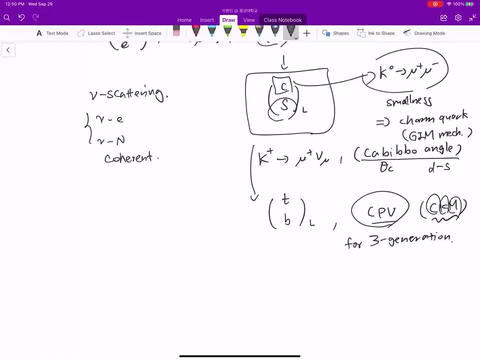 I mean the current is moving and nucleons are scattering. with the nucleons It's the origin of scattering, but the nucleons move at once, So these are coherent scattering, So also similar phenomena. But for document, we haven't, we haven't found any evidence for coherent scattering. 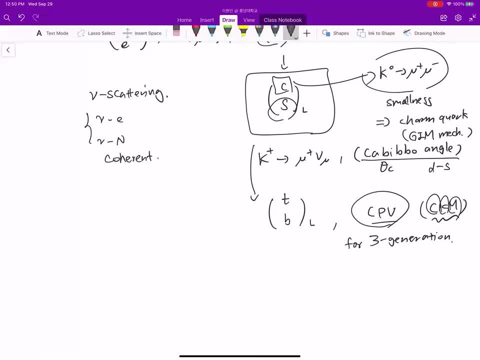 But in the Trino case there was evidence of coherent scattering in recent years. So it will be interesting. And then maybe the experimental data has been improved a lot. But I have to update. I have a note in 2014.. I have to see what are the current update on the experimental data.